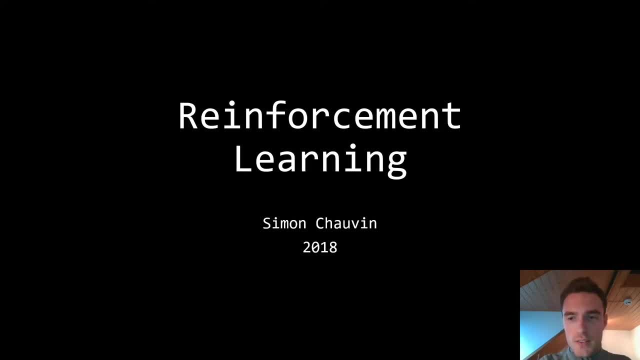 The second objective I have is to show you that actually reinforcement learning holds quite a lot of intuition about human behavior. So I will do some parallels and to show you that RL concepts can actually be transferred to your everyday life scenarios. That's the goals. Probably not so much cover in the other YouTube video, so I hope you will enjoy it. Before I forget, all the sources and references of the pictures I'm using can be found in the description. 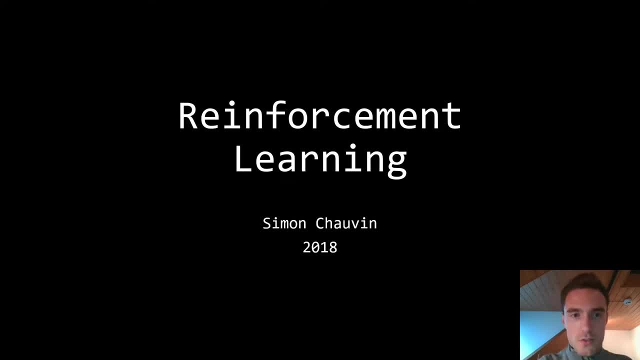 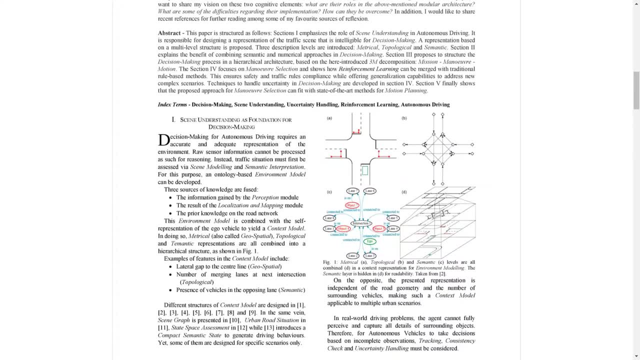 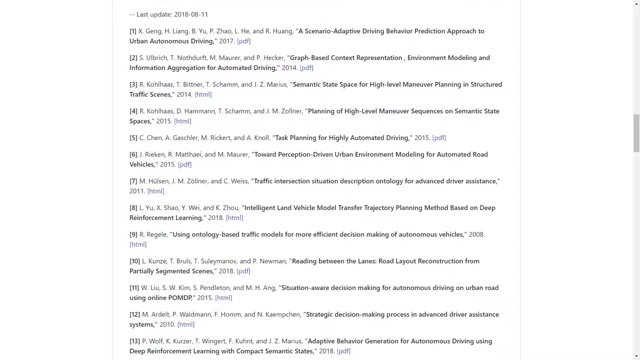 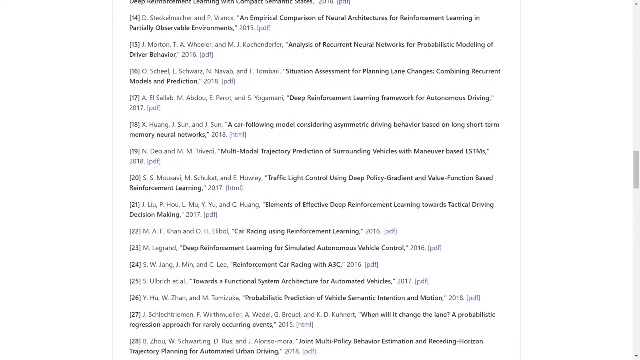 In this presentation, I will be mentioning some research trends about decision making and reinforcement learning applied to autonomous driving, and I have recently published an informal paper on these topics, So feel free to have a look. It is available on ResearchGate and on my GitHub as well. It comes with a very long list of references- more than 90 total- So just have a look if you are interested in these topics. 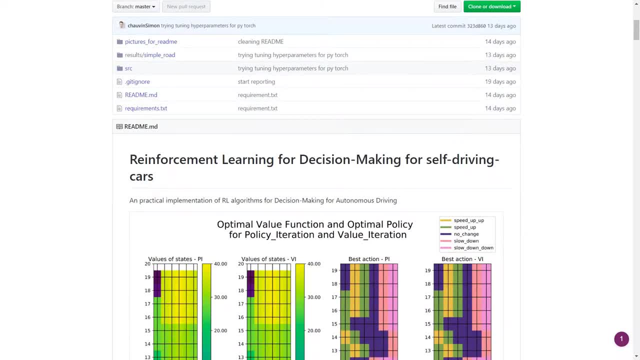 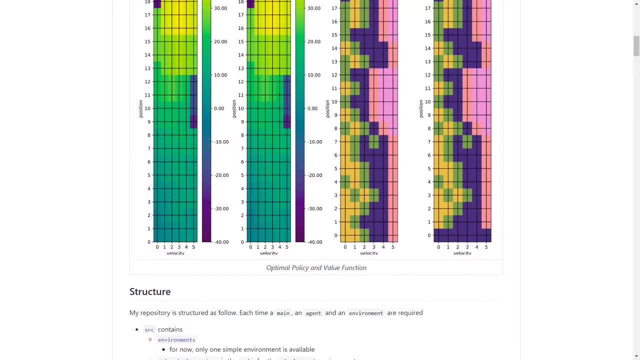 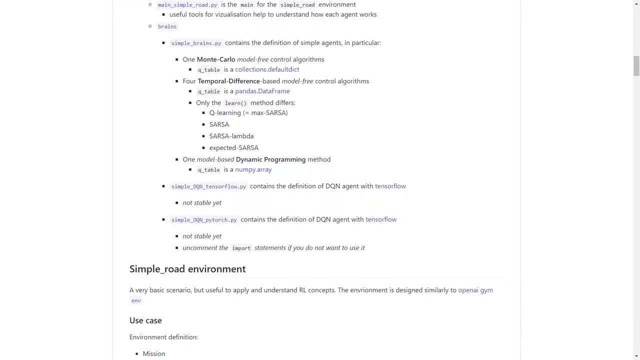 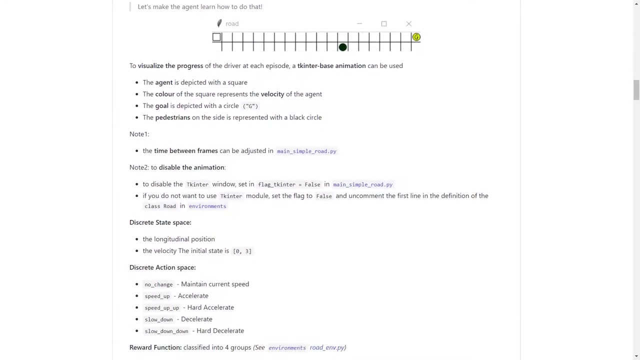 And finally, let just me mention that you can find the code of the example I'm using in this presentation. It's also available on my GitHub and it comes with the implementation not only of model-free algorithms such as Monte Carlo control, Q-learning, expected, SAR-SAR and SAR-SAR Lambda, but also for model-based planning, with dynamic programming policy, evaluation policy, iteration, value iteration and, in addition, you will find the definition of RL. 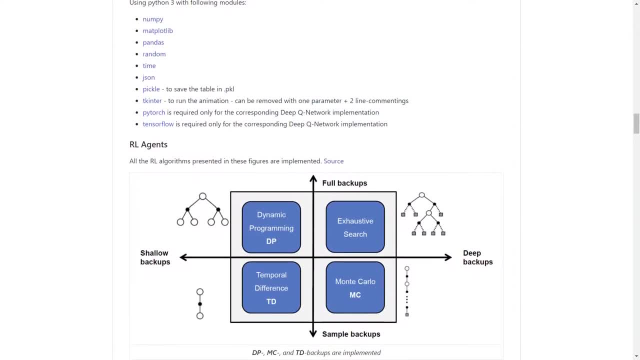 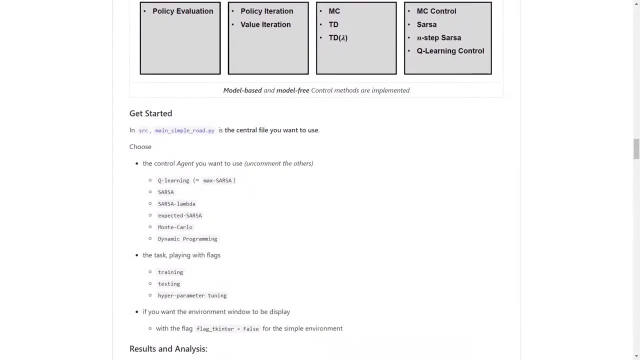 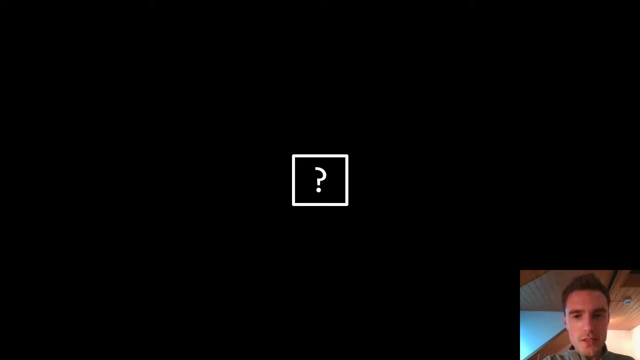 All the links in the description, And I really want this session to be interactive or at least dynamic, So there will be some time for a quiz. Stay attentive: As soon as you see this symbol, you know that there will be a question coming. 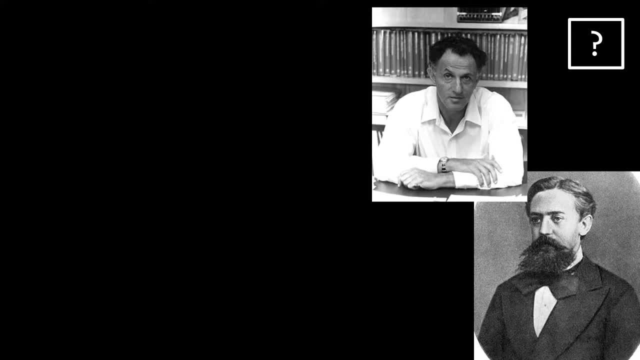 Alright, first question: Who are these two mathematicians? The first one comes from the US Senate- Okay Comment is Richard Bellman. If you don't remember about the second one, it's probably because of the memoryless property he has developed. He is the Russian mathematician Andriy Markov. 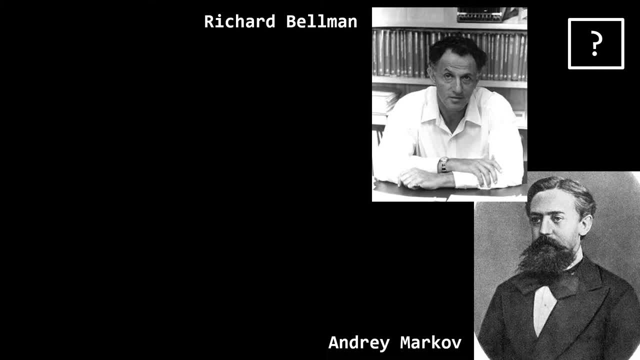 They will be joining us today and they are responsible for all the equations we will be seeing. So we will need some maths to set the problem with the Markov decision process, and then we will use the Bellman equation in the framework of reinforcement learning to solve this problem. At the end, I really want to keep some time speaking about the perspectives. 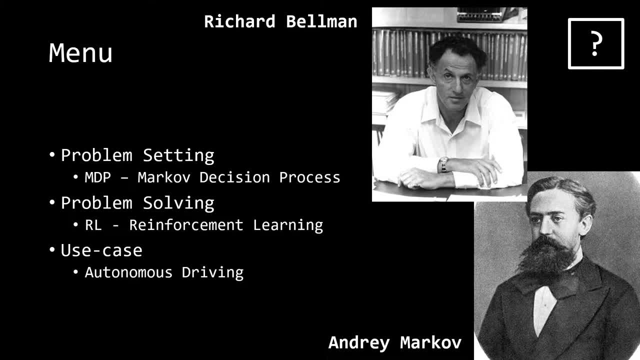 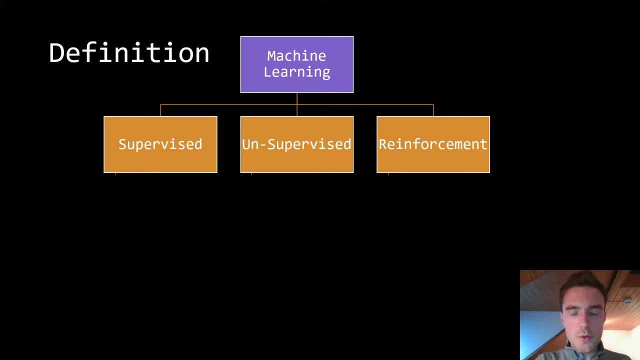 of reinforcement learning, especially in autonomous driving. But before that, let's start with concrete examples and applications to give some definition and have some intuitions about reinforcement learning. Let's start with machine learning. You probably heard, I've heard of it. This is the science of getting computer acts without being explicitly programmed. 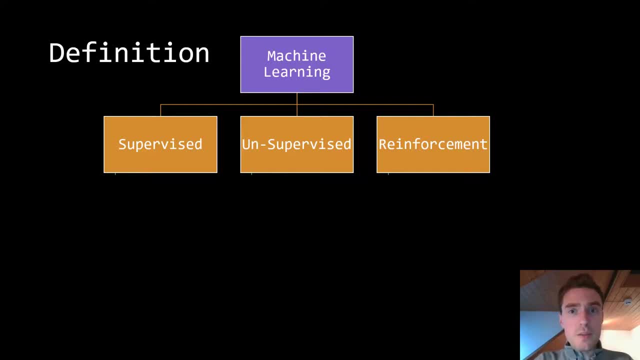 In other words, these algorithms have performance that improve over time as they are exposed to more and more data, And it can be divided into three classes. This is a simplification, but three classes, let's say supervised learning, unsupervised learning and reinforcement learning. 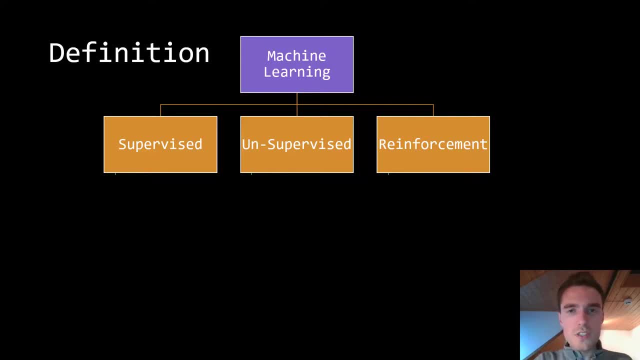 You may ask. OK, now the question is how to distinguish. I'll give you a method. Which of the three is applied? Well, I find it convenient to ask two questions. The first one is about the data set you are using when training. So training is when you are developing a model, improving your model. 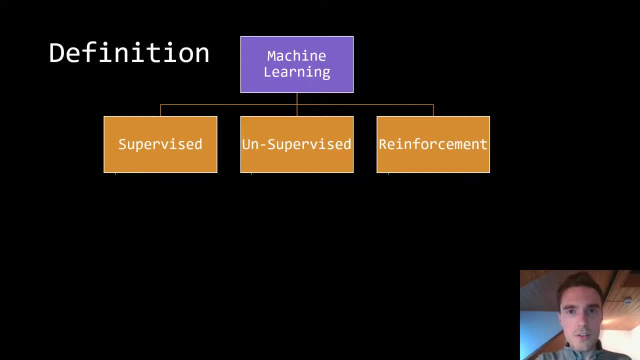 but it is not testing, This is not in production, This is still in development. So the data set, where does the data you are using come from? Is it from a static data set- In this case, the first two can apply- Or is it from an environment? 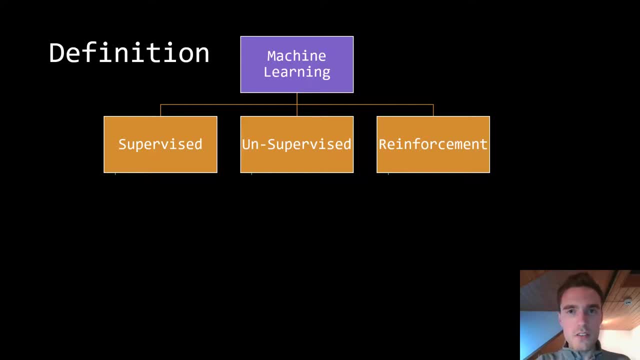 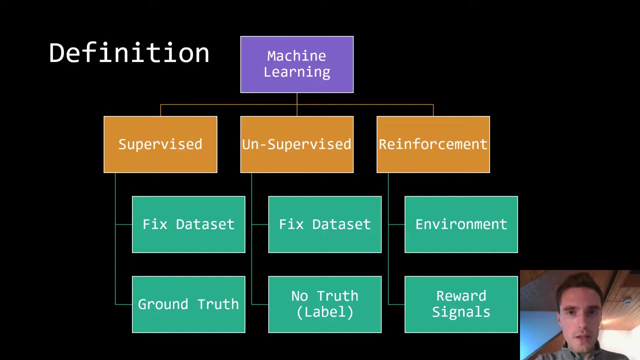 The environment means you are interacting with it. You are the agent and you are interacting with it over steps. This is the first difference you can have. The second one: in all the three cases, you will be giving answers, And the question is then this: answer, how is it evaluated, How is it assessed? 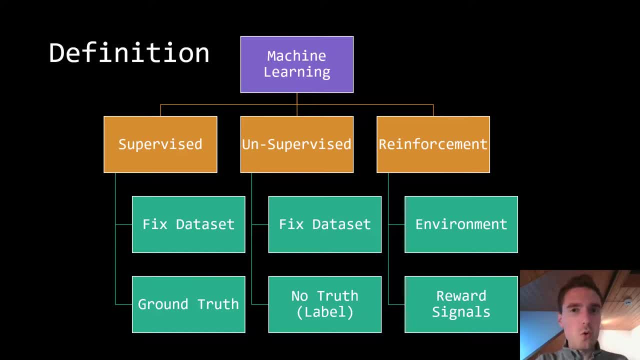 For the fixed data set. you can have a ground truth, It can be called a target, It can be called a label. You have something to compare with. This is not the case with unsupervised learning And, finally, this is very different with reinforcement learning since, as I said, you are doing steps. 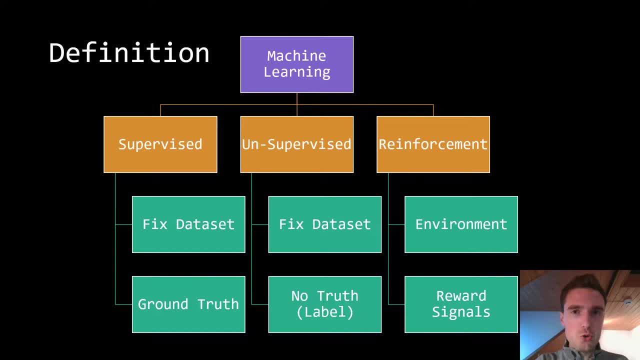 and for each step you receive a little reward, And what is important to you is, of course, these rewards, but more important is the sum of rewards, And that tells you if you act correctly or not. Let's take some examples. So here we have an images. The task would be to draw some. 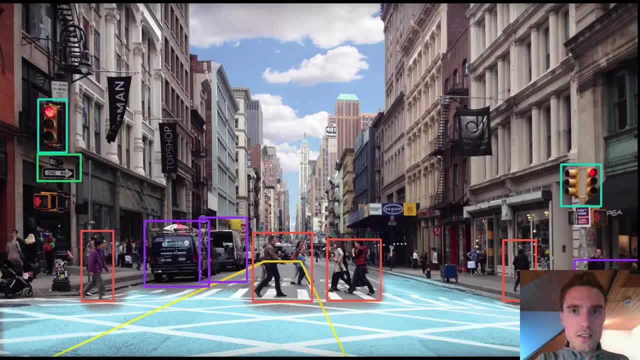 bounding box around the objects and to say to which class it belongs to. And then this is compared to some, let's say, ground truth. And the last slide. again, I'll give you a little detail on what these guarantees mean. So let's draw some questions right here. And a basic learning tool that everyone uses has. 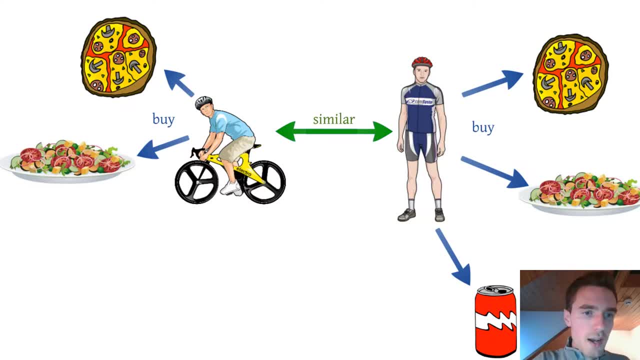 been a friend's mark for quite some time. And finally, like I've said, there is a competition about the choice of an object And it first comes down to you: Bitcoin or an asset which I know Josh and Atlanta really like. but I have no time to answer those questions. 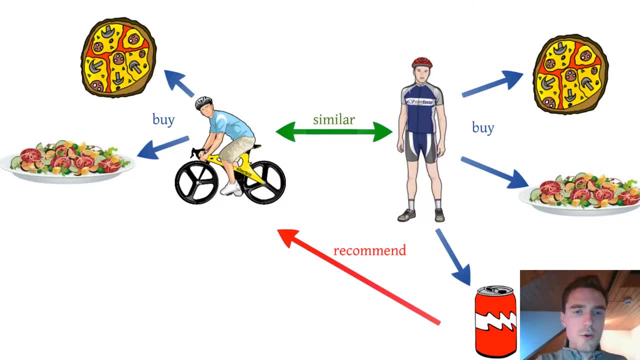 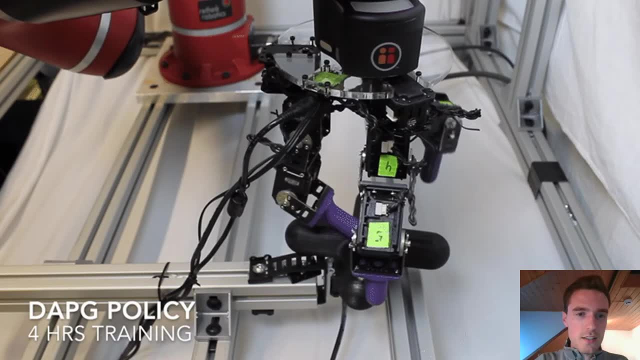 So I'm going to play it, like I'm saying: let's say Gold mining, let's play And having this, I'm going to give you some to say. now for reinforcement learning. this is an example where you have to try and to learn. 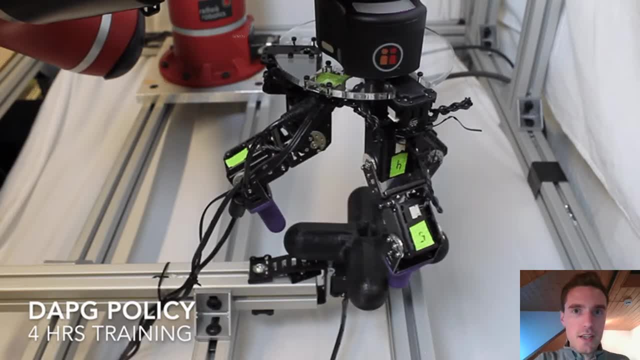 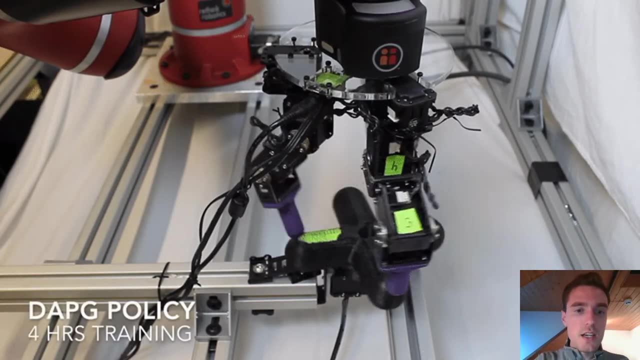 to turn this valve. at the beginning, you have no idea how to, so you might be stuck without doing anything for a couple of of minutes or even more. here you see, after four hours of training, is able to turn it and yeah, you are interacting with the environment, trying things, maybe the 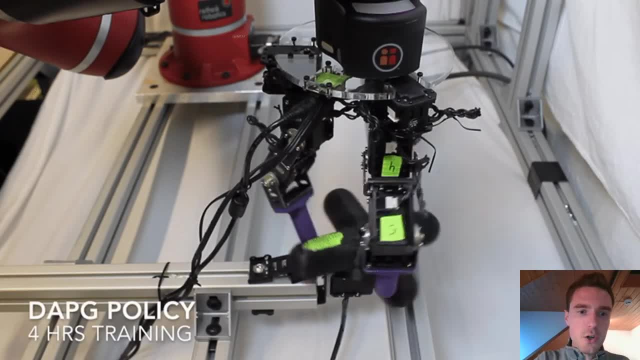 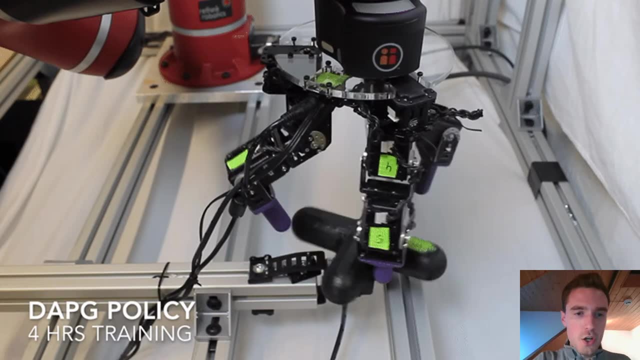 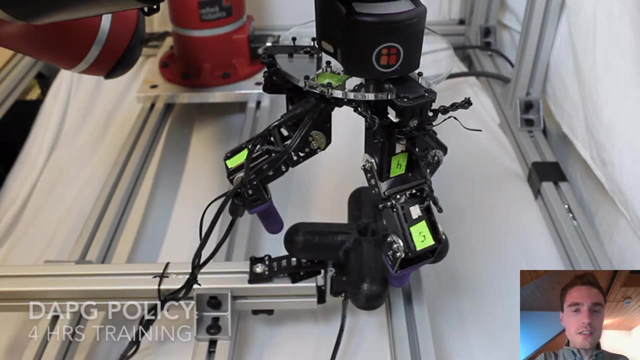 reward can be the angles. is it going the direction i want it to go? ie, i am turning the the valve in the good direction or not? so there are three conclusions now. the first one is for reinforcement, learning, union environment. the second one is it's a multi-step process. you can 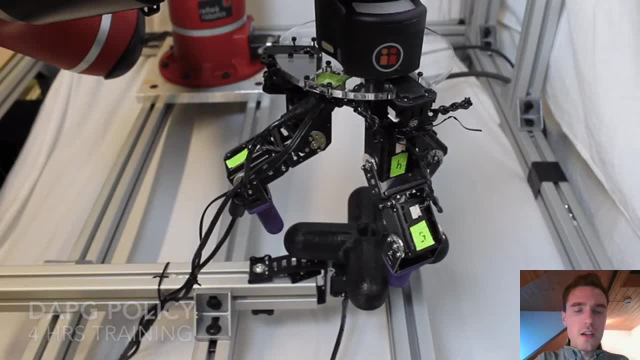 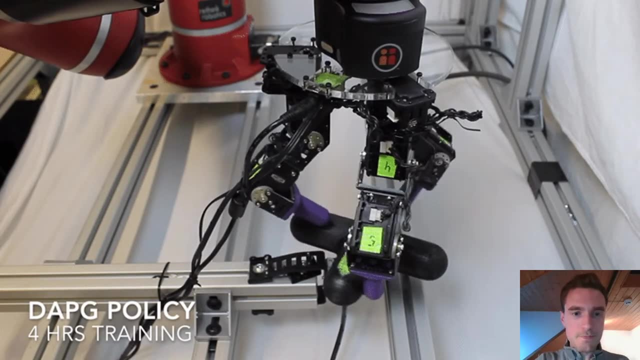 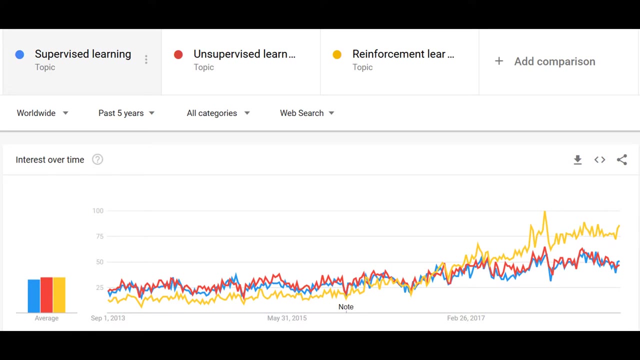 see, you can divide into time steps. and the last one is we have three subclasses for machine learning. they are not competitor, they are just serving different purposes. so the three are not in the same league. nevertheless, one could compare their popularity. so with the google research index we can compare unsupervised, supervised and 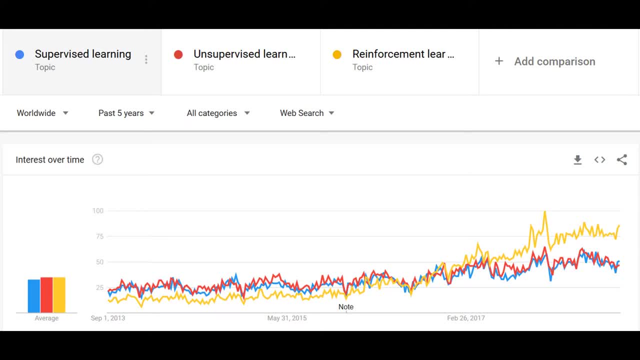 reinforcement learning. reinforcement running is appears here in yellow and you just see that it's quite recent and it's booming. and in the in the international conference of machine learning in stockholm this year, the biggest room was for rl and me, which is the primary- most of the papers were covering this topic. 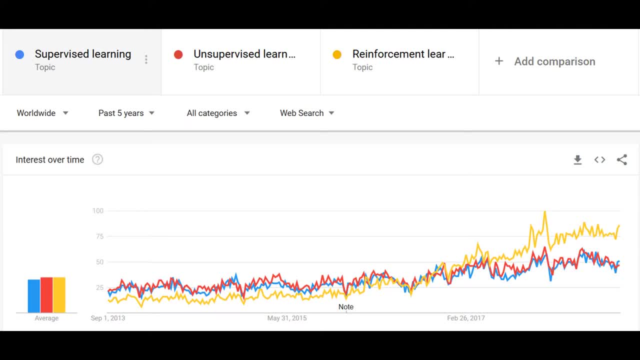 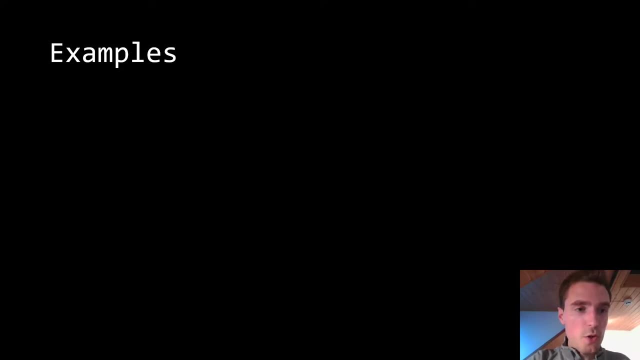 So a huge interest for researchers For applications. the application are limited for the moment, mainly on video games, robotic control and a little bit of autonomous driving. Let's see some examples about reinforcement learning for video games. That's the opportunity to introduce new concepts. 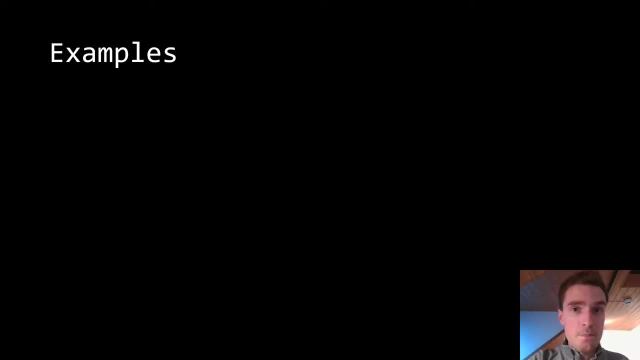 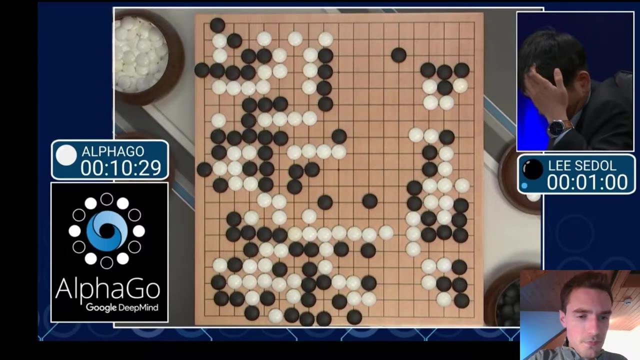 We have seen so far the concept of environment, the concept of step. Now let's see what a reward is, what an action is and what a state is With the game of Go. so what you have here is a board, and the board actually with the position of the stones. 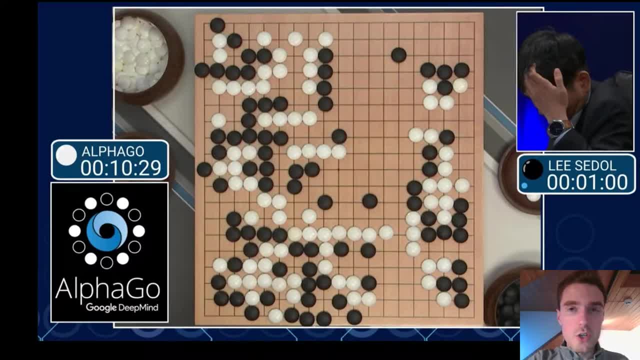 give you all the information you need to know in order to take action. So what you wanna do is take the position in the grid and code it in a array, for instance, and that will constitute your state. Think of the state as the configuration or the description. 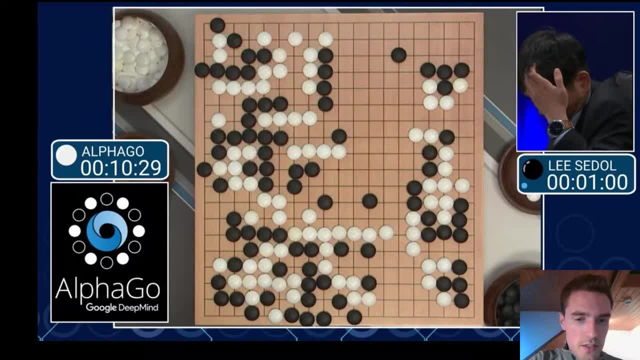 of the current state Or the current situation, and then comes the action. So one action could be: I want to put the one stone at the whatever position, and that will be an action. And then this is one step, Then you wait for the other to play. 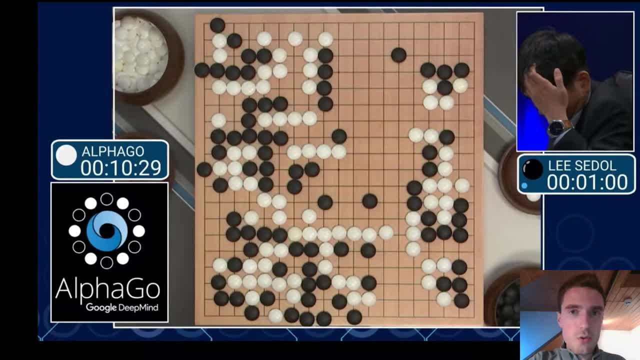 Then you have to do another step, And for each step you are getting a reward. It might be null. That's a choice on the designer. So what I can do is I put zero as a reward for each step apart from the last one. 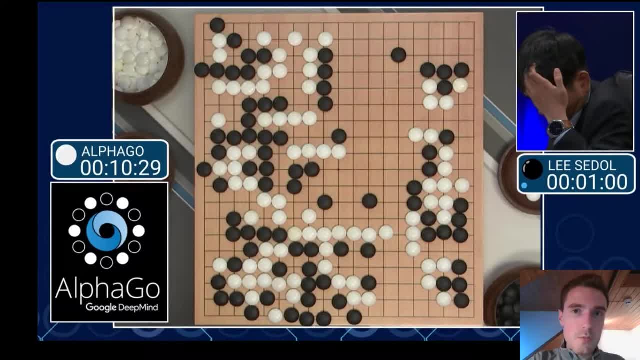 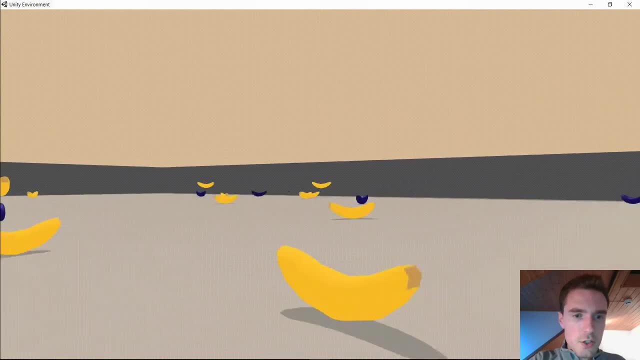 And if you lose, the final step you are doing will bring you minus one and plus one in the case of a win. That's the main idea about action, state and reward. This is another example taken from the Udacity course about reinforcement learning. 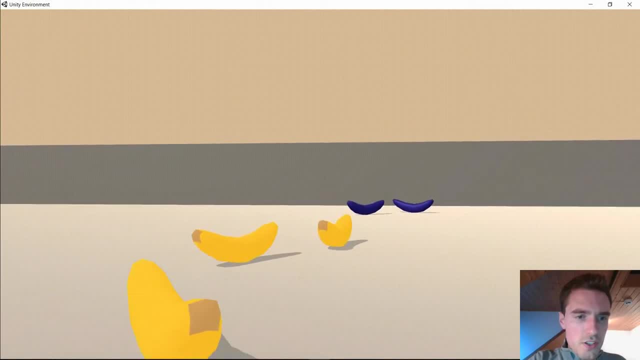 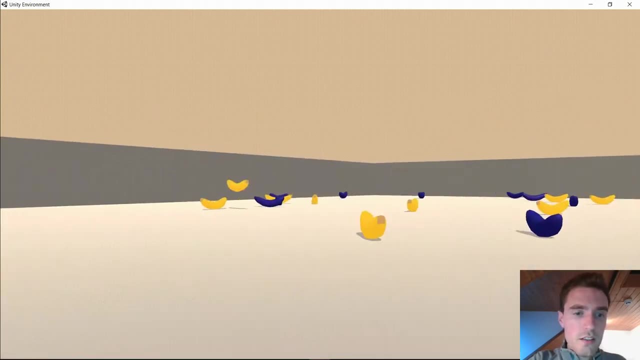 So what I was doing, my task, was to collect bananas. You see, the action is turning left, turning right. What is the state? One possibility would be to have the state as one screenshot, So each image is one state and the reward it might be null. 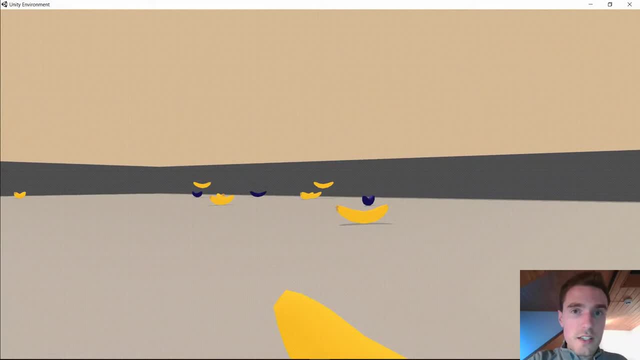 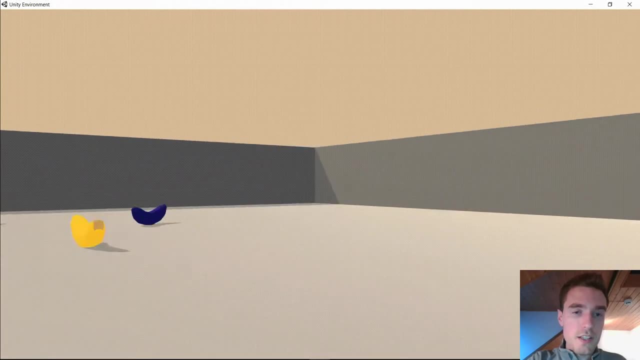 If I, for each step I do without collecting any banana, it might be plus one. if the banana I collect for this step is yellow And it might be minus one for the banana which I collect is blue. And you have the feeling now, okay, one step. reward is important. 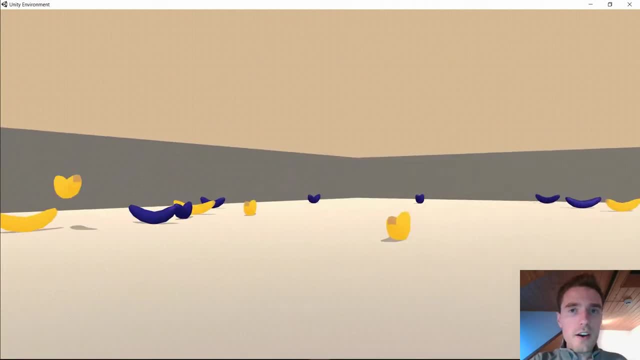 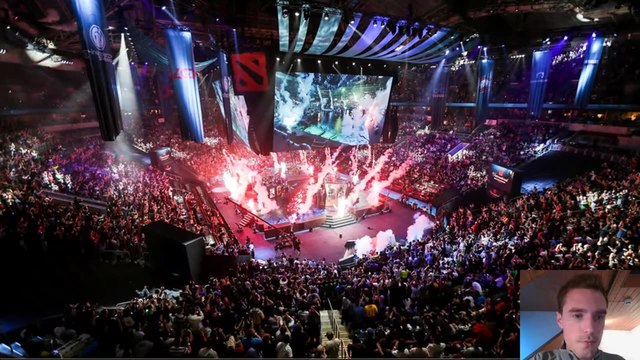 But what is more important is to collect all the time. So the sum of the two, Okay, This is the rewards I'm getting. This is what you want to maximize. This is simple games, Now serious business. So last month there has been OpenAI. 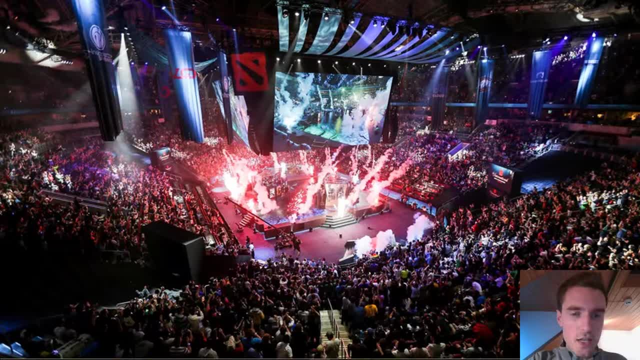 so research group for reinforcement learning defeating a former- some people really talented at Dota 2.. So Dota 2 is a game where you are in a team of five and you are fighting against another team of five. The difficulties here comes from three things. 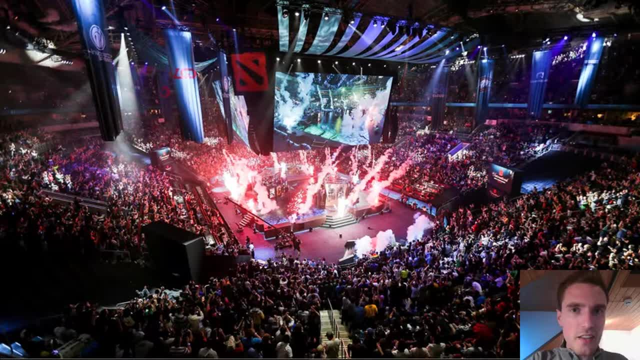 The first one is you don't have a full knowledge of the state. You don't know everything about the environment you are in, for instance because of fog or cloud. you don't have a full access at the description or the position or the position of the opponent is unknown for you. 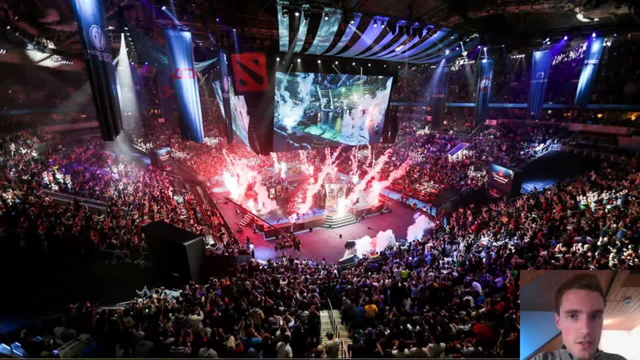 That's the first difficulty. Second one: you are playing in a team against the team. So it might be it is. it is actually Collaborative, you have to think of your teammates- and adversarial. so collaborative and adversarial. 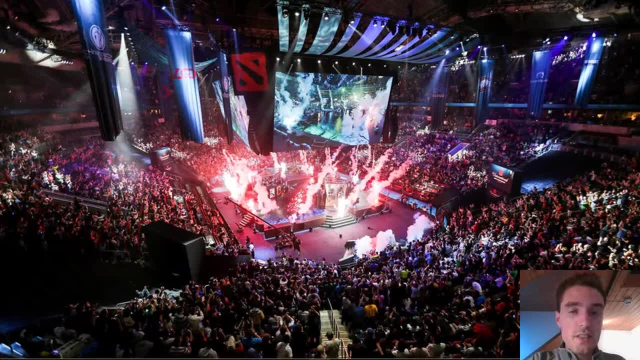 And this is not so obvious to solve. And the last one is that, compared to Go, this is a continuous time process: IE for Go: I'm playing, you are playing, I'm playing, you wait, and then it's your turn, and so on. 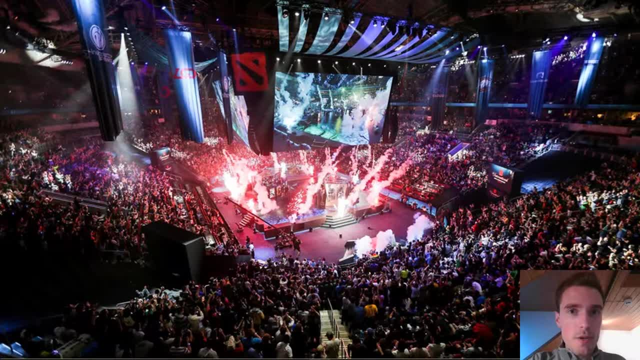 Here, at the same time that I'm moving, the other people are moving as well, So that makes it really difficult. So that there are a couple of examples for video games. Um, Atari is another one that now you can ask. okay, good, 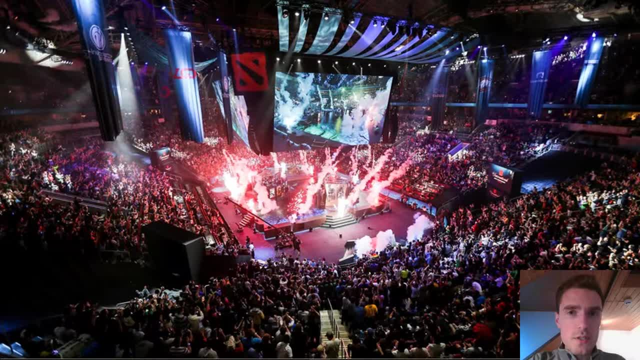 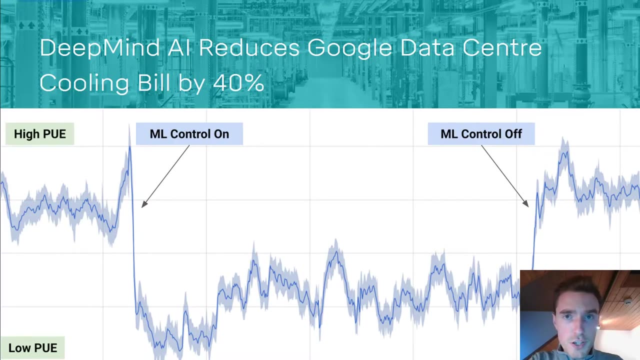 Why are you investing so much money in solving video games? And actually, this knowledge of reinforcement learning can be transferred to other domains, such as robotics and control, where there are much more money to earn. This brings us to the applications of RL in the domain of robotics. 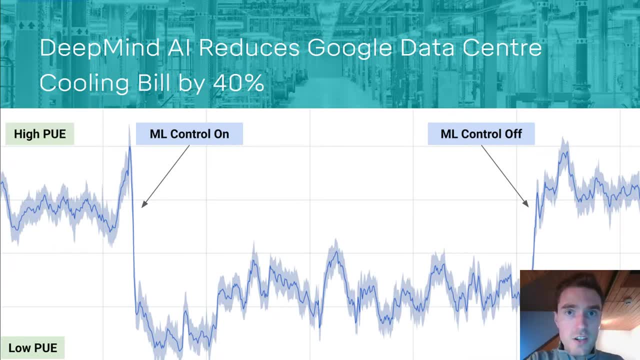 And control robotics. remember this example of the valve the robot has to turn And for control. this is a recent achievement covered by reported by Google about controlling the cooling system in a data center. The point of this slide is to show you that reinforcement learning is really close to. 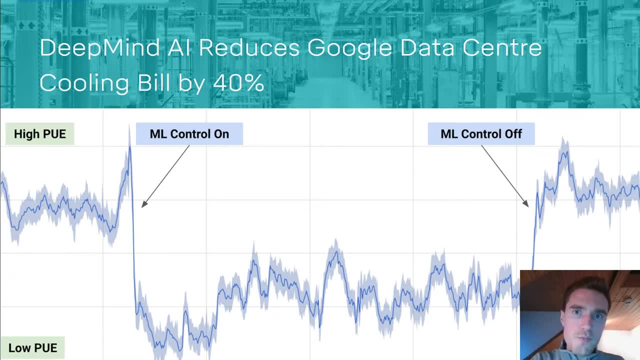 the control theory. It's not about perception, It's not about sensing. It's really about decision making and decision implementation. All the decisions you are taking, turning left, turning right. this is an idea, a decision intuition. they will be implemented as part of your interaction with the environment. 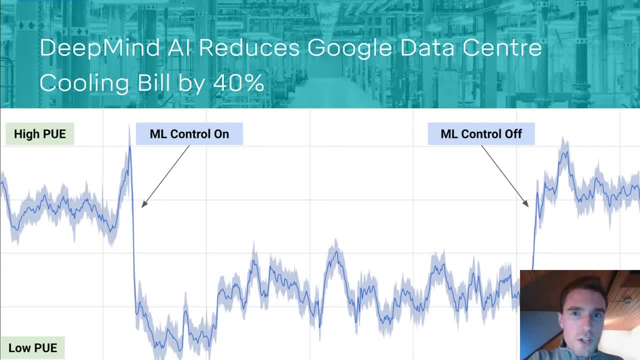 So have in mind, reinforcement learning is really about control theory, or close to control theory, and about decision implementation, as opposed to the perception field of RL. This is important to have in mind in particular when you try to apply RL to the domain of autonomous. 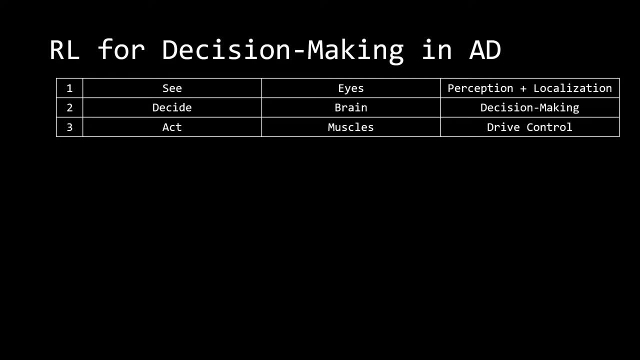 driving And, yeah, taking the modular, the classical modular pipeline of autonomous driving. So you start with perception. Your task is to identify where you are, your current speed. So all about sensing where are the others, where I am on the map, localization and perception. 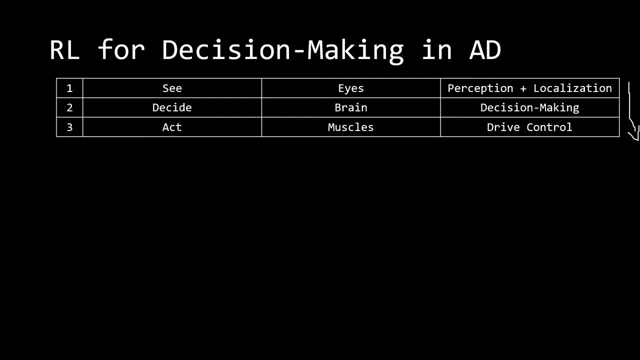 Then comes the task of decision making. When you Deciding, When you say, OK, I want to turn left or continue at this speed, And then this decision is actually implemented with a controller having the control of the wheels for the steering angles, or the gas pedal for acceleration. 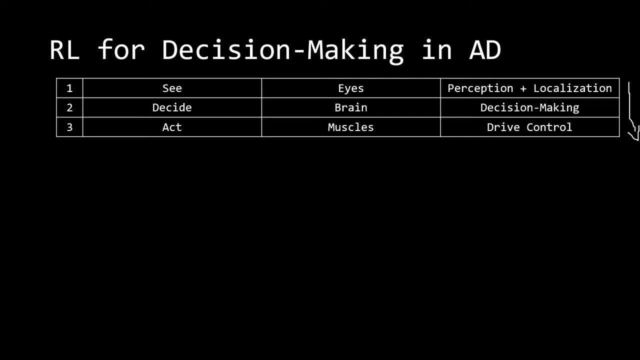 One could work parallel with the human, when we are using our eyes, then brain and then muscles to see, decide and act. And with what I've just been saying, reinforcement learning can apply to only the the line two, um, ie when you are making decisions and then they will be implemented, as opposed to perception. 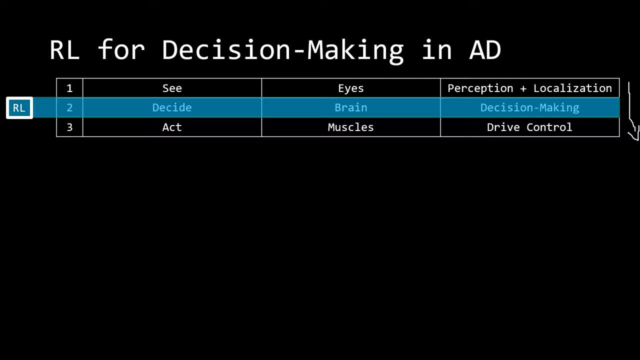 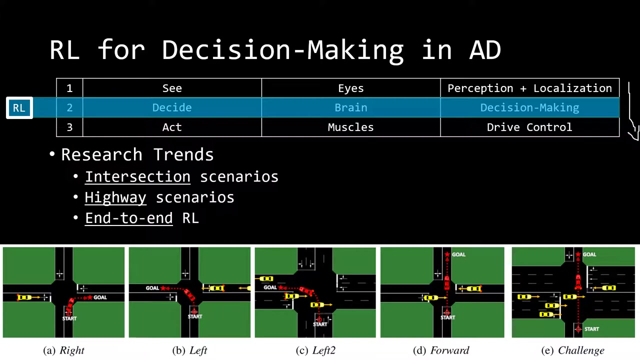 where supervised learning is- uh, is often used. this is a different, a different problem. so now there are three research we could- okay one could classify reinforcement learning for autonomous driving into three research trends. the first one is about intersection handling. so imagine you have different kinds of intersection to to address. it might be complex and the task, what is asked, is to 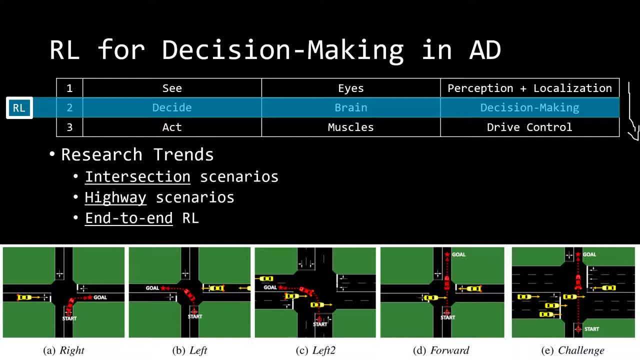 have something generic that can solve all possible configurations of of intersection. the second one can also use as an environment a simulator. this is a highway scenario. we will cover it in the next, in the next part. and the last one is end-to-end reinforcement learning, and we will mention it. 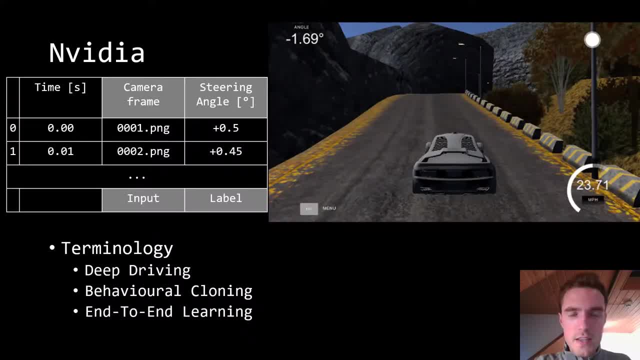 in the coming quiz time for it. let's take this example. so i'm giving you this picture. consider that it is a state and the action you have to to decide to take is: how much should you turn the steering angle of the car in order to stay on the road? that's the problem. in a simplification of what the 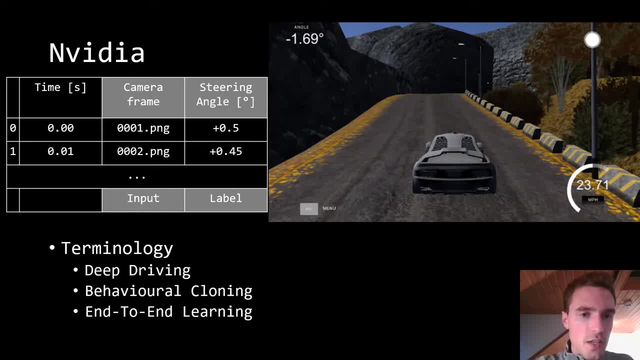 nvidia was reporting, and what they have done is they have asked a human to play the environment and then they are recording. they have recorded a for each time step, both the image and the, the decision applied, or let's say the steering angle applied by the human. so doing, you can constitute a big data set. and then back to the. 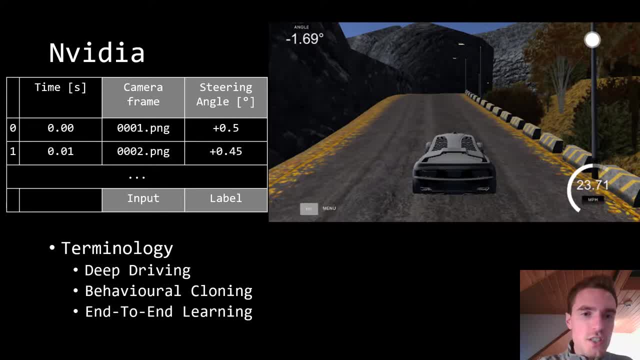 office. you can learn a model that matches for each image, gives you a value of steering angle. what i want to show you is that, okay, this works. we will see a video. this is oppressive, but this approach is not reinforcement learning. it's not reinforcement learning. it's not reinforcement learning. it's not. 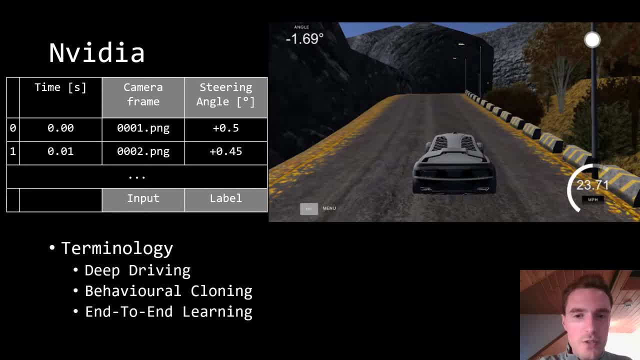 reinforcement learning at all. although i have been using terms like environment, steps and action state and so on, this is purely supervised learning. you have been using an environment, but not for training, only for recording data, and then you have been applying classical regression methods. so, yeah, be careful. i'm not so fan of this terminology because you 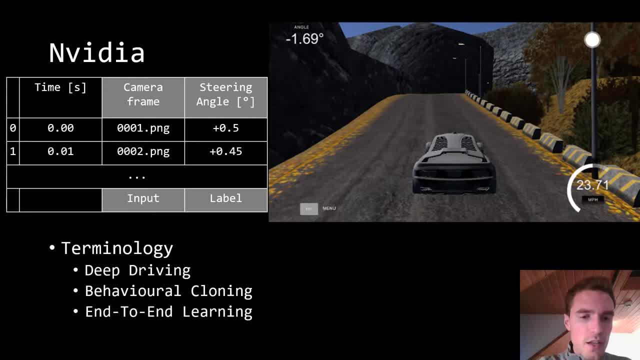 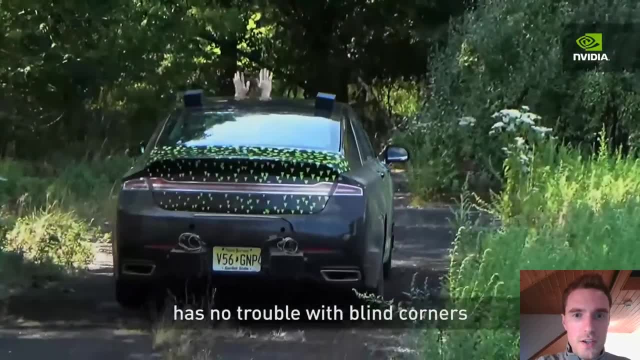 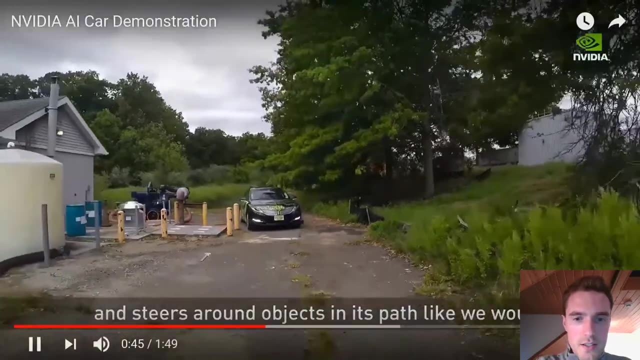 don't know which of the three methods of machine learning applies. be careful when reading it. and the video is quite impressive and the power of generalization it makes. this is yeah, writing, uh, everywhere. let's go a little bit further. also in the night you are able to to drive. 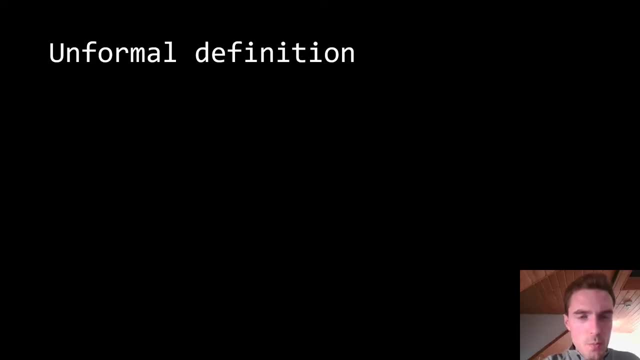 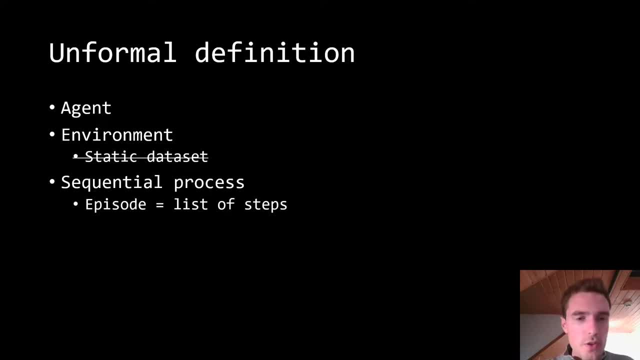 interacting at each step with environment. a step- um is a basic- is the single second motion where you have to take an action and to transition from one state to another. what is called an episode is a list of steps which ends at the end or at the termination step. so concretely, when playing go. 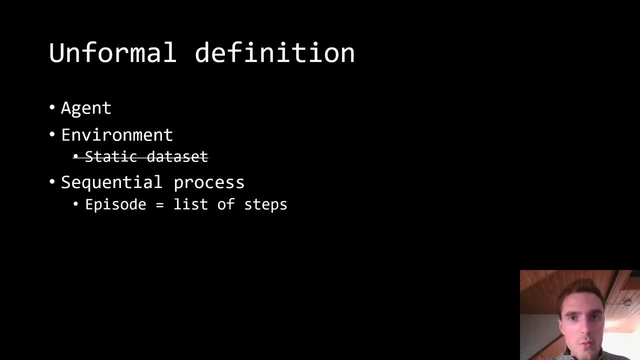 the episode is from the start until the end, when someone wins or lose. this is an episode for each step. we have seen that, for instance, for the bananas, we get rewards minus one, zero or plus one, and what is important is we are trying to maximize the sum of them. we collect them and we try to maximize the sum of it we have. 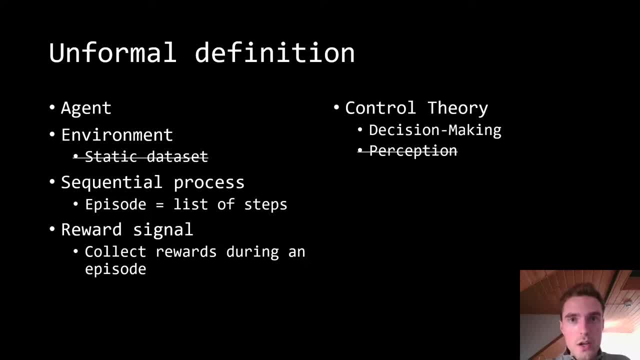 seen that reinforcement learning is quite close to a control theory in the way that your decisions turning left, turning right- will be or are implementing directly in the environment. and finally, with the valve example, we have seen that it's really about trial and error. so you start having no idea you might be stuck with this valve not turning it for. 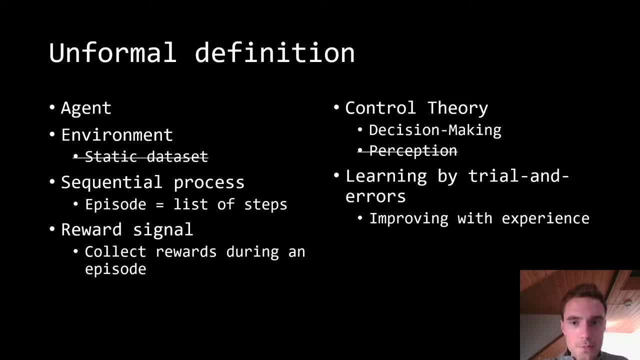 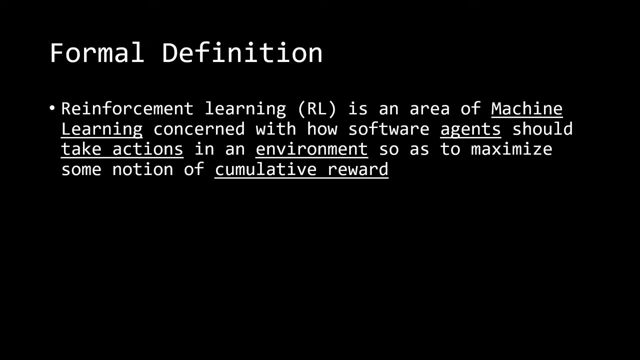 a couple of minutes, but then trying to get it better and better and we improve with him with with the experience. that's the informal definition now. so a more formal definition, reinforcement learning, is an area of machine learning concerned with our software. agents should take actions in an environment so as to maximize some notion of cumulative reward. 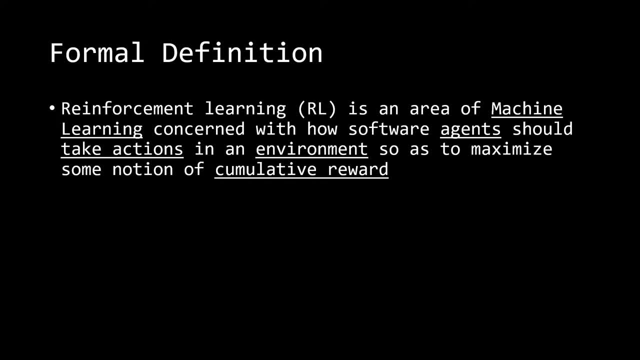 this is exactly what we have been um saying in the intuition. maybe just cumulative reward. again, what is important is not the one-step report you will get. what is important is to think of a time horizon. this horizon may be short, maybe long, but this is the cumulative um. 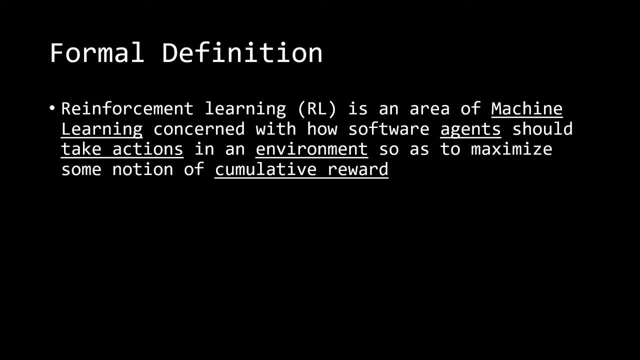 some the sum of the rewards. that is important. well, how do we start then? in machine learning, the environment is typically formulated as a markov decision process, so the modeling part is with mdp and you will find most of the problems are already formulated, defined. this is the case. 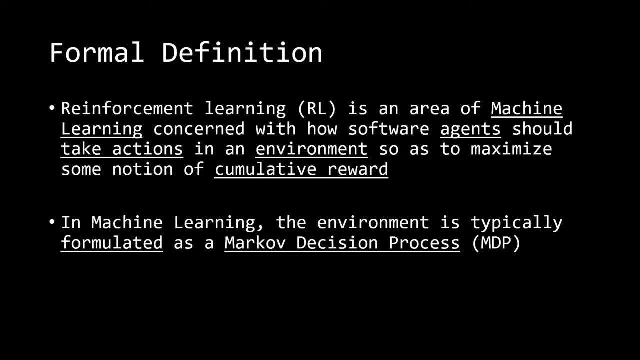 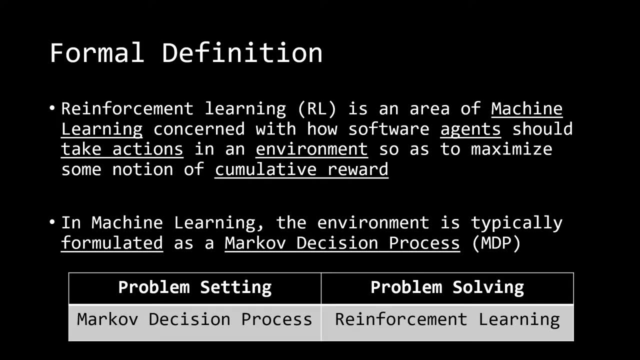 for instance, if you are playing with open ai gym environments. so the task is then to to solve the problem, but the modeling part is already done. nevertheless, i find it really interesting this- this is the reason why i'm mentioning it, and we will see how it works, but for the moment, 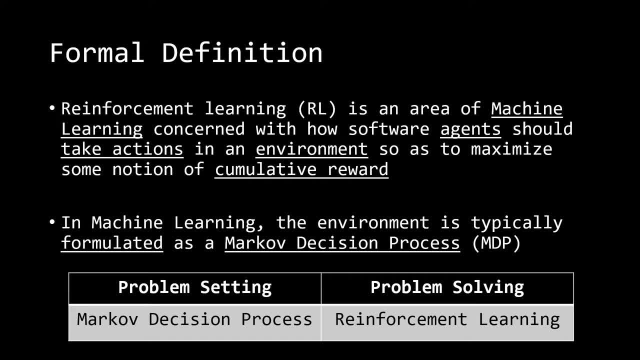 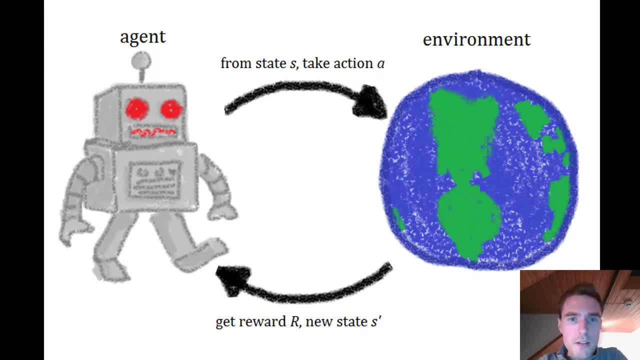 distinguish the problem setting markup decision process from problem solving using the reinforcement learning framework and to help us, this is the big picture to keep in mind. you have the agent playing with the environment. the agent starts. he's saying i'm in the state s i want to. 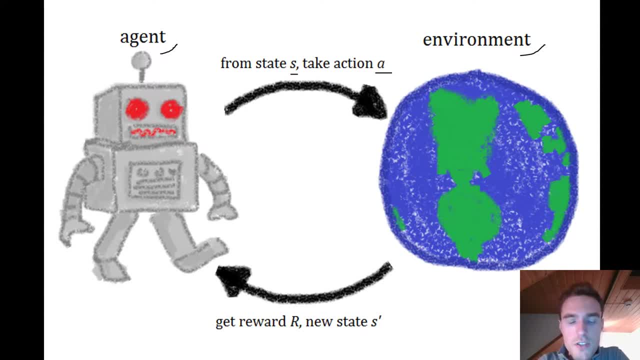 take action. a the environment takes these two, information and transition, to move the agent to a new state s prime and give our agent a reward error. so let's consider a very simple case, for instance, where the state is you're driving velocity in the inner city. yeah, 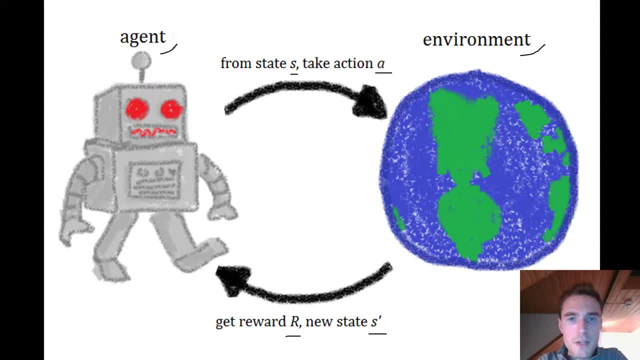 so only one information: in the state you are at speed 50, this is s, and you want to speed up, this is a, the agent. in this case, the car will take you at speed, let's say, 60, so more than 50. so you have speed it up. comes with that the reward, which is negative in this. 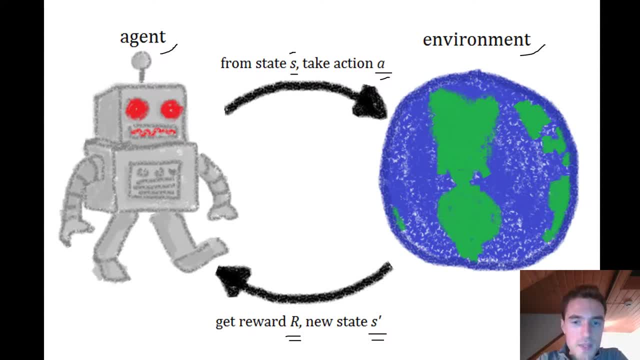 case, because this is bad to drive too fast in the city. and that's basically constituting one step. what does the agent can do of from this one step? It collects the four information, so S, A, S' and R, and this constitutes a tuple, tuple of four elements and you can store this tuple in the memory of the agent. 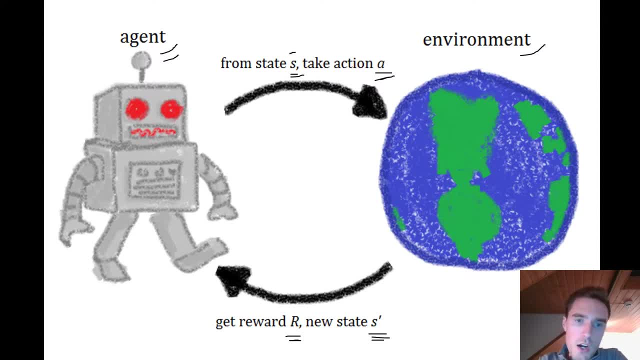 And for the next time, the agent will use this experience to adapt or improve his model and won't probably speed up while being at 50 kilometers. This is to me exactly, or really similar, really close to how humans use experience to adapt their action. for the next scenario. 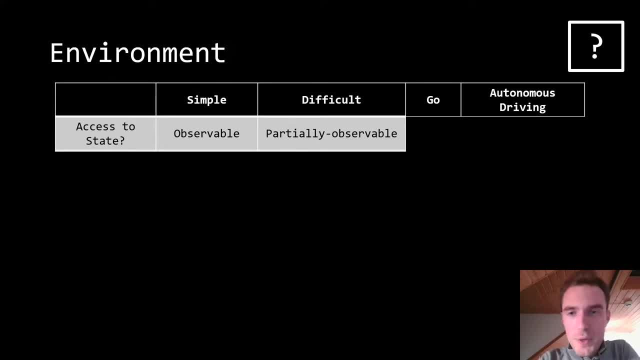 So, before we move to MDPs, a quick quiz about the environment. I will be comparing, or we will be comparing, the game of Go and another environment of, let's say, autonomous driving, for instance, urban environment where you have to decide which maneuver to take. 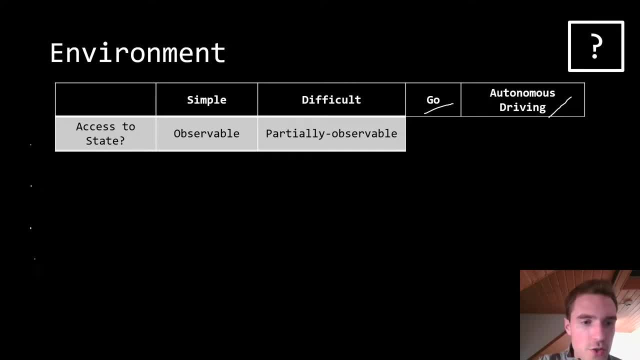 There will be a list of rules, There will be a list of criteria, And for each criteria there will be a simple and a difficult version. And the question is which of the two applies to both Go and autonomous driving environment? The first one is about the state. 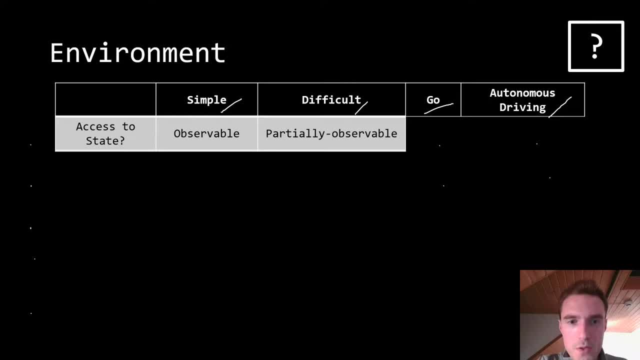 We have said the configuration, all you need to know, or all you could know about the situation. And the question is: can you have access to the full state or is it only a part of it? So for Go, remember You have this grid and both players actually see the full grid. 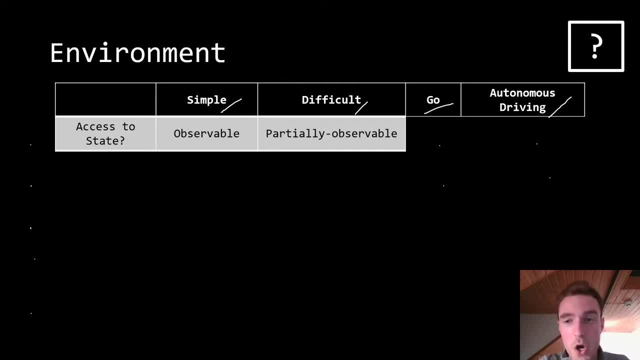 So it's a fully observable case. On the other end, for autonomous driving, you have no idea if there is a car in front of the truck you are following or if there is someone coming from left at the next corner, if there is a building in between. 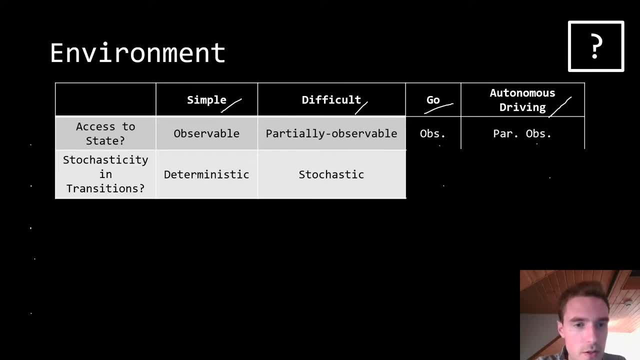 So that's the first distinction observable, or partially observable. Now about stochasticity in transition. What does that mean? Remember, we make decisions and we give this decision to the environment, and then the environment take us, move us to the next state. 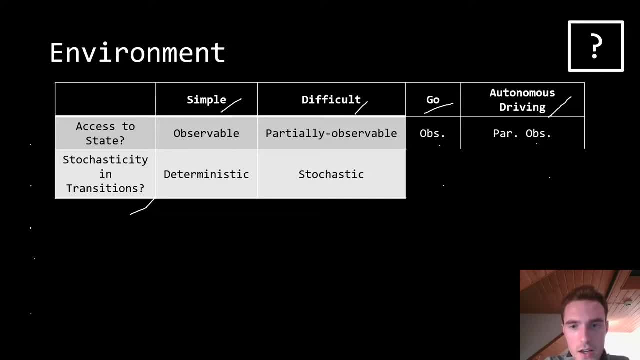 The question is: when moving us, is there any randomness or stochasticity For Go? there is no, Because when I think, OK, I want to move or I want to put this stone at this place, this is 100% sure, because I'm in control of it, that this stone will end up at this place. 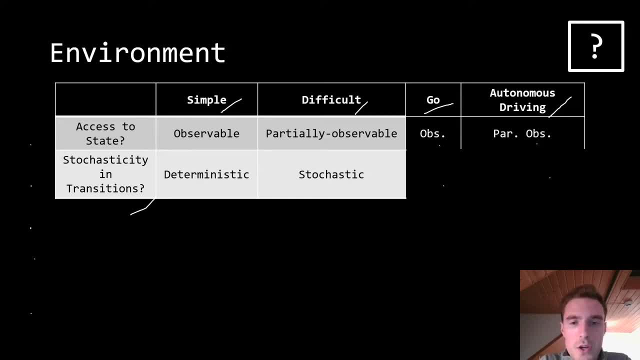 On the other hand, for autonomous driving, let's say: your decision is OK, I want to keep to be, to stay in the middle of the lane, But for some reason you are close to the sea, or whatever, and there is a strong wind coming from the left. 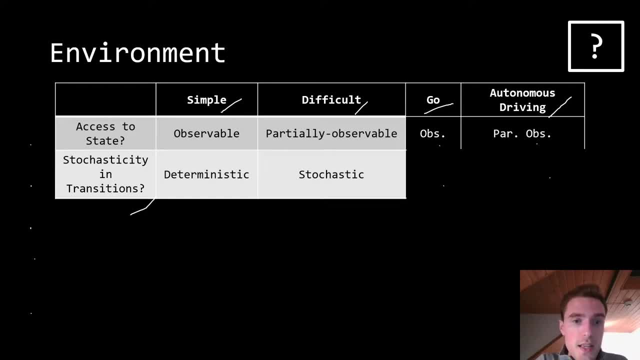 Suddenly, you couldn't predict it, And then it moves you. But then the next state: you are not in the center of the road, Not anymore, Although you thought, OK, I'm doing the right action to keep this state. So, stochasticity in the transition versus deterministic transition. 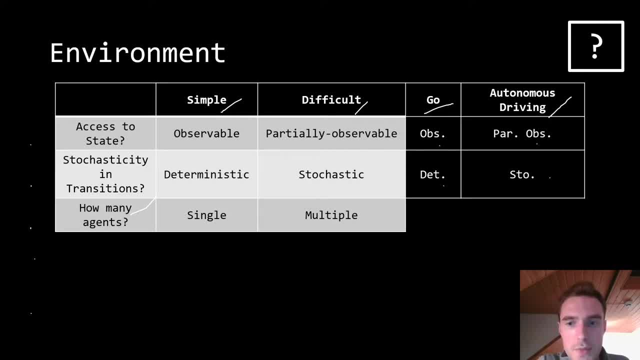 How many agents? That's quite obvious. It can be adversarial or collaborative. It is adversarial for Go. It can be both. for autonomous driving, OK, multiple agents. The question for autonomous driving is: do you want to collaborate with the other participants? 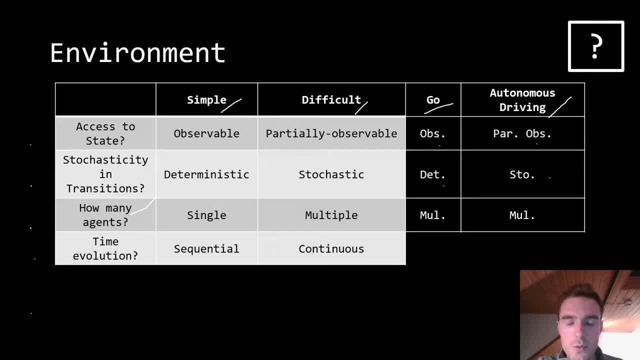 It's possible with communication protocols, And this is what is called V2V, vehicle to vehicle. for instance, The time evolution with Go: I am playing, Then I stop, Then you are playing, Then you stop, Then I'm playing again. 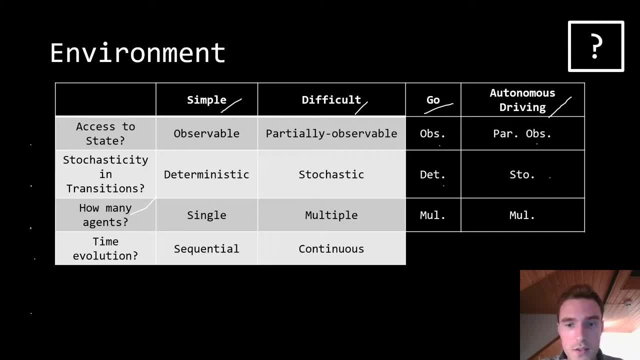 And so on. So this is sequential. This is continuous. All agents are moving at the same time. for autonomous driving, State space. It can be, of course, discretized in the case of autonomous driving, But it is originally continuous In a sense. my velocity is something continuous. 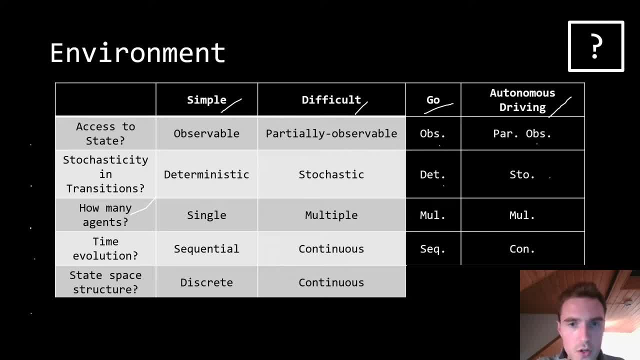 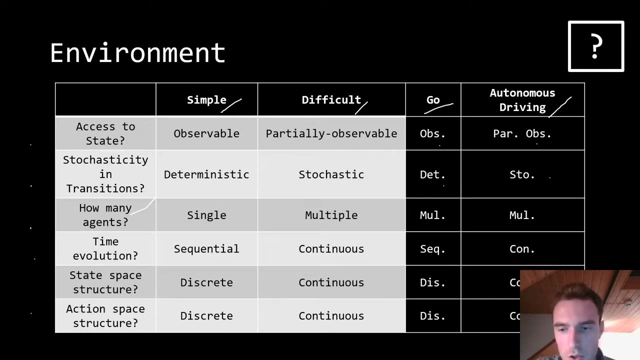 It's encoded with a float. On the opposite, the Go, You have a grid so you can code it with integers. It's totally discrete, And the same applies to the action space: Discrete for Go. Continuous for autonomous driving. What I want to show with this slide is that autonomous driving contains all of the difficult parts. 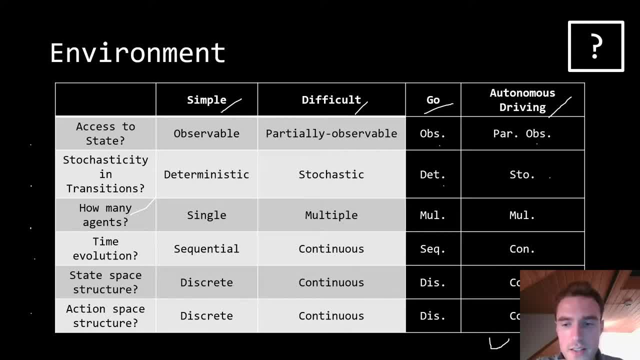 There are simplifications to make, of course, but it is at itself, from scratch, a very difficult problem. What does make the difficulty from Go? It's about the state. The state is really huge And it's about the delay reward. You are playing on average, 120 steps in one episode. 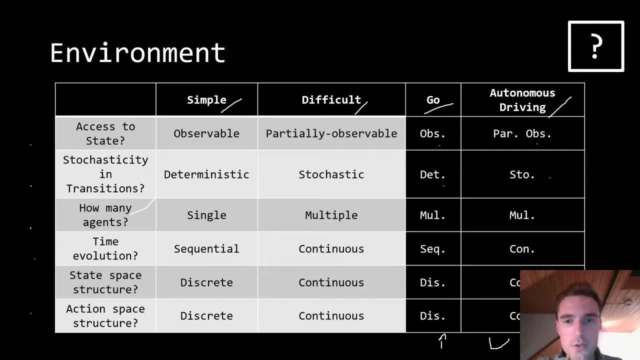 And you only get one reward at the end of the 120 steps. So that's the difficulty. That was about the environment. Now let's have a look deeper in what the MDP is. So MDP Markov Decision Process: We will start easy, ignoring the decision. 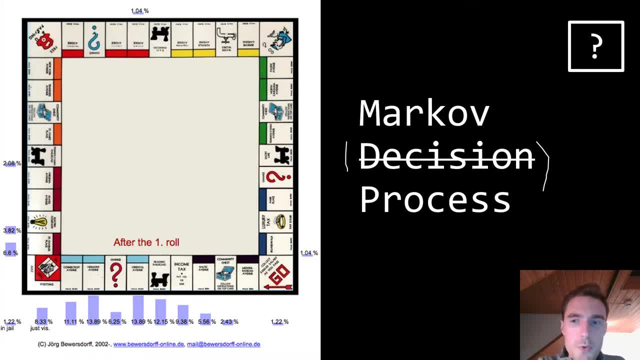 So only Markov Process. There will be a quiz. We will be using this example of a monopoly, So we'll take an easy version of it. The point is to illustrate again three concepts. The first one is the transition function. 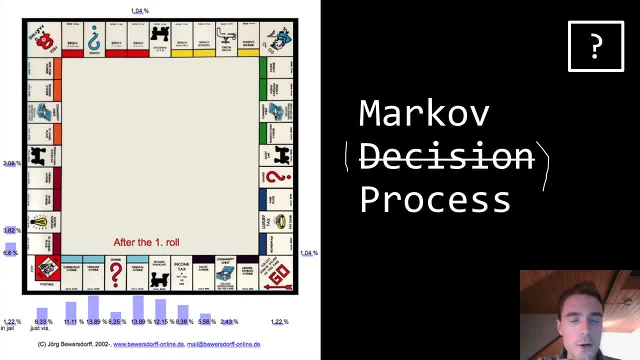 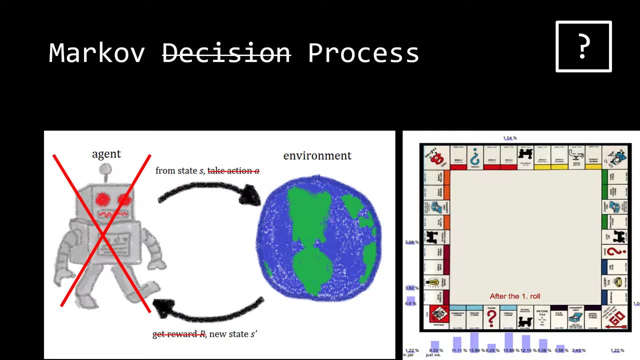 The second one is the state. We have already mentioned it. And the last one is about the Markov property, of course. So we just said: we ignore the decision part, So we don't need any agenda. So we don't need any agenda anymore. 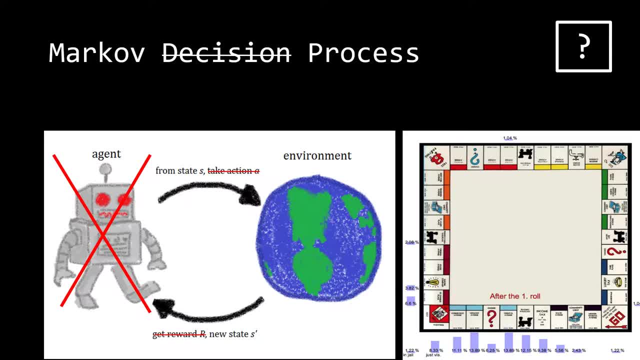 There is no action being taken, There is no reward being given. We are just spectator, in a sense, of a transition from state S to state S prime And we are playing with this board. So if you remember the previous classification, you can say this is a fully observable environment. 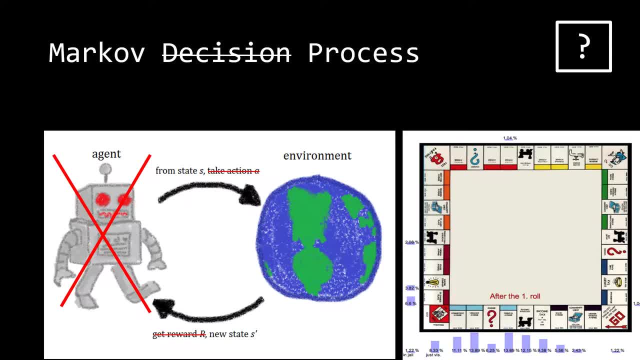 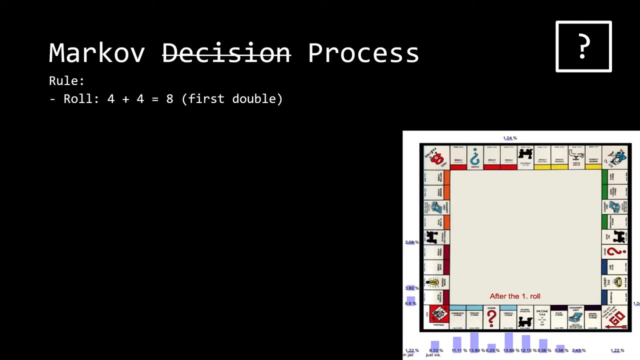 It's also discrete in terms of state. There is no action And, the most important part is, transitions are stochastic. Stochasticity means they are randomness induced by rolling the dice. So now, having said that, let's define the rule. You have two dice. 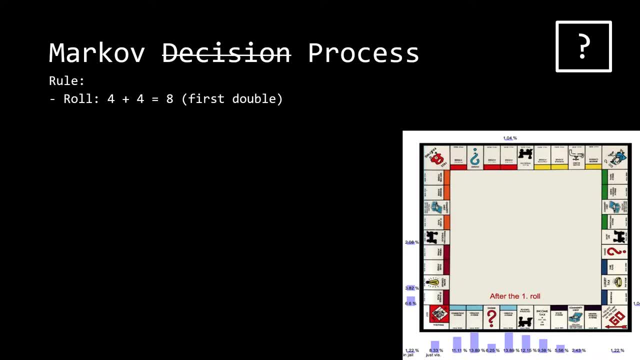 You roll them and then you move according to the sum of it. So if you are, you move eight forward. in this case, You do that all the time, except for one condition, And this condition is based on double. So here you see four plus four. 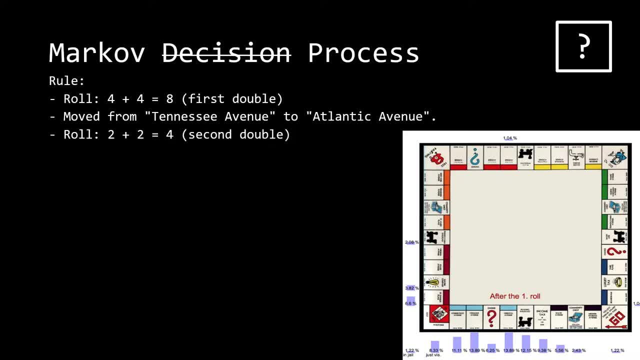 You have made one double. If you do a second double just after, then it's a double double And then you go to jail. This is one rule. Let's go with it. The question is, how do we encode the state? 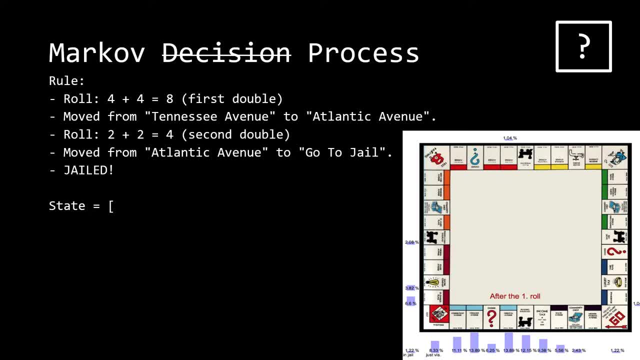 Encoding the state means or designing the state means. which information do we need Or how do we describe the configuration or the current situation? Obviously, we need a position, So there are 40 positions in this board. We need also the information about: in the previous step, did we get a double? 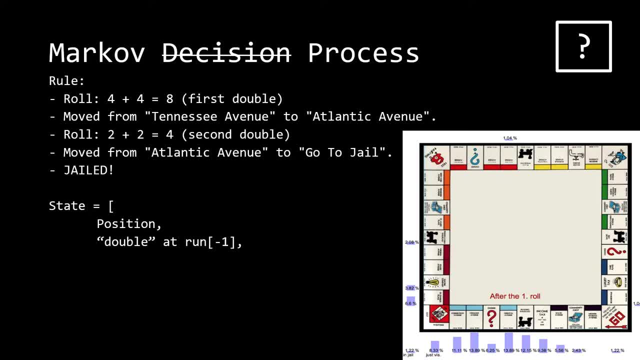 Yes or no, And then in the previous previous step did we get a double Yes or no. OK, that's our state Now. we just leave the process run and then we observe it. And one question could be OK: how much time is spent on average in jail? 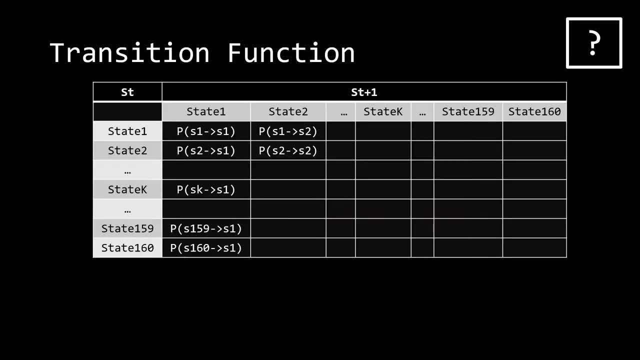 This is a question I am leaving to you All. right Now, let's take the opportunity to mention two concepts: the transition function and the Markov property. What we have said is that in our state, we have the position. How many positions do we have? 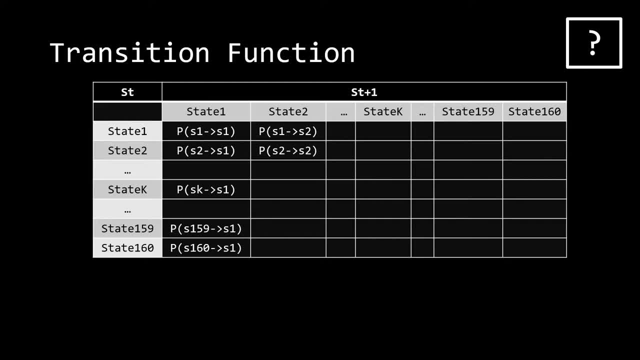 40. We have also a Boolean ie yes or no about the previous double. So two possibilities And another two possibilities for the previous previous double. At the end of the day, we have 160 states, So you can think of our current state to be one of these. 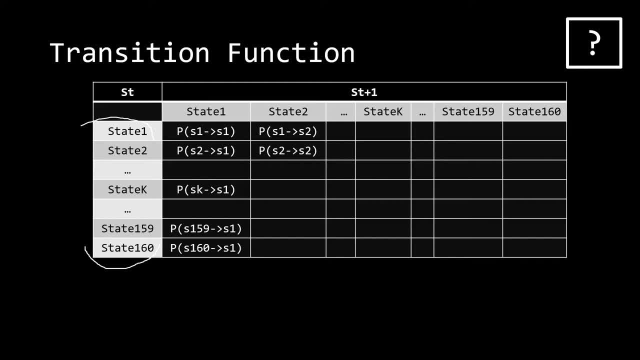 And then one question we could ask is: these are the candidates for the S plus one in the next step. So where do we go, Where do we step in? And the answer is given by the probabilities, And this is, for instance, the probability to go from state one to state two. 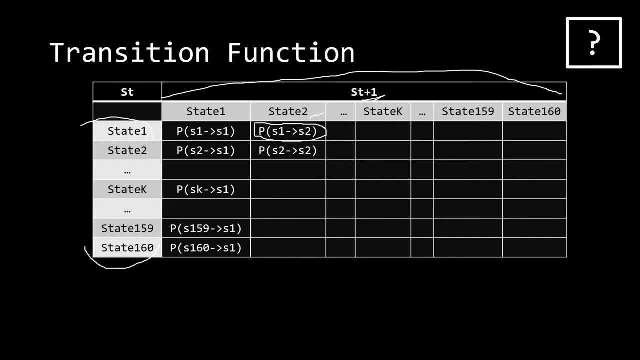 And you can fill this table, transition function table. What you see is that in order to predict the state S t plus one, the next state, you just need the S t. Nothing else is needed. S t minus one is not required to do this computation. 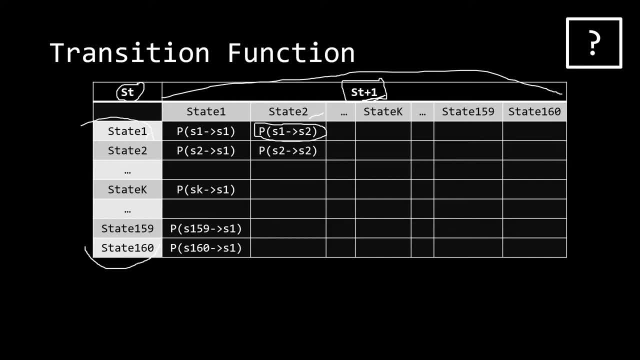 This is because the state was designed, let's say, correctly, or at least it holds the Markov property, And the Markov property says S t plus one. The state at time t plus one only depends on S t the state at time t. 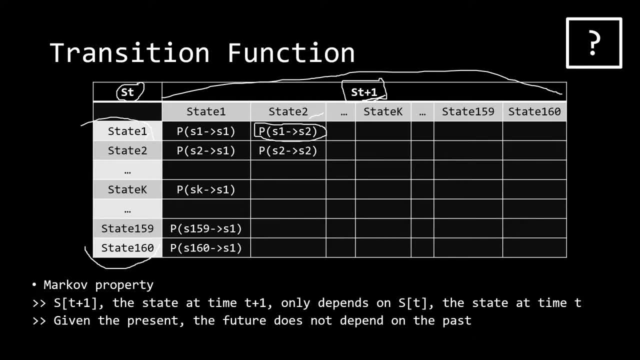 In other words, given the present, the future doesn't depend on the past, And this is a strong assumption for most problems, but really useful. In particular, you can think of what happens for the memory If we don't have this property and if we have to store or to consider. 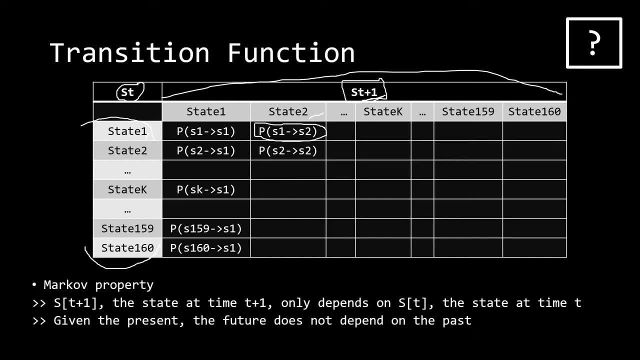 I don't know the last hundred states to predict the next one. It really, really quickly becomes intractable. Here we have already 160 states. You can think of problems where there are way more and doing the combinations, it becomes expansionally or really quickly intractable. 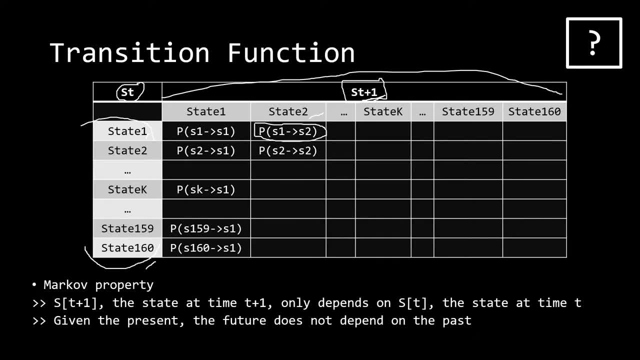 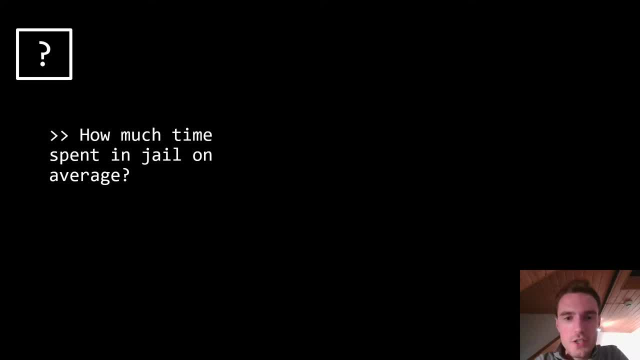 That's a strong assumption, but useful and proper to this Markov decision process. So remember the question: How much time spent on average in general? Now that we have this table, this transition function probabilities, it can be used to solve this question analytically. 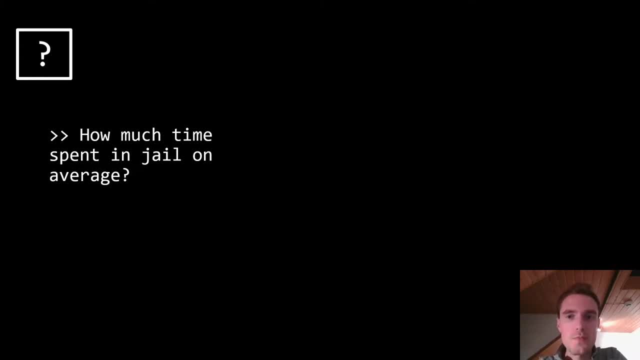 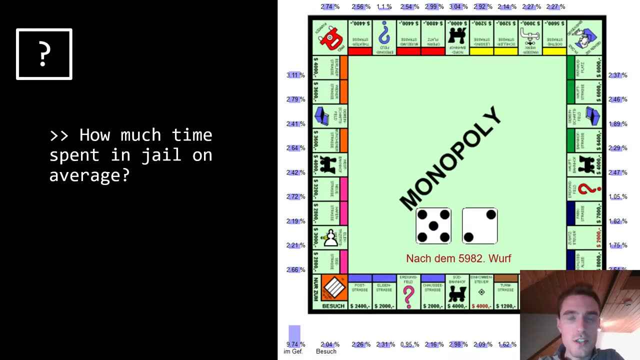 Otherwise, what you can do is go for Monte Carlo methods, And it has been done here. Again, the source and reference is available in the description of the video. So with this example, we have seen a Markov process where there is no decision. 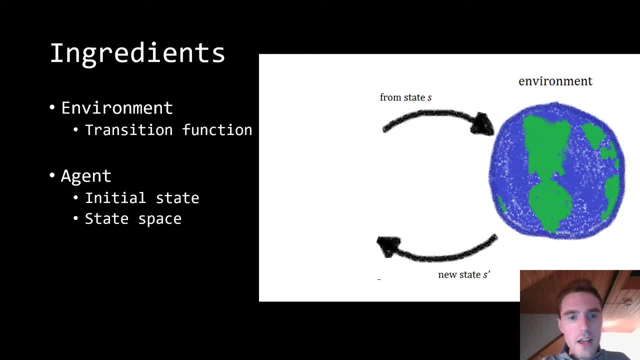 We saw the transition function, The initial state and the state space we designed. Now it's time to introduce actions. So actions and reward. So we see, now it's agent back, We can make decisions, We can change the world, so to say. 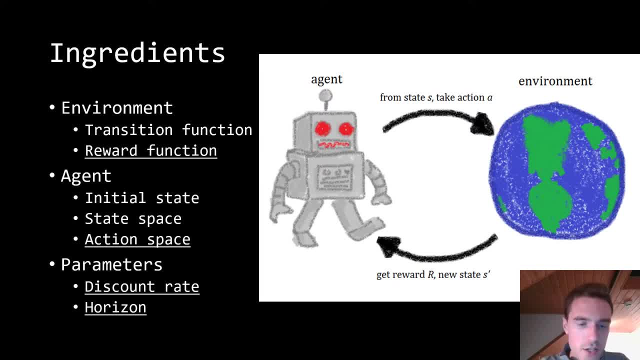 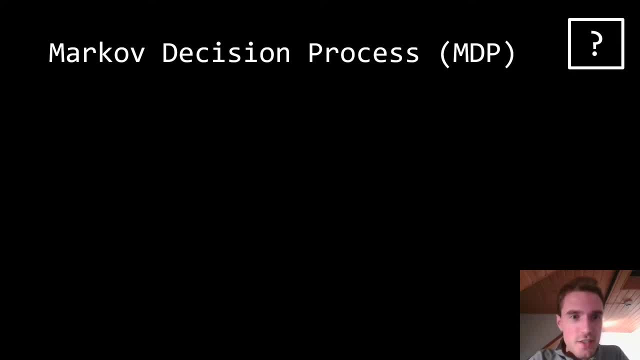 And we will introduce reward function, action state action, space, Sorry- And two parameters: the horizon and discount rate. So let's see the definition of a Markov decision process. We have said it's about modeling- Modeling a decision making problem. 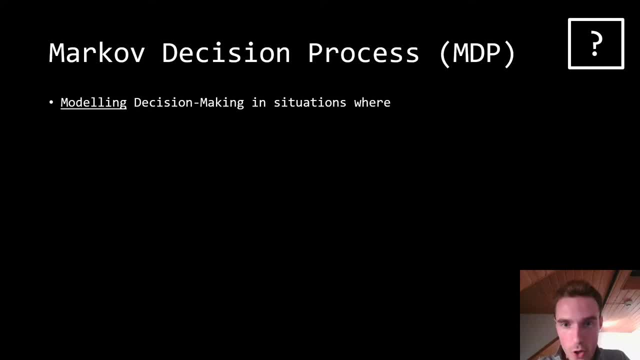 And we have two components: stochasticity and control. Stochasticity: this is the monopoly example where the outcomes comes from randomness. We have no influence, no impact, We are spectators. But in Markov decision process now it's partly under our control. 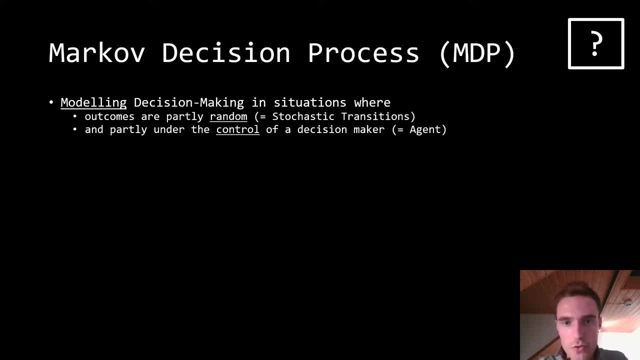 There will be some wind on the road So we won't control everything, But at least turning left and turning right won't have the same impact. The Markov property has to be included in it in Markov decision process. Again, next state is only a function of the previous state, and this time action and the previous action. 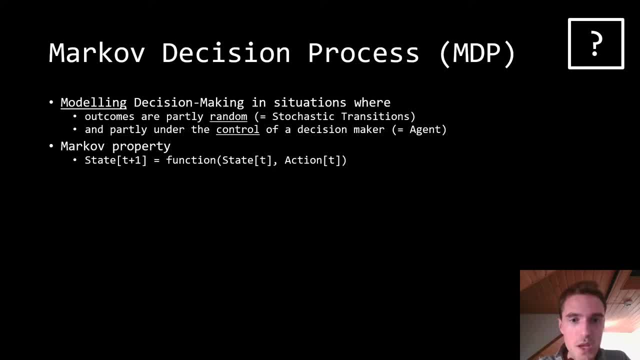 Of course there is stochasticity in it, but there is no part reserved for past. You can ignore the past if you are the current state. It holds all the information you need to add. Now introduce what's called control. Control the policy. 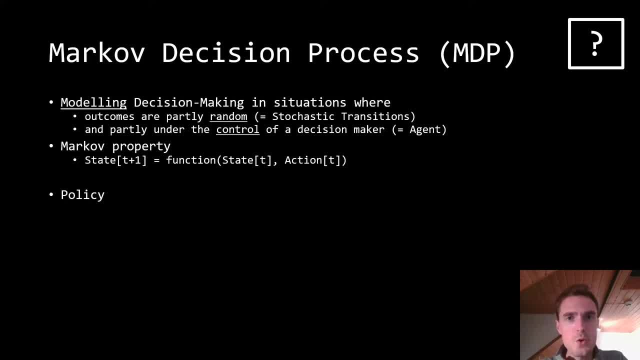 We have mentioned state and action. When you are playing you might ask: OK, I'm in this state, which action should I take? And this is given by the policy. So the policy is a function named pi which maps, So a mapping function from state to action. 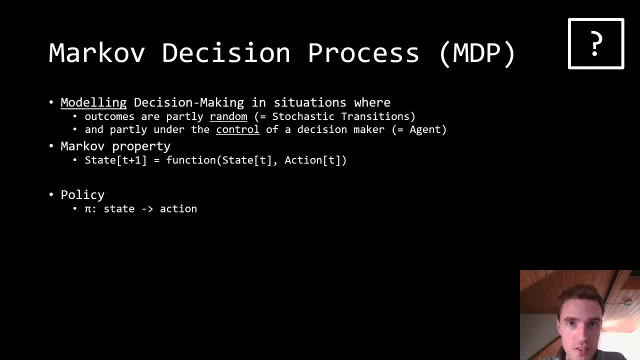 It's like a guideline or an instruction or a handbook. You read: I'm in this state, which action should I take? OK, according to this book or this policy, I should take this action If you are familiar with game theory. 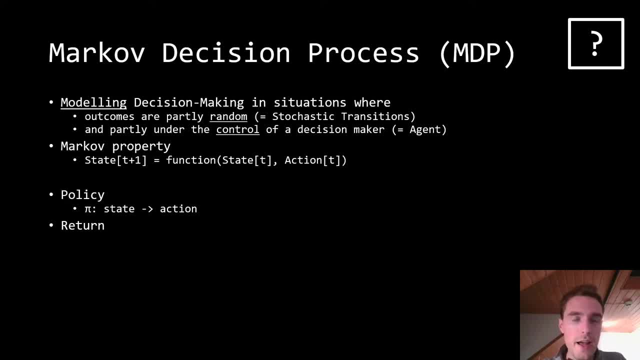 it's related to strategy, So strategy for game theory and policy for Markov, decision process, The return. So let's say, today you get a reward of, So this reward today, Tomorrow we get this one, and the day after, and so on. 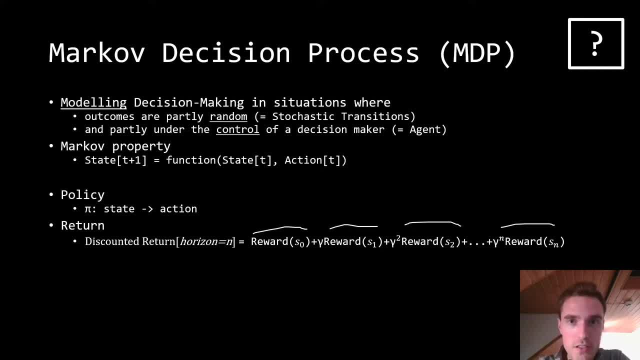 You want to do the sum of them, because we mentioned that this is what is important. But the reward you get tomorrow is maybe not exactly accurate, As important as the one you get today, Or especially if the day if the day, So if the reward comes in one month. 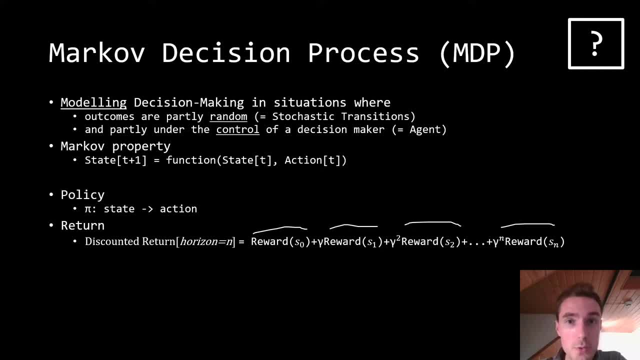 This is not. This has not the same importance as the one you would get today. That's the reason why you discount it. You discount each of them with a factor gamma that is between zero and one, And that you raise to the power of n. 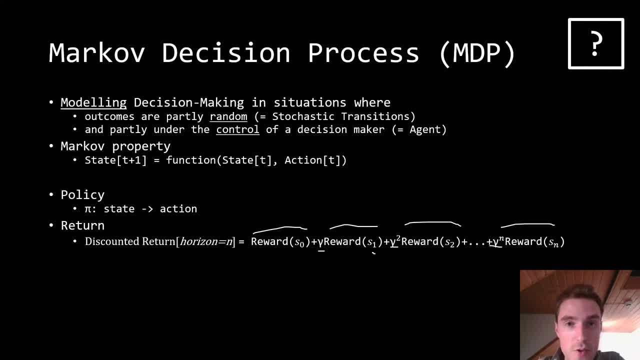 So here is one, is two, and so on. So gamma represents the preference you have for the, For the present over the future. If gamma is equal to zero, what does happen? Well, all these terms cancel. You end up only having this reward. 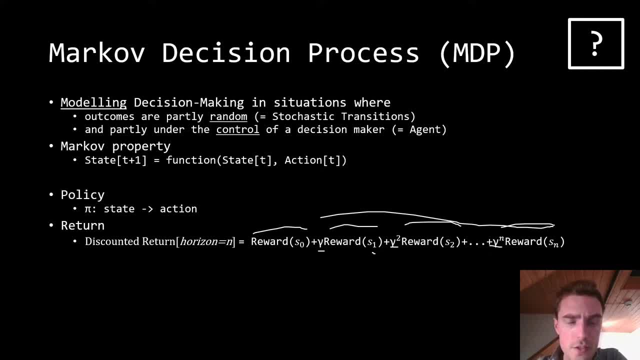 Otherwise with gamma equals zero. And so, to put it another way, if gamma is equal to zero, you only consider the very, very short horizon, But if, but if gamma is equal to one, then you consider them all equally. So you have to play with that. 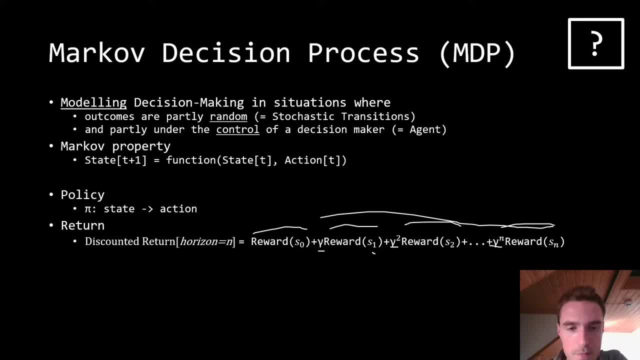 So this is called Discounted return over an horizon. and And then linking these two concepts, the policy and the return. The policy says you what to do in one state, So we introduced the expectation over this quantity When following pi. So this represents: 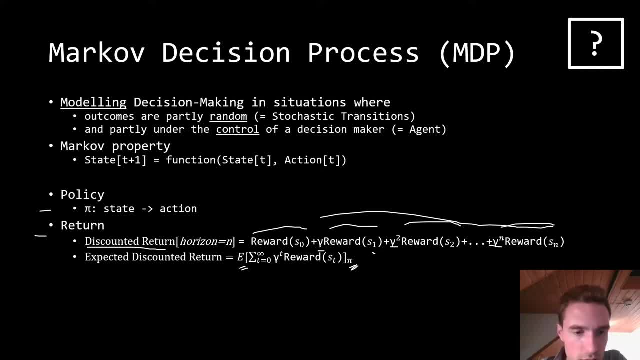 So this is the expectation when following pi: This expected discount return. What it is, It's actually The sum of the rewards Discounted That you should get on average. If you listen to pi for each of your decisions, This is what it represents. 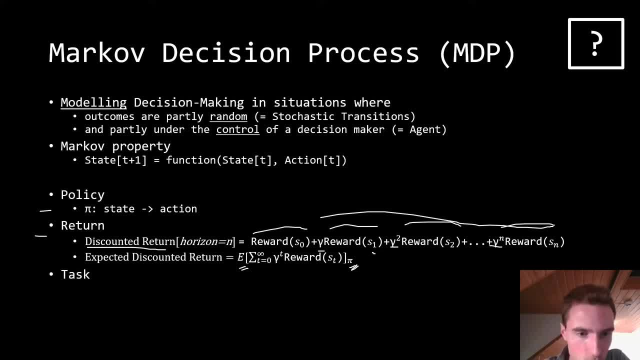 And your task. Well now, we have one quantity here That is function of a policy. In other words, We can compare pi one and pi two, The, The quantity associated to pi one Will be Okay On average I will get. 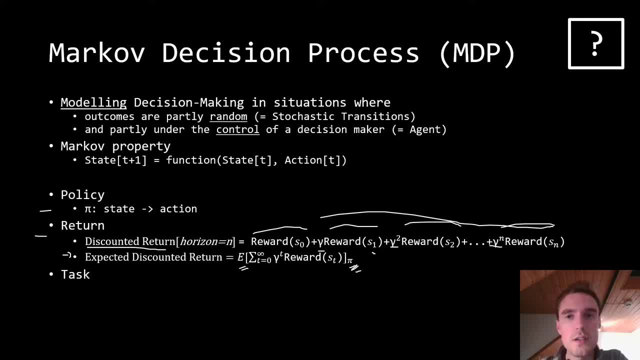 This quantity of Discounted Return, The quantity Associated to pi two, Is okay On average. If I listen to pi two, I will get This quantity. So you are now able. You have a metric, You have a. 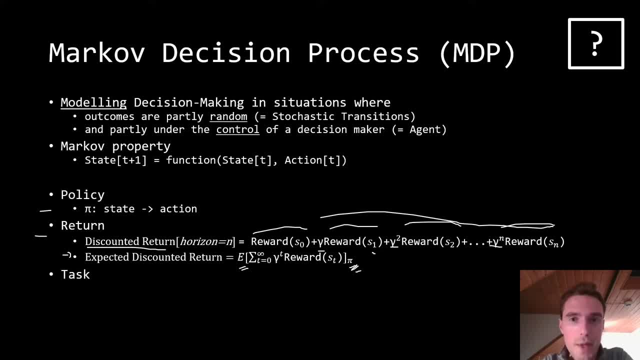 Evaluation Metric That you can use to compare pi one and pi two. So it's an operator to make This is greater or Smaller than, And this will Enable you to To make a ranking Of different Classification. 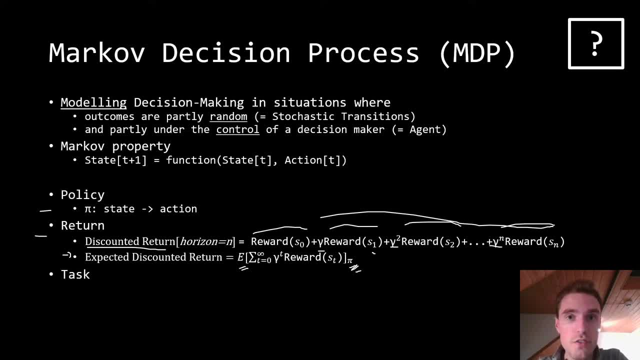 A ranking, An evaluation Of the difference, The different Policies That are possible, And solving the MDP Means finding The pi That maximize This quantity. Otherwise, Sorry To put it another way, It's finding pi. 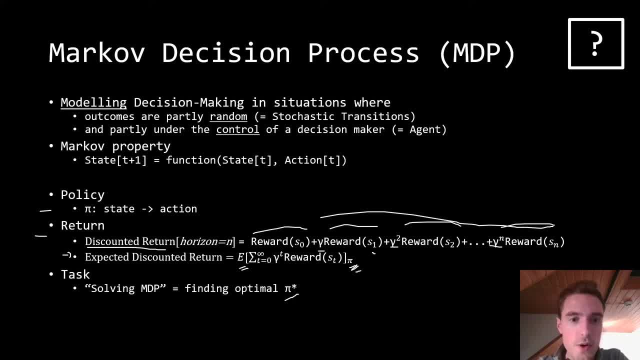 That is at the top of the ranking, If the ranking is based On this criteria. So maximizing The expected Discount In sum Of rewards Over time, Over an Horizon. Again, I've Mentioned it, If you're not familiar. 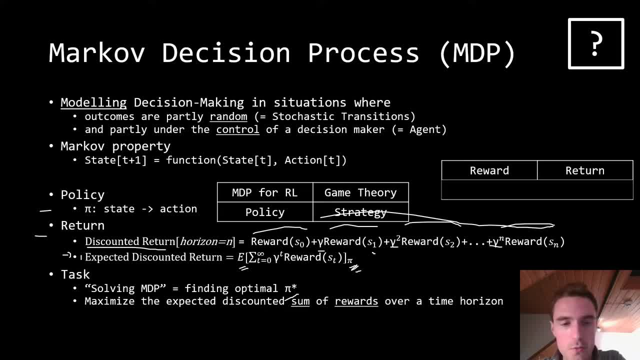 With policy. Think of it As a strategy. This comes from Game theory. Another, Maybe a Little Quiz: What is the difference Between a reward And a return? They have the same Unit, In a sense. 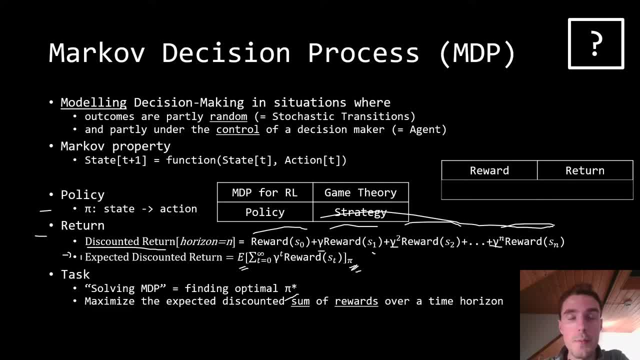 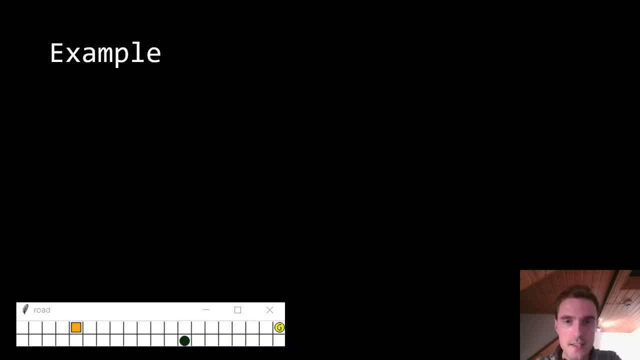 Of This is Something You collect But they don't Have the same Return Is for One Episode. That's the difference. Let's take an example To To our figures In it. So this is an. 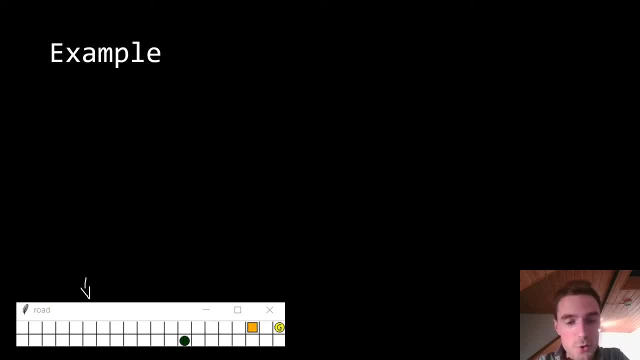 Environment I have Designed Really, Really Basic But useful For education. So we are Here At the position, At this position, And we want to go there. So think of A car Trying to drive. 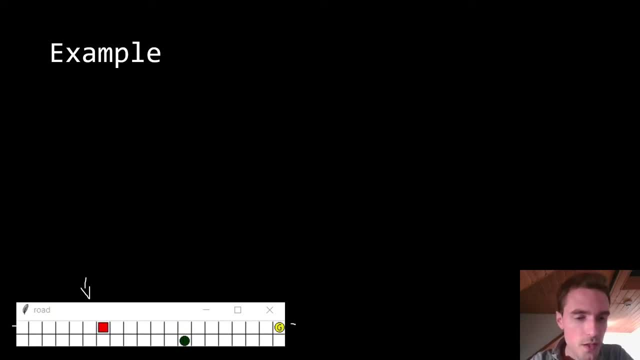 Along The road And you have To slow down Or to maintain Your velocity. The velocity Is represented With the color, And the higher The velocity, The bigger The jump Or the The step You are doing. 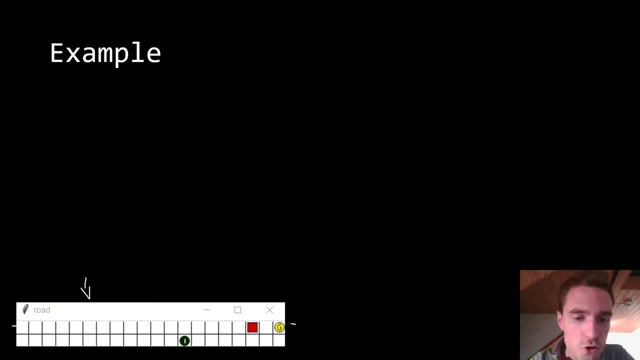 In one Time step. You have noticed There is Here A little point And Is to mention: Okay, I want you At this Part of the road To slow, To slow down, To drive Slowly. 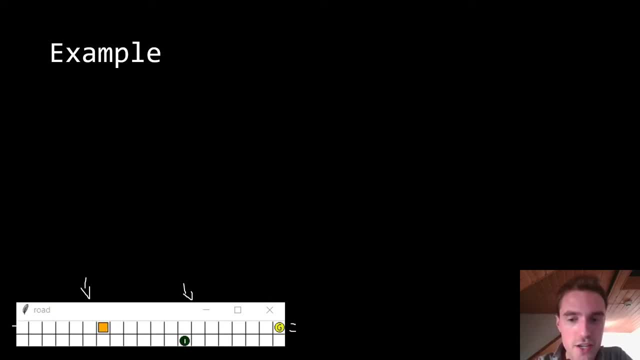 So As well. Okay, Another constraint Or another challenge. I want you to To get To this finish line With the velocity Of Three, So velocities Between zero And four I want you Exactly To have. 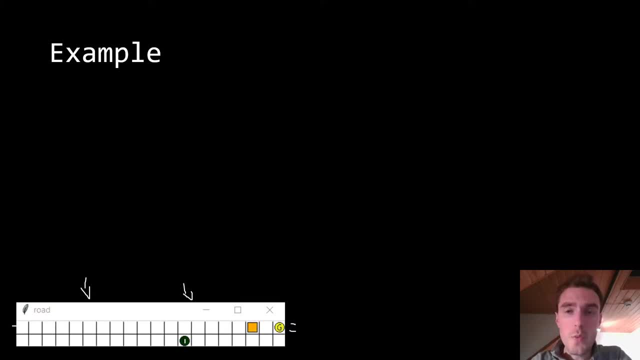 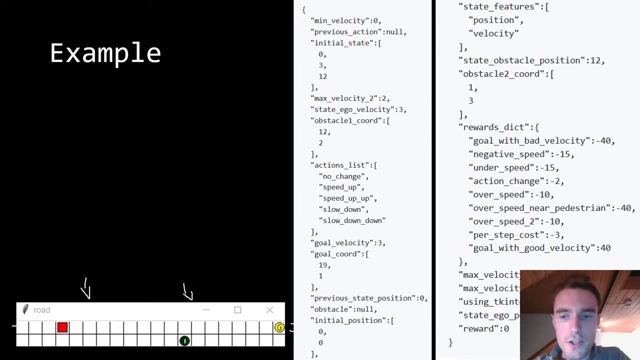 Three, I want you To go As fast As possible To the, To the Finish line, So all This Requirement Can be Encoded And Position Form Together The state So you described. 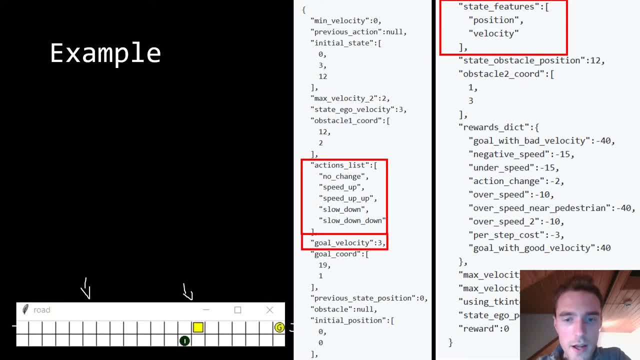 With these Two parameters: The action Possibilities About the velocity- And I want The velocity At the end To be Three Exactly- And The reward. I have Designed it Manually, You can see. 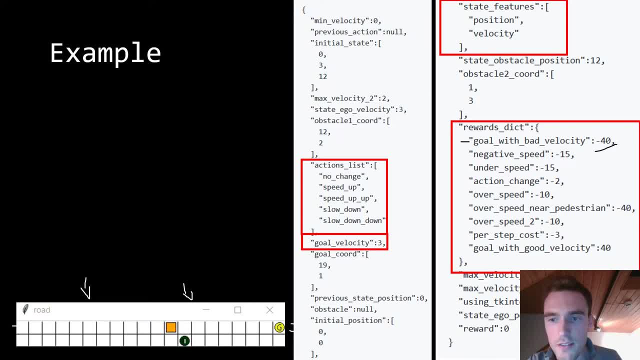 If You Reach The destination With Which With which You cross The finish line, And The same applies If you drive Too fast, Close To the pedestrian, But If you get To the 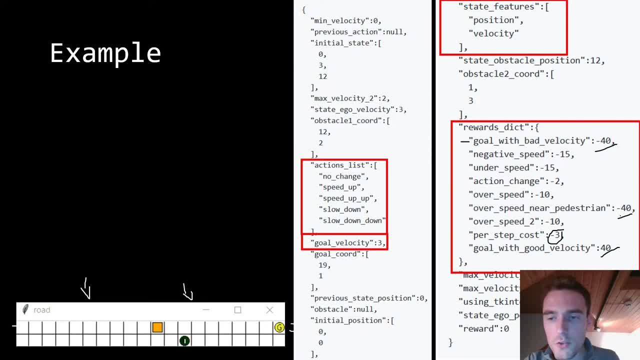 The end With the Good Velocity Is. This Parameter With A Minus Three Is Useful For Each Step And To End As Fast As Possible. The 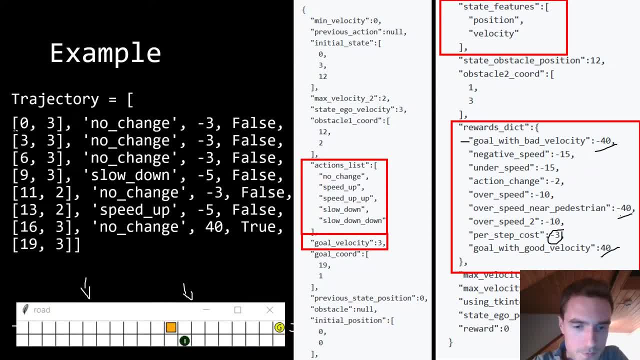 Task. Now Let's Have A Look At The Trajectory, A Possible Trajectory. You Start At This Position, So Zero Means. Position Zero Is Called. 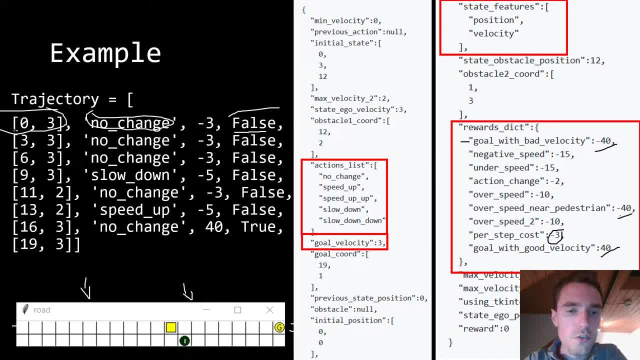 Determination Condition. Have You Reached The End? The Answer Is No, So False, Then The Next One. This Is Your Next Step From Three, Three. 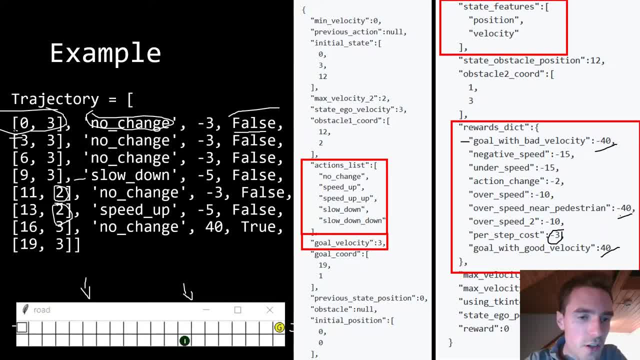 Against No, You Get To The End With Velocity Three, Which Brings Him For This Particular Step Plus Forty. And At This Point Determination. 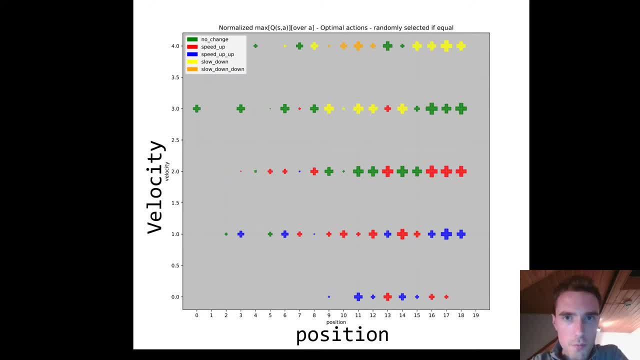 Is True. He Has Ended The Task To The Two Dimensional Figure, Because We Are Our Two Elements, The Position From One To Nineteen. 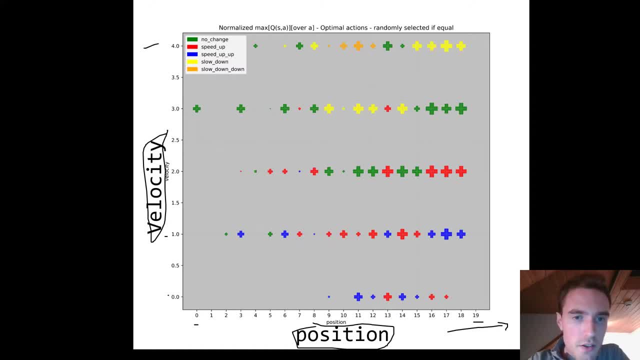 So Remember The, Remember The Straight Line And The Velocity. We Are Here, So We Read That In This Action. So In This State, The Policy. 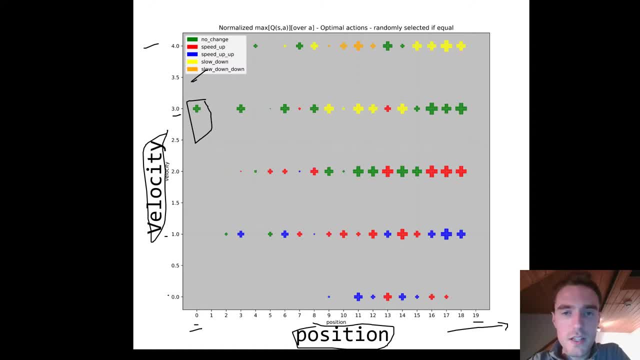 Which Is Represented Here, Is Saying: You Should Take No Change. I E You Maintain Your Service Among These Five Candidates. This Is Another Policy. 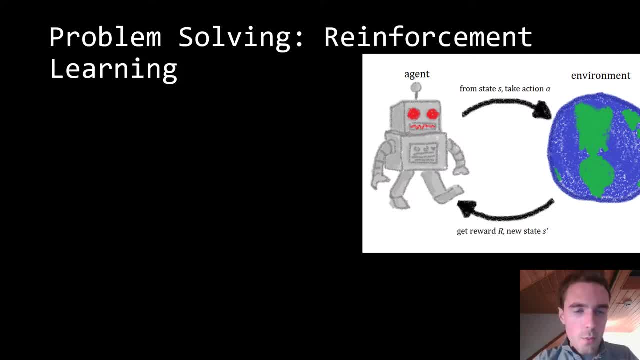 Again, Just An Example To Illustrate The Concept Of Policy Mapping States To Actions. Well Done. Now We Have Our Here, We Will Use It. 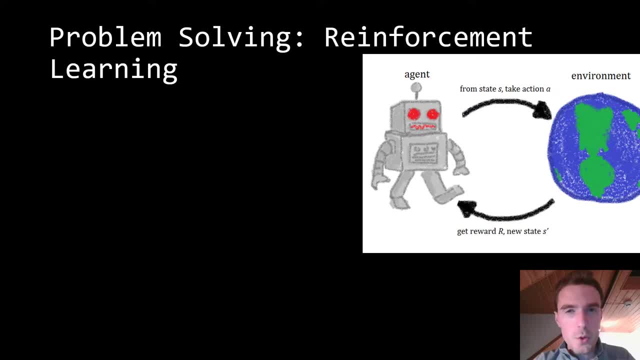 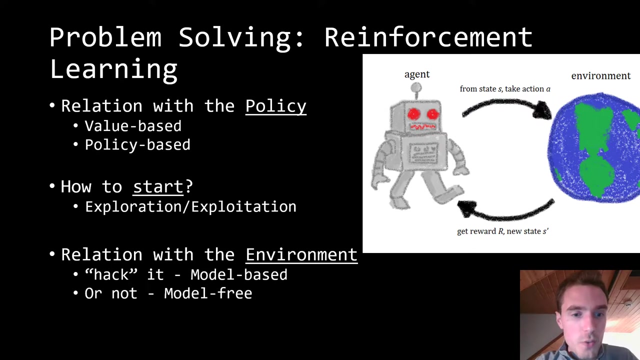 And Now We Have Three Design Choices, Or Three Design Elements. We Need To Consider The First One. Remember, We Have To Find The We Have 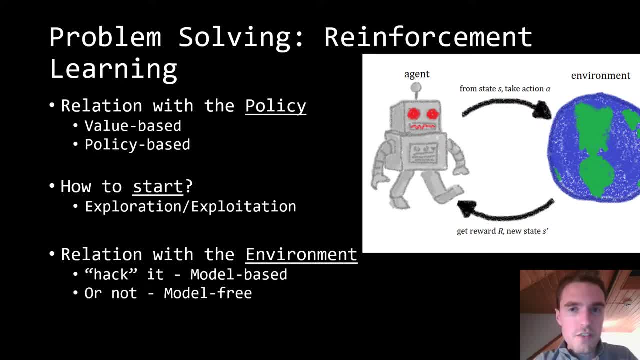 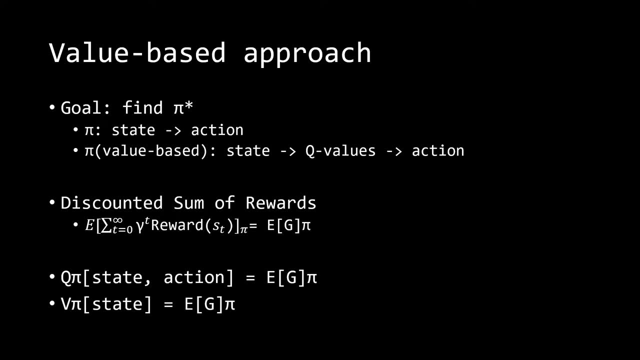 With The Environment, And Again A Distinction Between Model Based And Model Three Approaches. Let's Go For The First Task. Let's Start With Value. 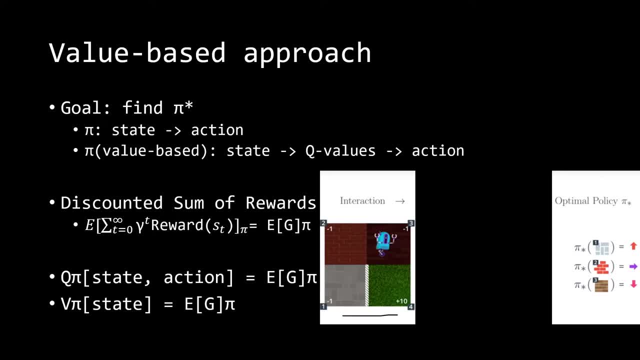 Based Approaches. Remember The Last One? Here Is Actually A Termination State, Which Means Termination Is Equal To True When We Are Here. So 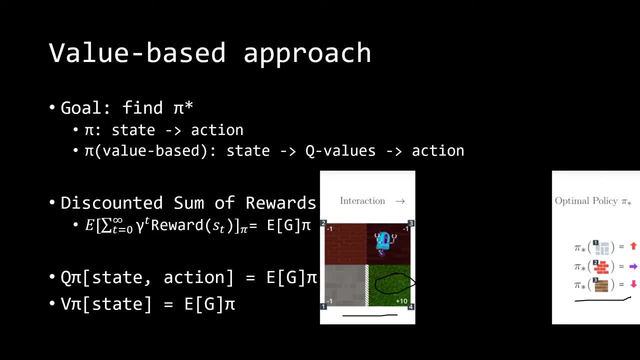 We Don't Need To Take Any Action. The One You Should Go Up, And So On. So Just An Example Again To Show What The 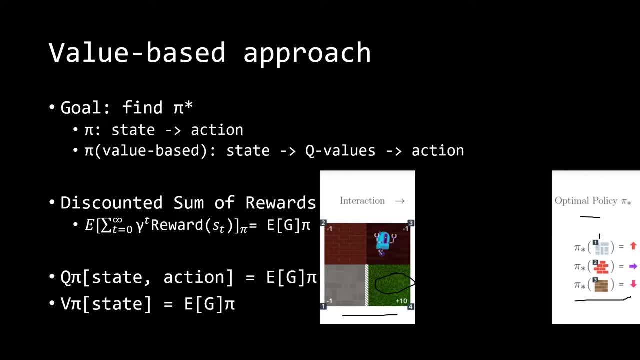 Policy Is. Remember The Task Going From Here To Here. Well, Remember The Four Possible Action That Says Us Okay, Going Up As A Value Of. 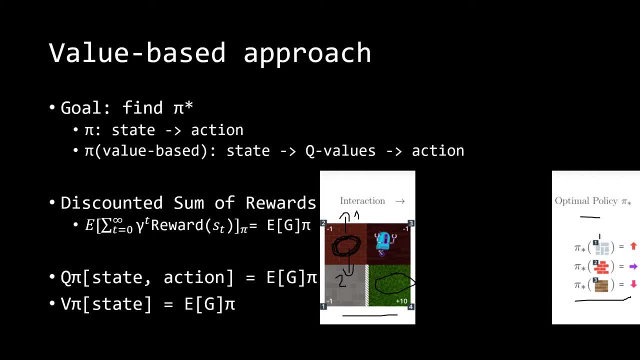 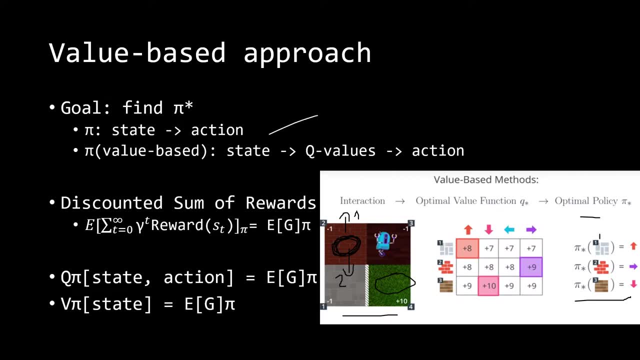 I Don't Know One Going Down As A Value Of Two And So On. It Pass To What Is Called Q Values And Q Values. 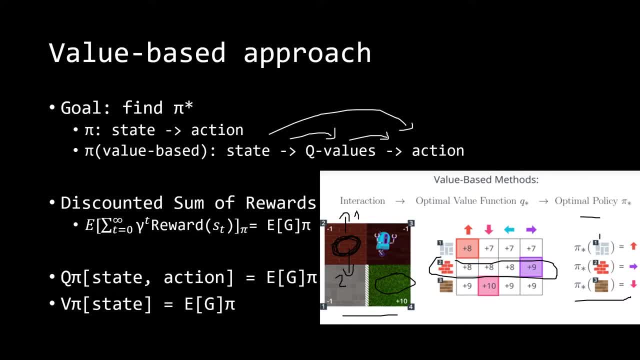 Are Represented In This Table. So Again, We Are In This State And This Table Collects For Each Of The State. Well, And The New. 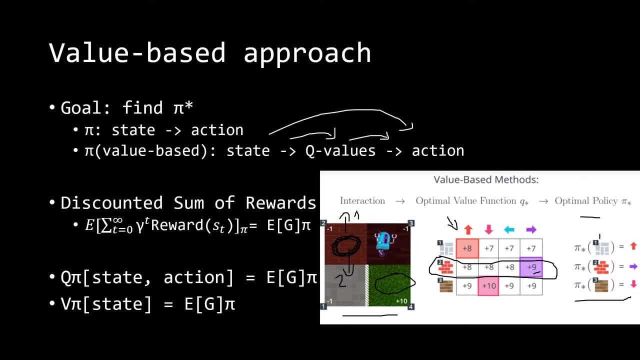 Task Is To To Complete Or To Determine Or To Fill This Table. This Is A New Task Once We Have Done It, Once We Have. 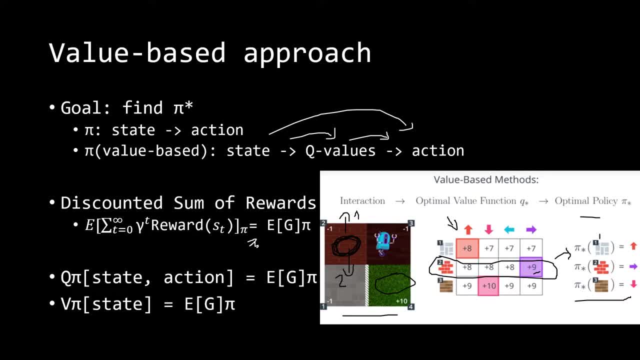 Done This And This Is A Very Important To All The Activity Of The Action And It Represents Again The Quality Of Taking This Action, Being 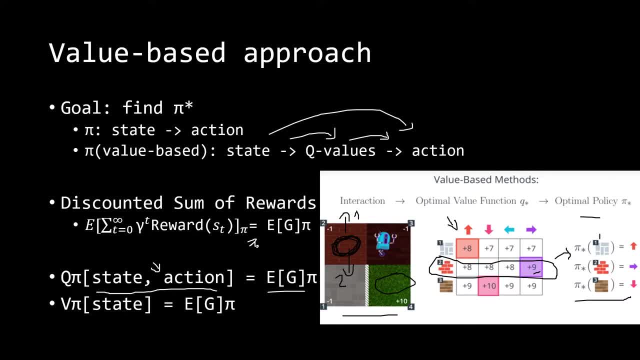 In That State And Mathematically It Represents The Expectation You Have If You Take This Action- Being In That State- And Then Follow The 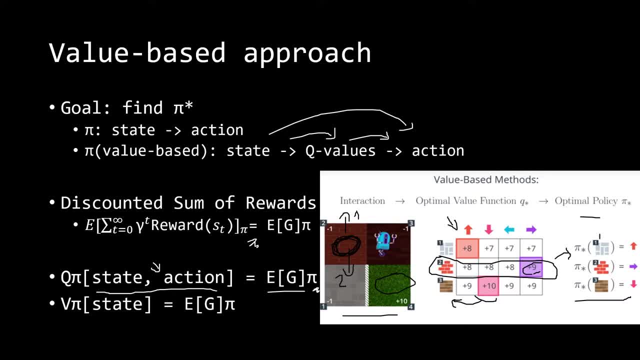 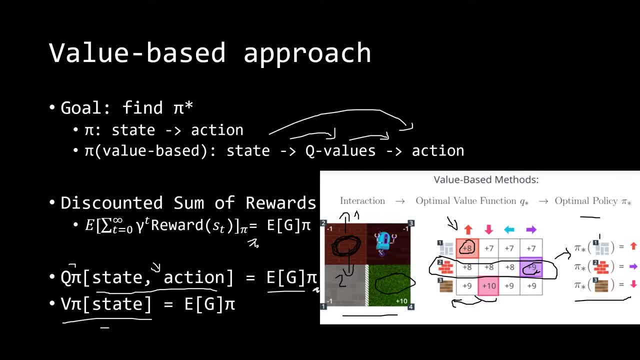 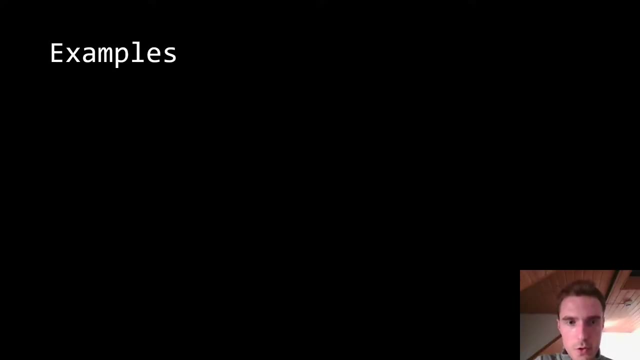 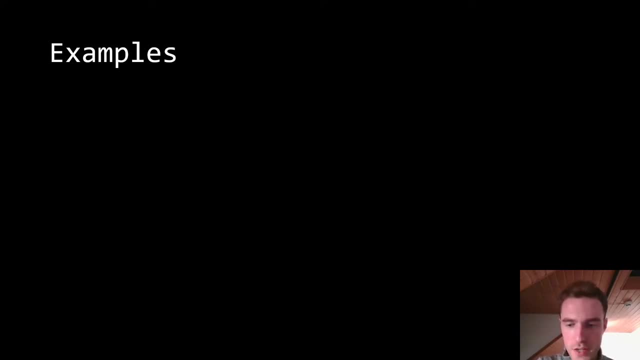 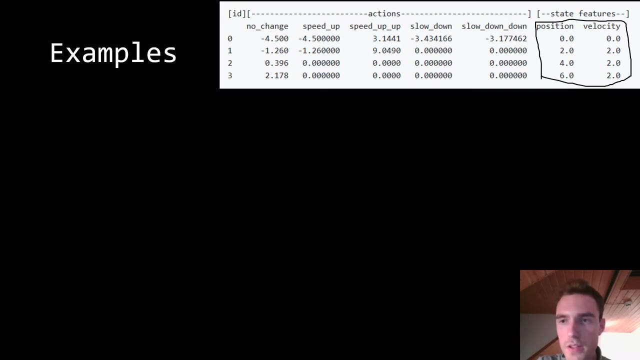 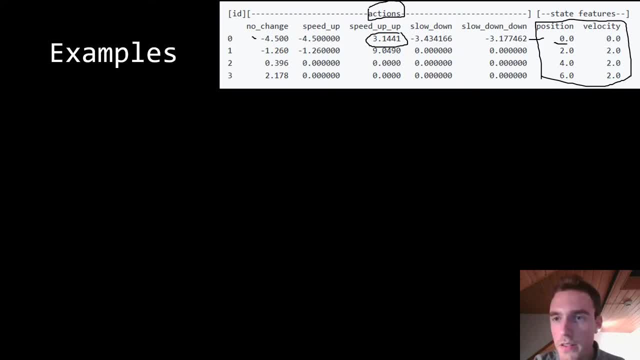 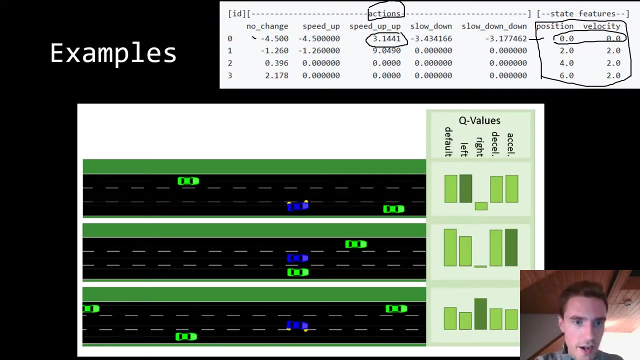 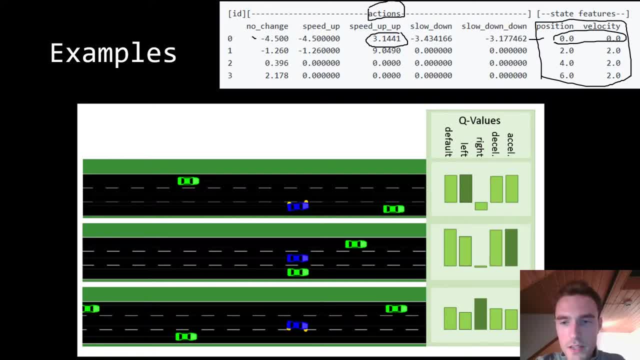 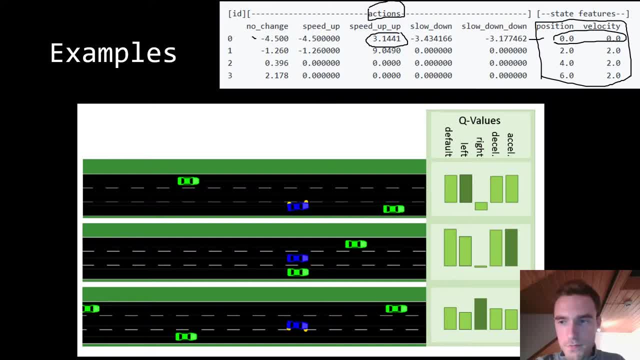 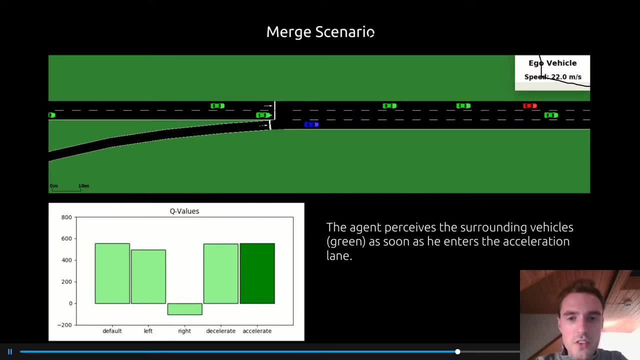 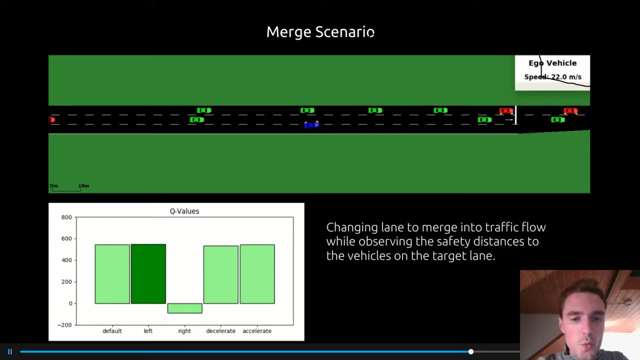 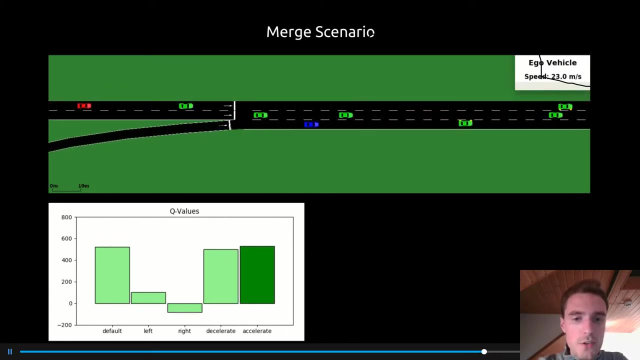 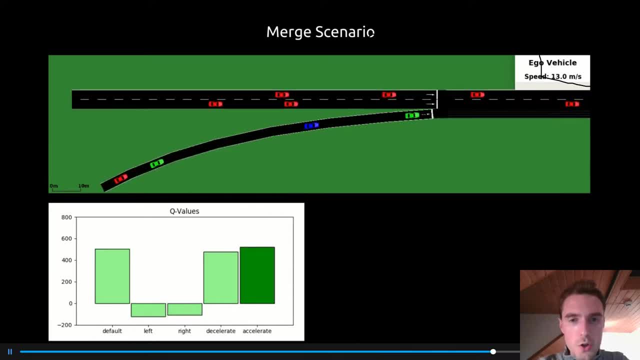 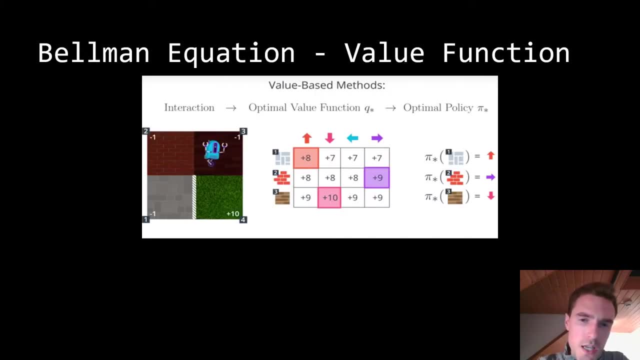 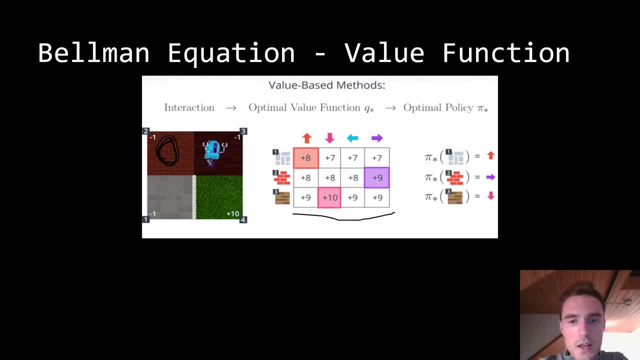 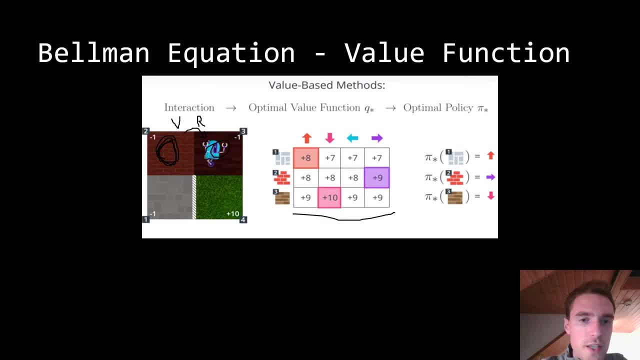 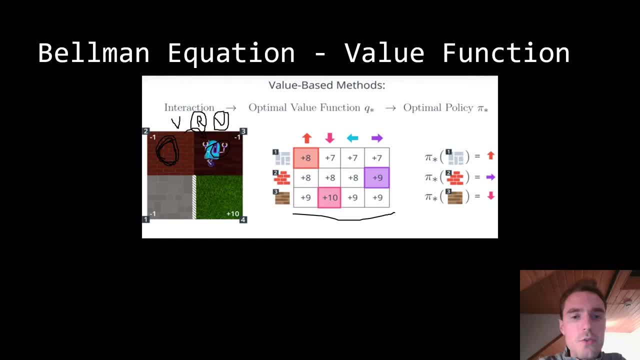 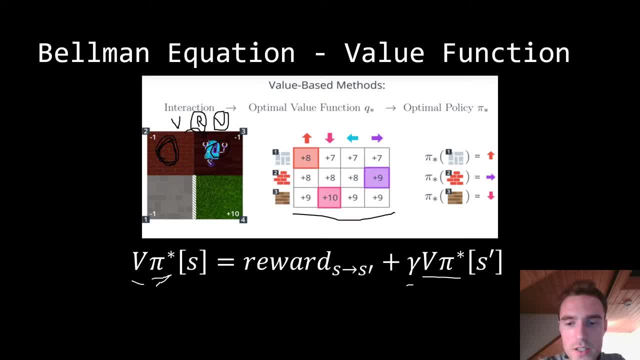 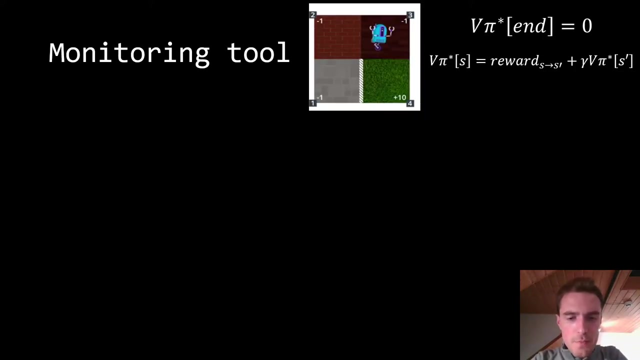 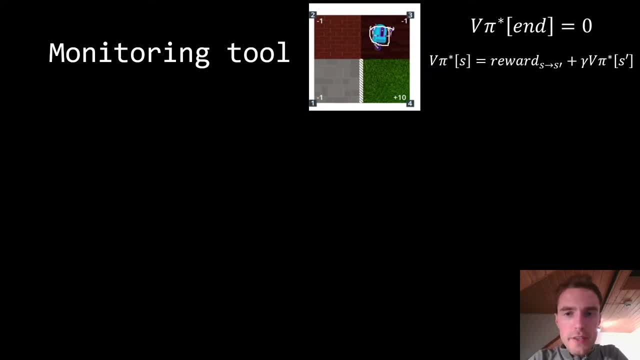 Let's say now we are in this state, so we are just about to terminate. We have the possibility to terminate if we go down. You may ask, if I apply the Bellman equation, what should I take for the value of the termination state? The answer: we take the convention of value. 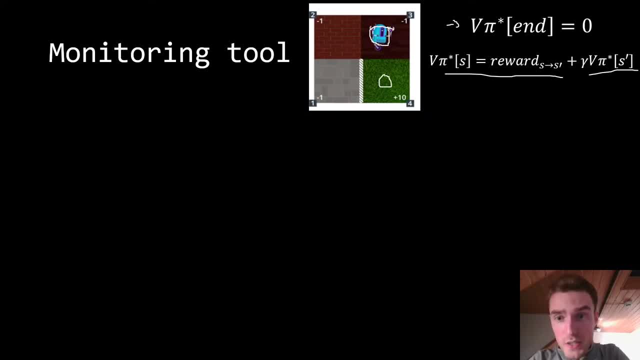 is equal to zero because it's terminated. Well, but what happens then? to this part We only have the value of here is equal to the reward associated to this transition. That's it. We don't have to look for an estimate of the next value, And that's a really powerful property. 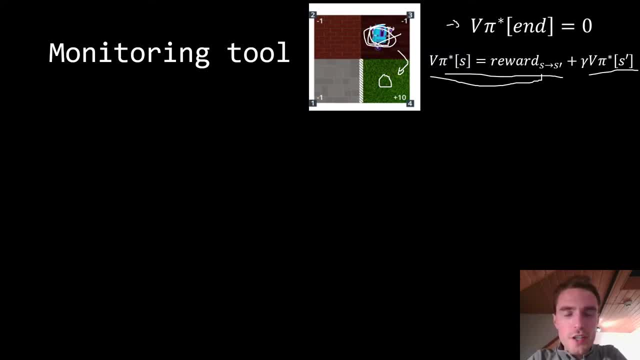 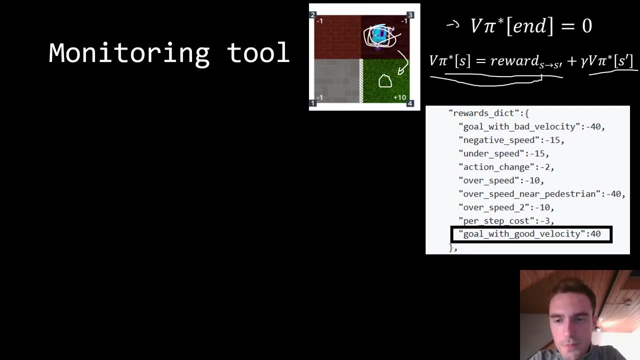 You can use it to monitor the evolution of your learning phase. I explain why. So here we have the structure of the reward for the simple road environment. Remember that if we get to the final state, the finish line, with the correct velocity, we get plus. 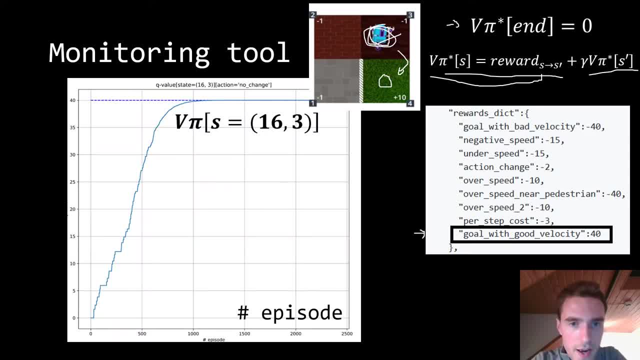 40. In other sense, For this particular state, position 16,, velocity 3, we are able, if we take the right action, which is the maintaining velocity, to get to 19,, which is the terminated state, the finish line. So we are, in this case, we are about to finish and we know that for the optimal, 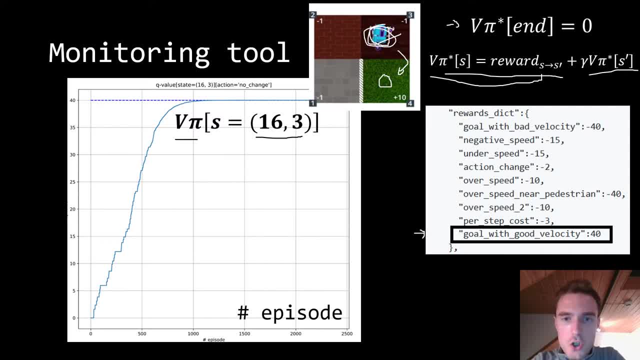 policy. the value associated to that should be 40.. In other sense, we can monitor the evolution over the training process. So these are the number, the idea of the episode we are training on And we plot the evolution and we can in real time during training process. 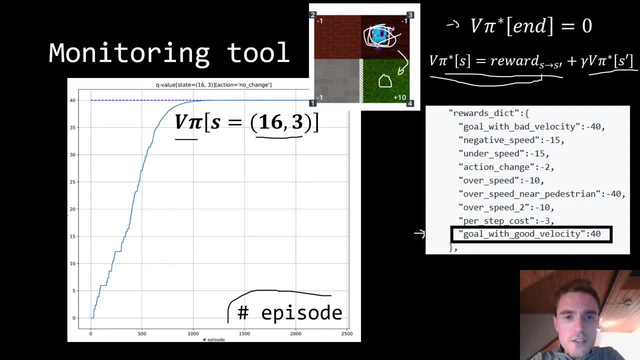 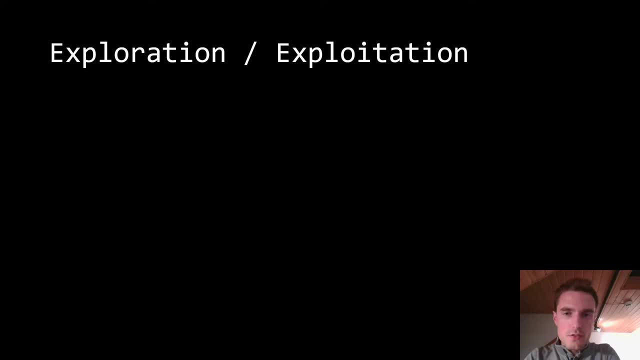 have a look. Does it converge to a value first, And does it converge to the expected value? If not, then there is something wrong. So quite powerful tool to monitor the evolution of learning. Okay, Time now for exploration. Exploration versus exploitation trade-off- It's really really close to the intuition. 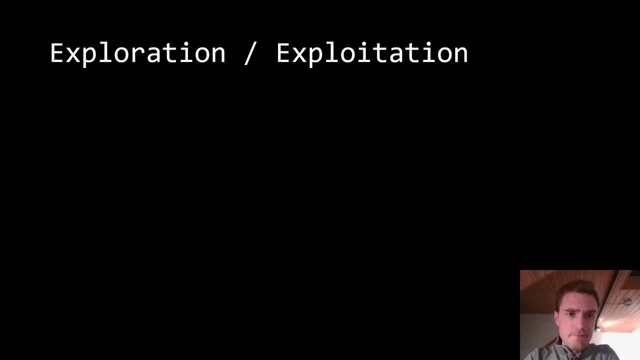 of human behavior, what we are doing in life. Especially, let's take the example. You have moved to a new city. You know no one, nowhere, no place. You want to go to the hairdresser, So you will pick one randomly. This is exploration. Then it might be not satisfying, So you just. 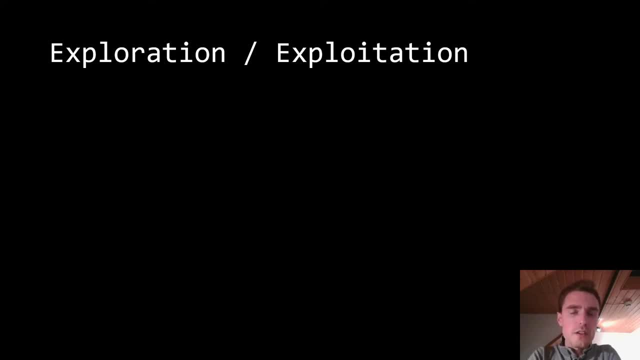 move to another one again randomly or with a high stochasticity, And so on. This is exploration. Now consider your situation today. It has been a couple of months. You just continually go to the same hairdresser. No room for randomness. It's about exploitation And this concept. 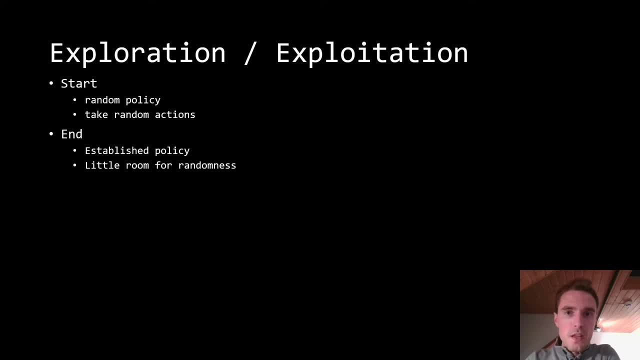 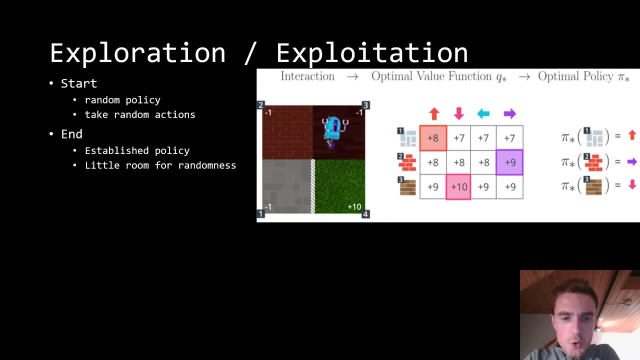 is used for reinforcement, learning, And especially when acting with the policy. Let's take an example: You have to fill this table And then, from this table, you take your actions. The question is, what or how is it structured? How, from this table, I can? 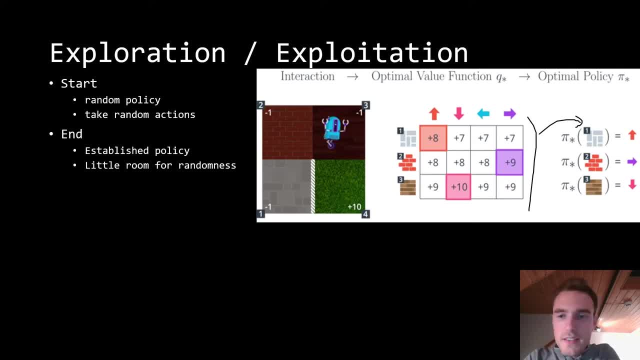 take the action We have said at the end. if we are really confident in having consistent values here, it's just enough to take the max. So that will be done here At the end. we take the max. So no room or little room for randomness. 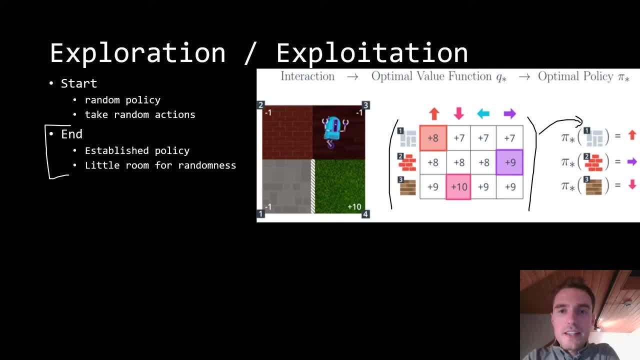 But at the start, consider that this table has been initialized to its random values. So that may be instead of 8, OK, this is the best one, But that may be the worst one. So minus 2,, then plus 2,, plus 1,, plus 10, and so on, Randomly initialized. 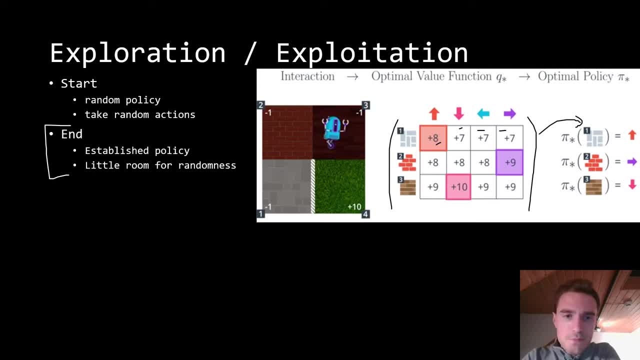 So you don't want to consider the values first, because they have no robustness or no consistency. What you really want to do at start is take a random action among all the possible candidates. So this is done at here, at the start. 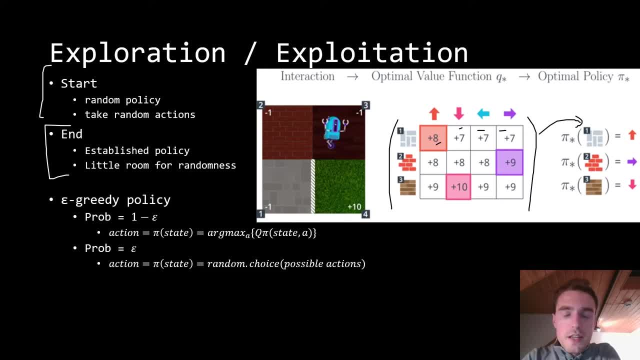 How do you do this? How do you do that? Well, introducing epsilon parameter, which is a float between 0 and 1.. And you see, I consider 1 minus epsilon And with this probability, I use the best candidate. So the best candidate here will be 8.. Here is 9 and here is 10.. So I use up. 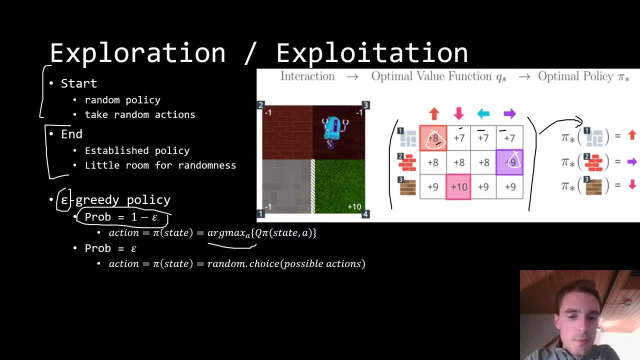 and then right and then down, But with the probability of epsilon. I don't do argmarks, I actually don't consider the values that are in this table, I just randomly select one of these. Now let's take an example. if I say to you that epsilon is equal to 1. 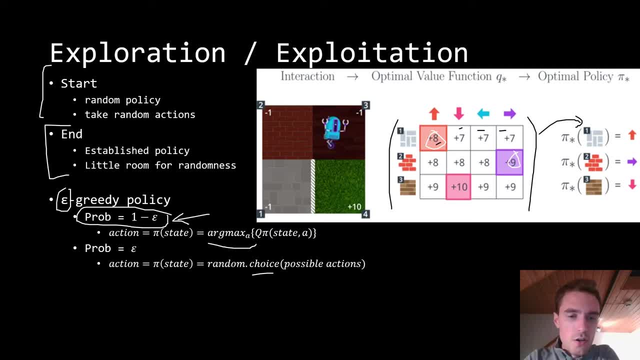 That means that this probability is null. so we don't listen to this case, we go for this one. So if epsilon is equal to 1, we act randomly, but purely random, only random. On the opposite, if epsilon is equal to 0, then there is no room for randomness. 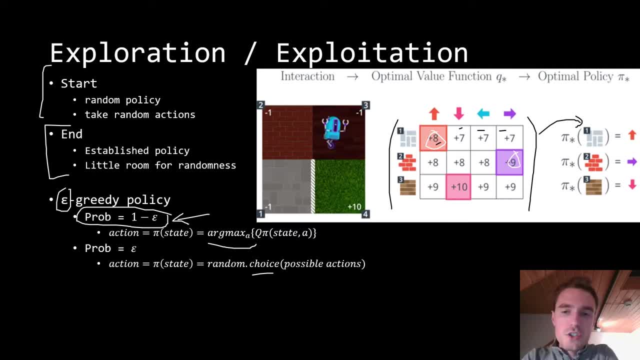 We just take the argmarks, So you just apply argmarks, We just take the best, the corresponding action to the best, to the highest Q value. Now the question is: we should start from something close to 1 and then go to something. 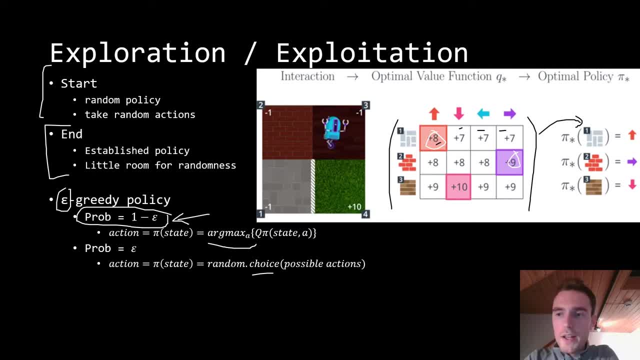 close to 0.. How do we process? We have to shuttle the decrease of this parameter. This is done by having an additional variable. So we have to have an additional variable. So we have to have an additional variable. So we have to have an additional variable. for epsilon, let's say 0.9999 or even 1.. 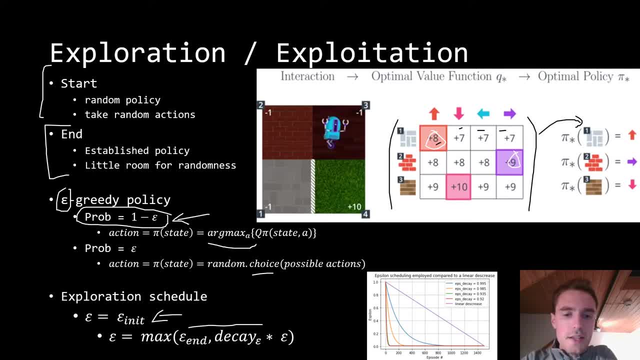 And then we decay it, decaying by multiplying. at each episode We update epsilon by multiplication with a decay parameter which might be okay: 0.9999.. So it will go a little bit, it would get a little bit decayed, and so on and so on, until 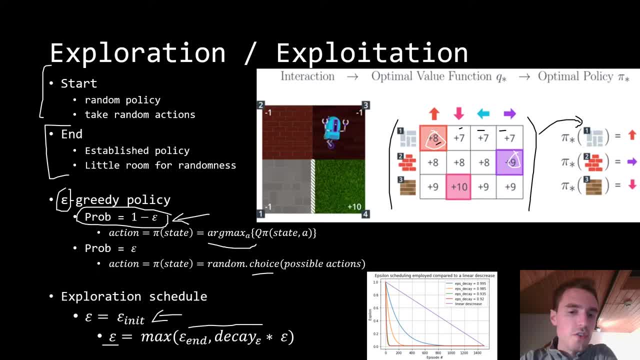 reaching 0 or let's say, 0.001.. Two comments. The first comment is from experience. This decay parameter is really really important, or at least has a lot of impact, has a huge impact in terms of performance, So don't neglect it when you are doing your hyperparameter tuning. 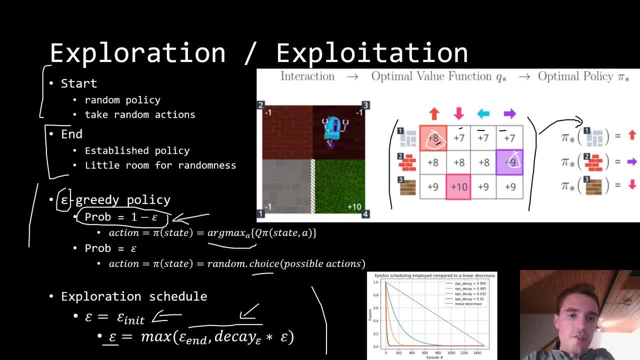 Second comment is that this idea of epsilon greedy policy, this idea of how do I go from my Q table To the definition of the policy, This idea is really really, really commonly used. It's everywhere, So most algorithms use it. really simple, but really powerful. 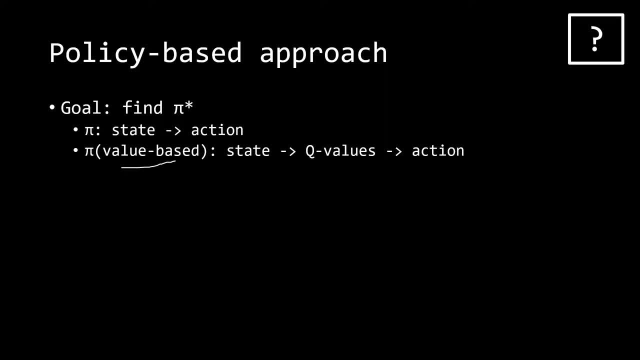 So so far we have seen the value based methods that introduce the Q value in order to go from state to action. There is the possibility to go directly from state to action. This is known as policy based. I have no time, or I don't have time yet, to cover this topic, but just mentioning three. 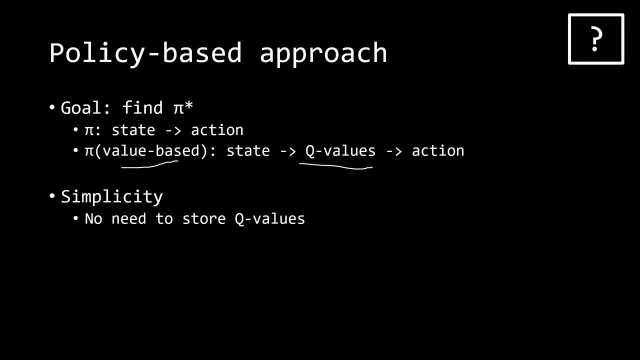 strengths It has. first one: There is kind of simplicity because you don't need to store these Q values. The second one is it enables you to define stochastic policies. Stochastic policies means this was not a stochastic policy because it was value based for each. 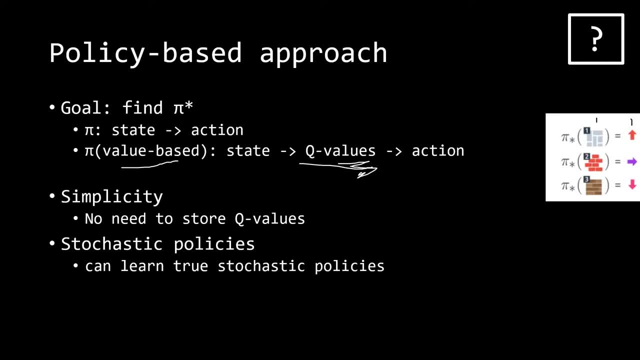 state You can't say. if you are in this state, then I would recommend you to randomly decide between go up and go left. This is not possible. You have to be strict and say there is only one option: Go there, But for some particular problems. this is good to have this stochasticity. think of this. 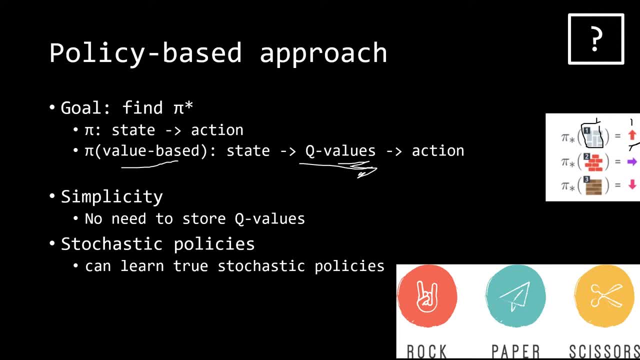 game. in game theory, It can be showed that the best order, The optimal strategy, consists in choosing randomly between the three of them. This is not possible with value based. This is possible with policy based. It says you: one third, one third, one third. 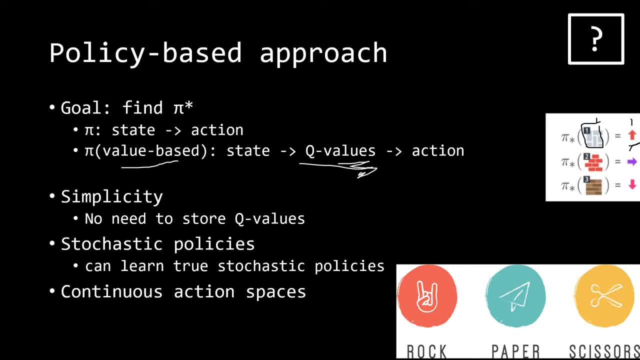 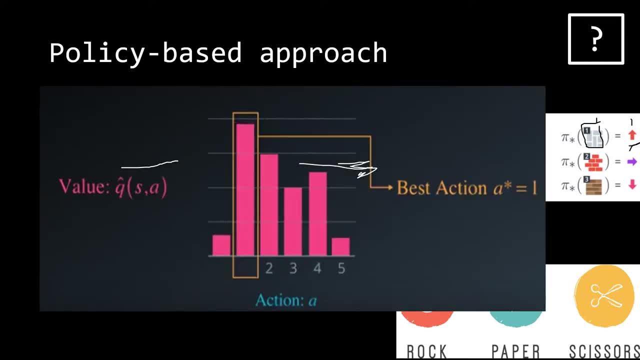 And the last big advantage is that you can cover more easily continuous action space. Remember we had this case of, For instance, driving, Driving the on the highway. Should I go left, go right, slow down and speed up, and so on. 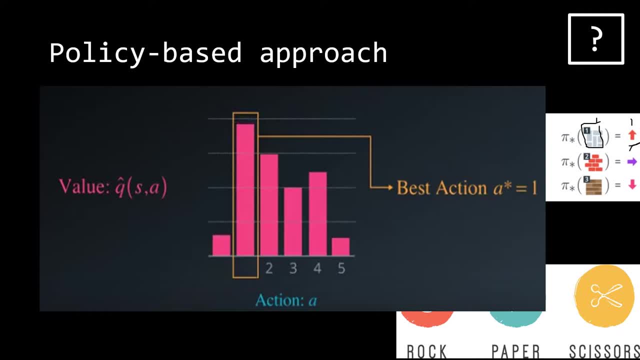 And for each of them we have a Q value. Then we were selecting the best one, the highest one. This was the argmax operation. This is feasible for discrete state space, but it becomes quite tricky to do with continuous space. You can think, for instance, this might be: 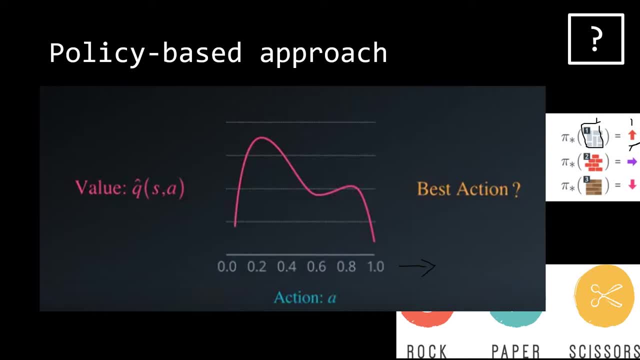 The, The level of acceleration or, let's say, the steering angle you have to make. and to find the optimal point, you have to put some optimist to implement some optimization which is not tribal or at least which is computationally demanding, Which is not the case with the policy based approach, because you don't have Q values. 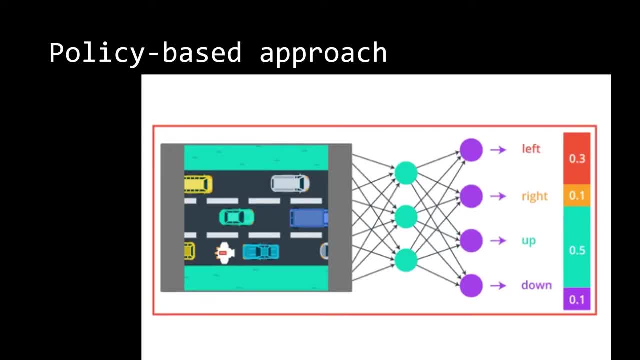 A quick word very quickly about how do you learn in a policy based approaches? So again, this is your State. An example here is a. You defined a picture with pixels, The pixels are processed and at the output You have for each value, 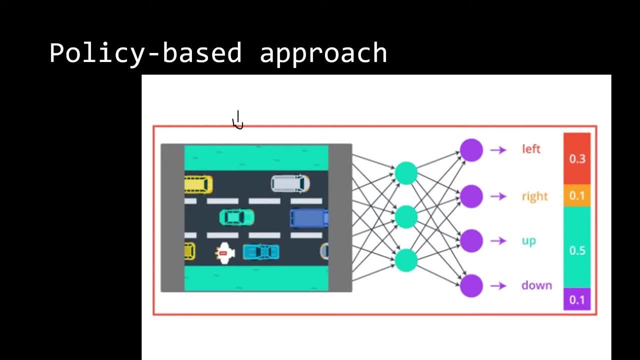 Sorry for each action It recommends you to take. left with probability One third up is the Is the most likely one. You should have it for the time. So this is one policy when doing policy based approach, One result. So that's it. 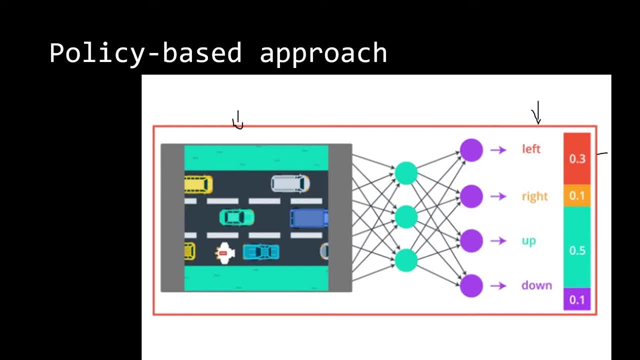 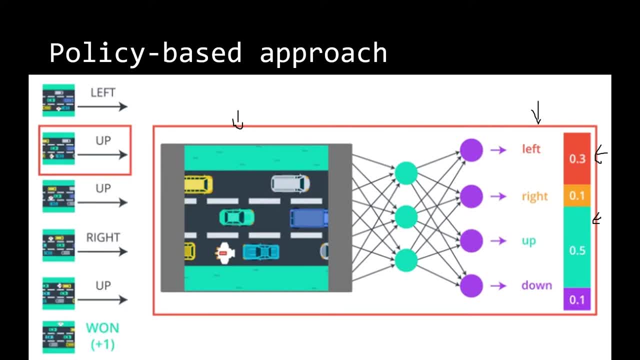 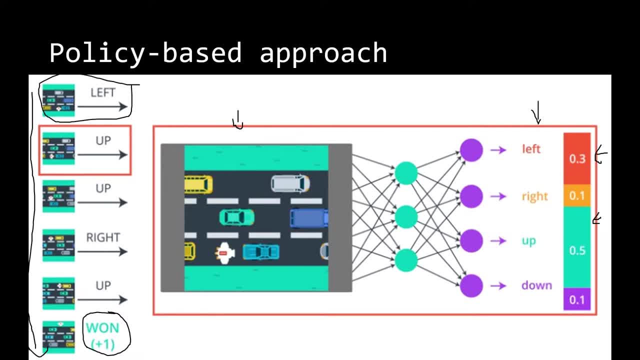 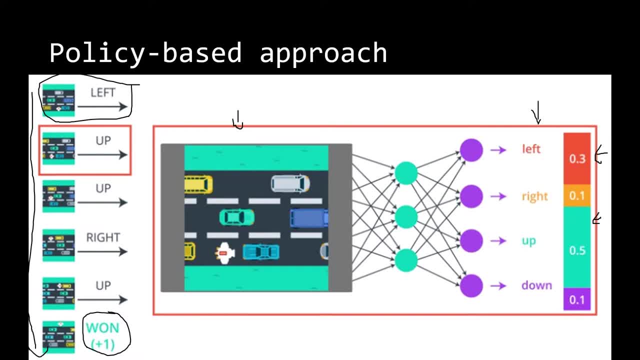 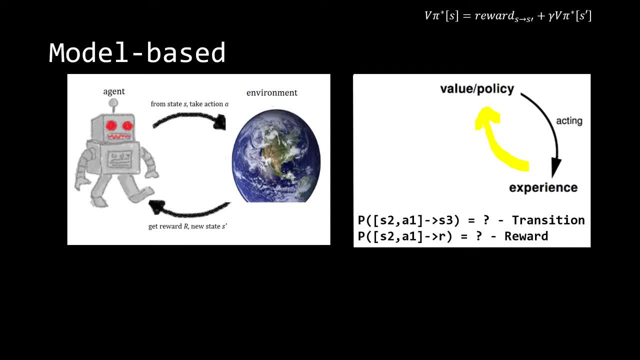 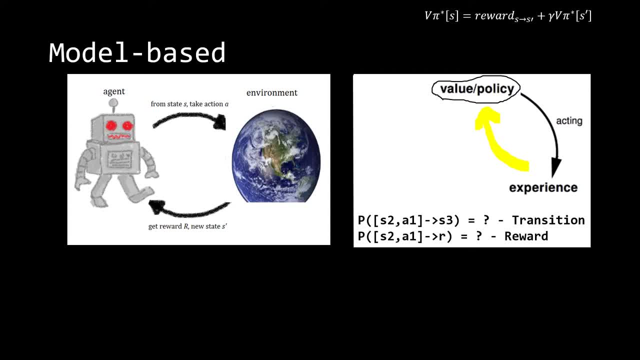 we are experiencing, in order to improve this value and policy. another thing to to note is that the transition function, how you are taken from s and a to s prime. this function is only known by the environment and the same applies for the revolt. in other words, if i say in you, you are in. 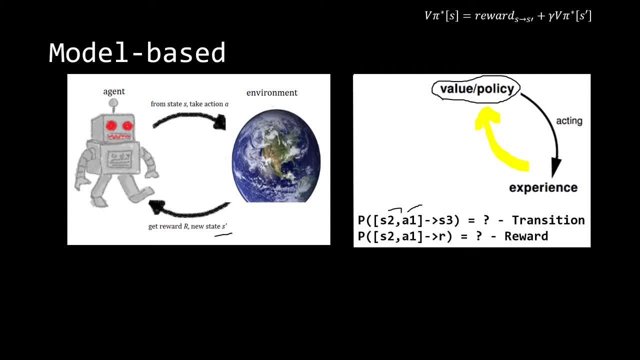 s2. let's say you are at 20 kilometers, you want to speed up. what's the probability of getting to 30 kilometers? actually, you don't know. you have no idea of this transition function. and, in the same way, you are taking from s to s prime. you are taking from s to s prime. 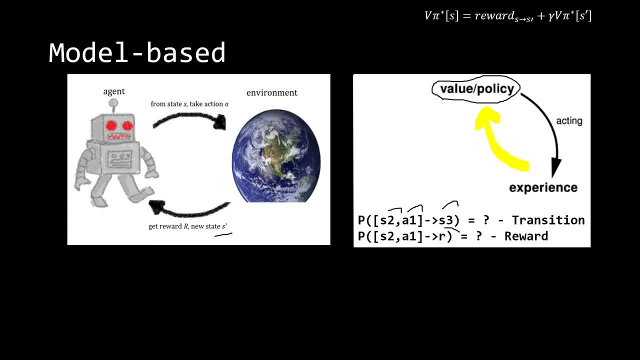 vain. what's the probability of getting plus one? you have no idea. this is only from the knowledge of the environment. nevertheless, once you are doing, or when you are doing, this step, you are collecting information about s, a, s, prime and r. so this is one temple, one experience we have. 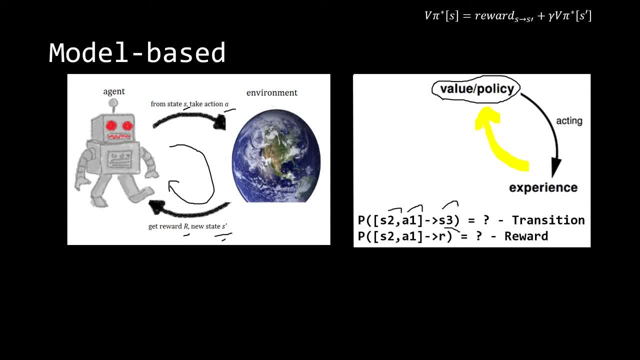 already said, you are using it to update your model, your q values, for instance, to improve your policy, and the idea is: why not using this tuple to try to model these two functions? why not observing? okay, i was at 20, i asked to ask, i'm now at 30. so i might have the feeling when i asked to speed up, then i should my velocity. 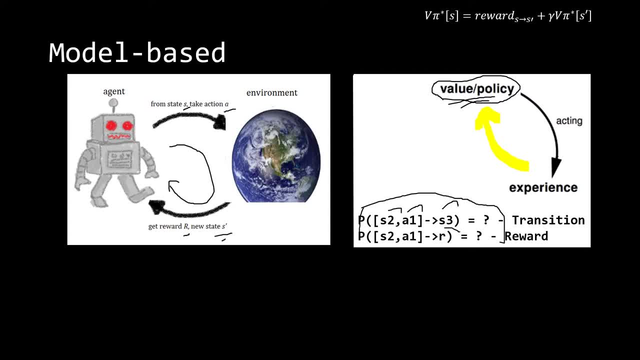 should increase, and so on. this is the idea behind model based. what you want to do is to have two tasks when experiencing one step. the first one is to gain in quality with respect to is the return, and to gain with knowledge- knowledge how the model evolves at the 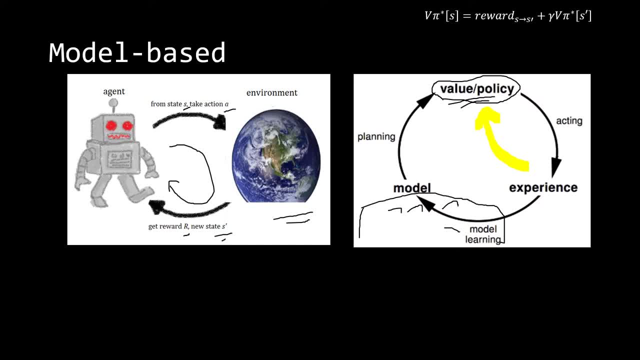 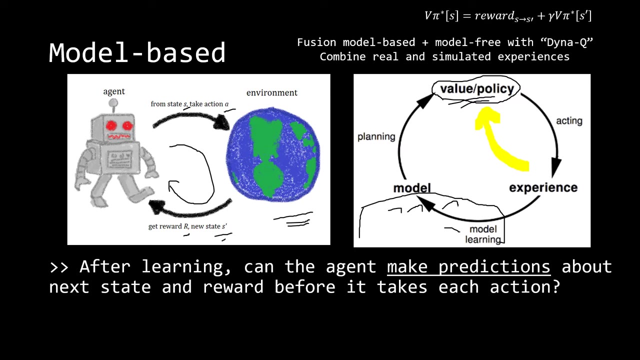 end of the day, what you want to do. this is quite extreme, but is to disrupt, to remove the need for an environment and replace substitute with a model of this environment. so when, when developing your, your solution, you can ask yourself: after learning, can the agent makes make a prediction about the next state and the next? 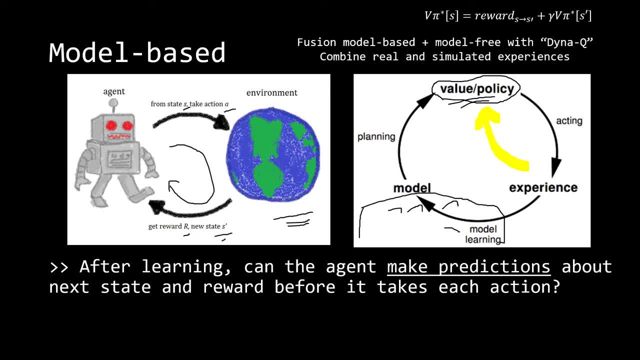 reward or the report before it takes each action. if yes, then it is the case of model based. if no, it is called model free. all right, let's say, now we have done model based, we are no need now to get um a direction with the environment, since we can predict. i can predict that. 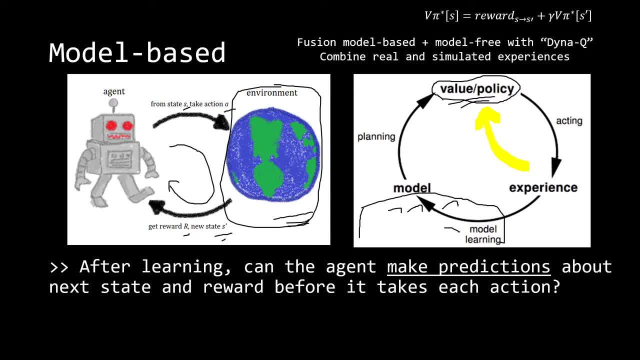 if i am at 30 and i want to speed up, i will be at 40 next time. if we are in this case, then we don't need the environment and the problems comes. in solving the mdp, finding the optimal policy, what you can use is what is called dynamic programming. there are policy iteration or value iteration. did 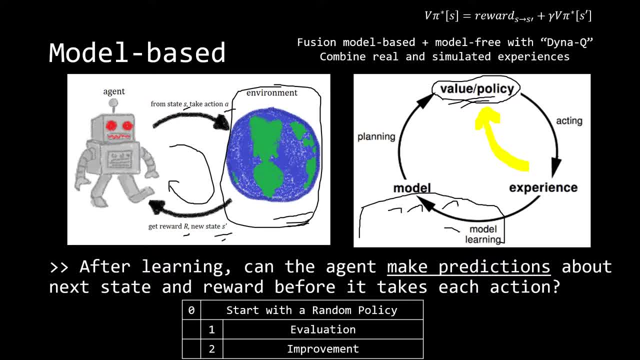 really, really quickly. you start with a random policy. you want, at the end, to have the optimal one, but you start with the random policy, then you evaluate it, and then you evaluate it and then you assess it. um, yeah, assess the quality and then improve it. and then you do that, you iterate. 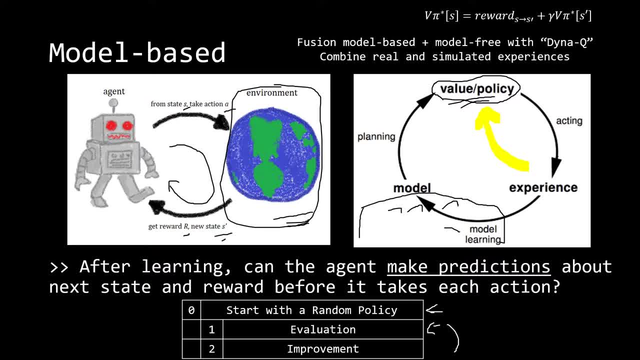 until you converge, you are converging and this is important. you have no interaction with the environment, since you have a model of it. this is the idea: model based versus model free. okay, back to results. here are some results. one is for model based, the other one is for model free. 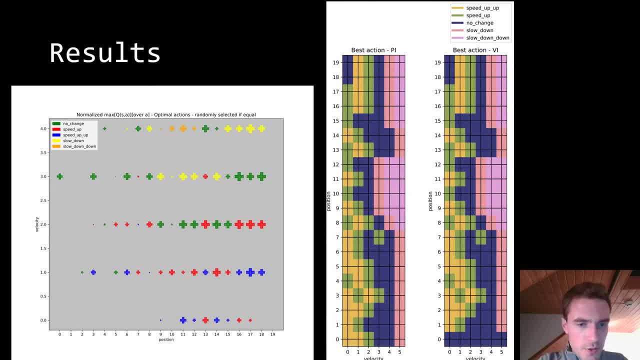 so, having a first look, what differs, you notice? they both represent the policy you have to implement here. however, you don't have any decision. or yeah, the policy says, i don't know. so this is model free, because with model free, you didn't have the opportunity to explore it. you just rely all what you are saying, all the um, the policy. 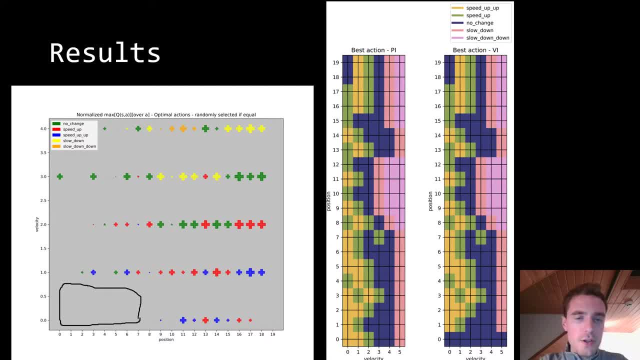 domain is based on what you could experience and in this case, since we are always starting with velocity three at position zero, we are always starting with velocity three at position zero. we never had the opportunity to explore this region, so we can't say this was good or this was. 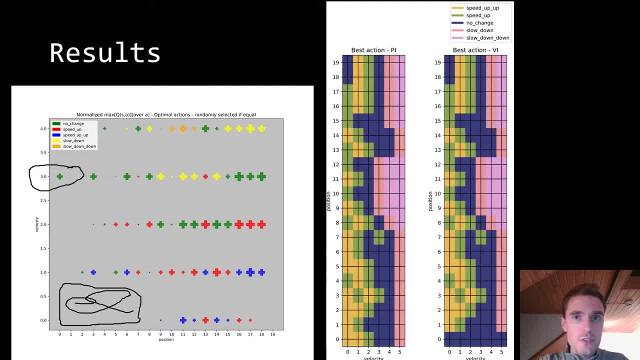 bad, or in this case you should take this one or this one, or at least not with a tabular representation. with function approximation is possible, but not with tabular representation. that's model free. on the other hand, here we have also a representation of the policy, the position, the velocity here, and so for every model three you have to take a position. 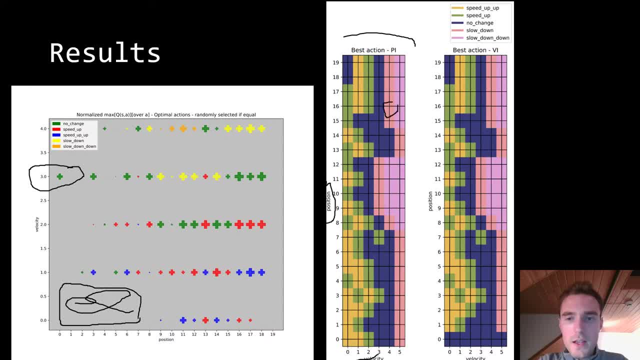 so for each position it is one state and for each position you have one color. then refer to the color code here to know which action you should take. so again, these two figures represent a policy, describes the policy. the difference is that this one was made with policy iteration. 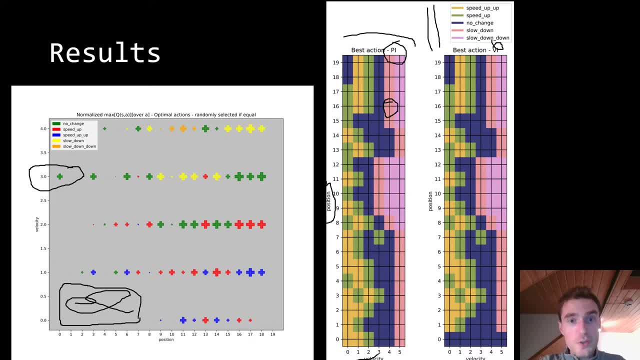 the other one with value iteration, just to illustrate the concept of model based versus model three. model based: you have the full knowledge, so you know. if you are speeding up when being in position zero, you will do that. so you can fill the part at the at the bottom of the. 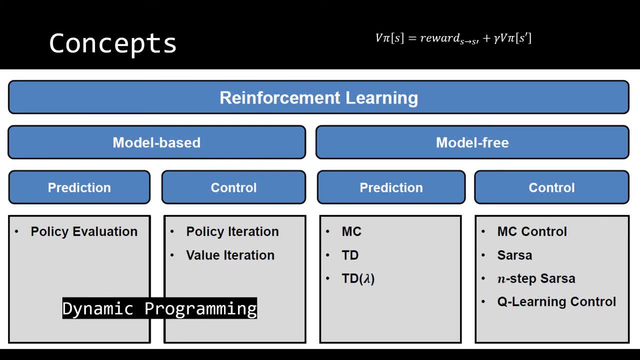 of the plot. okay, just to sum up, reinforcement learning can be divided. we have seen in model based versus model free approaches, and what is control versus prediction? control is exactly what we have been busy with, ie trying to find which action should be taken in one state. on the other end, prediction is about 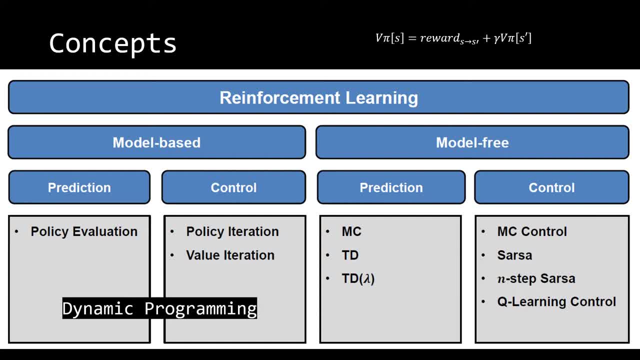 trying for each state to find what is the value of this state. this is another question: determining the action you have to take, the optimal action, or determining trying to assess, evaluate, how good is this state? we have quickly mentioned the dynamic programming for model base. i've been implementing this policy. 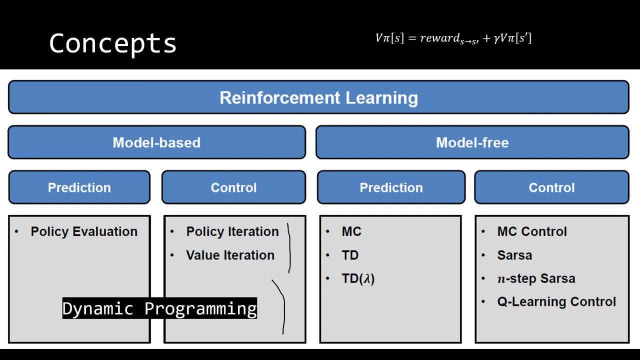 from Sesame Hill in 2017, we began again. theseatch feels rather now 8 and 8.1. now Rolle of the production system. basedAKEU is the usual method that says that in the case of model three, we have a change of value with a arising of Qus. then 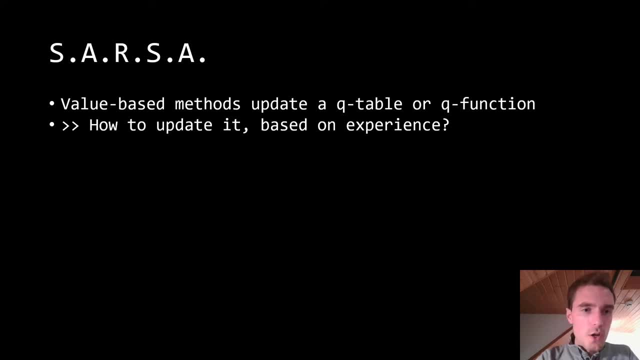 we turned to системаa positions ver gen and foroured Monk, that is, the westbound versus the northern edge position. remind you, take the usual value, one we are providing a respecto to 1000 in this system. Sansa means, or where does it come from? you might have identified s is for the first state you are. 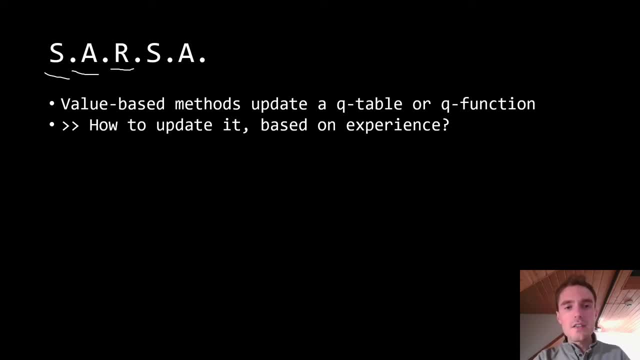 in: a is the action you are taking and r is the, the revolt. this leads to another, another state, which can be s prime, for instance, and being in s prime, you can, i don't know, take action a1 based on the same policy, but at least the first. the first one has been experienced. now the question is: you know, 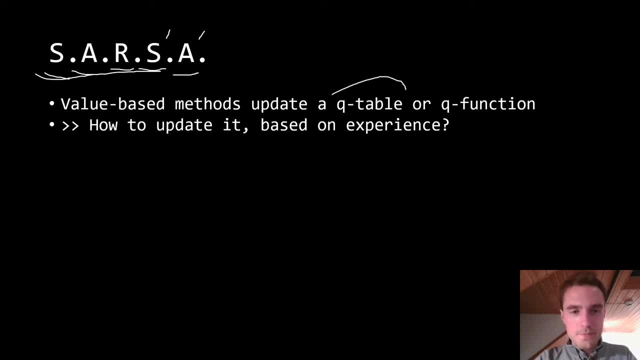 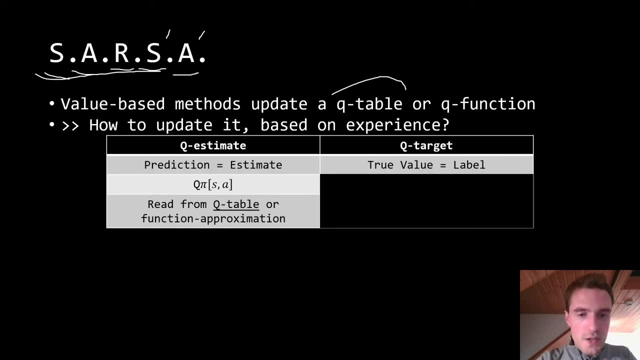 for value based, you have to update your q table. how do you update it? this is not so obvious. in particular, you have been reading in your table this value because you were said: okay, you are in state s so for action a, you read this value. now the question is: how do i update it? 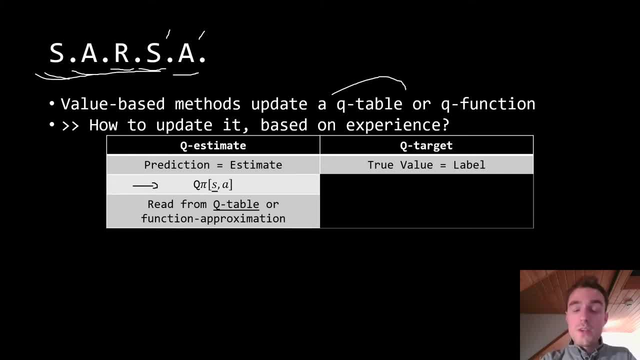 should i make it bigger or smaller? what would be really nice would be to have the ground truth, ie the, the correct value or the value of s a for s a, but this time with pi prime, the optimal policy. but this is of course not available, otherwise we will already know the. 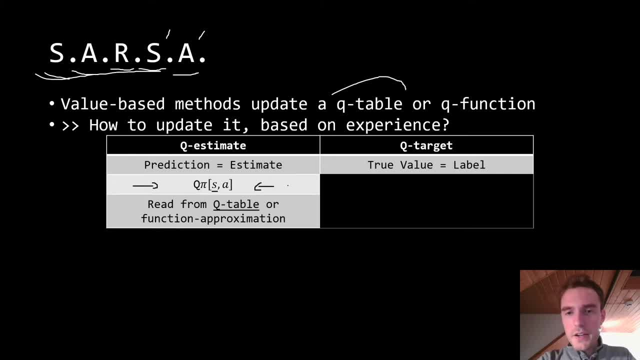 the optimal policy. so you have to fix one target or one value you aim at and then compare your current estimate to that target. but how do you get a target? one solution would be to use this optimal equation where behrman equation says: for the, at least in the 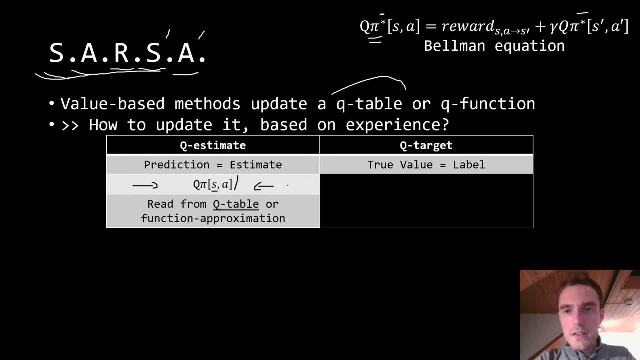 optimal case, when the policy is optimal, then this relation holds. so what you want to do is use your s prime. you have been observing, take an action, another one, a prime. so this is for the neighbor state, the new state, and compute for the initial one. for the initial state, action pair a q value. this q value will be your target. so you have now. 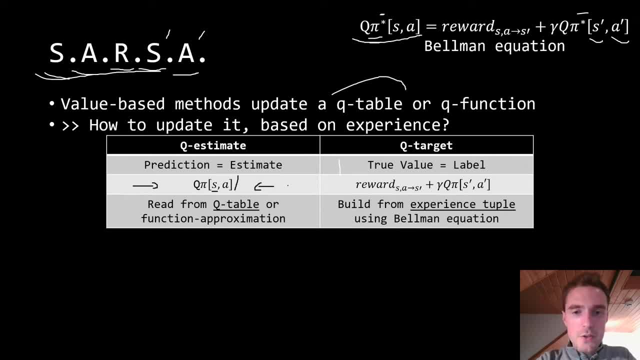 a q target on the right and you can compare now your q estimate to this q target and then this is exactly similar to what supervised learning is, where you have a label or a ground truth, you have an estimate. this is the the current model is doing is giving you. you compute the error, the difference between two, you apply a learning. 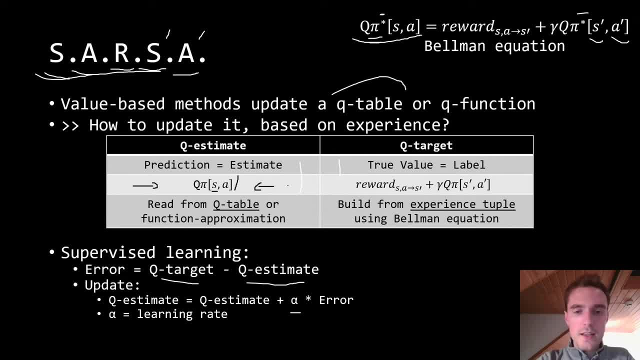 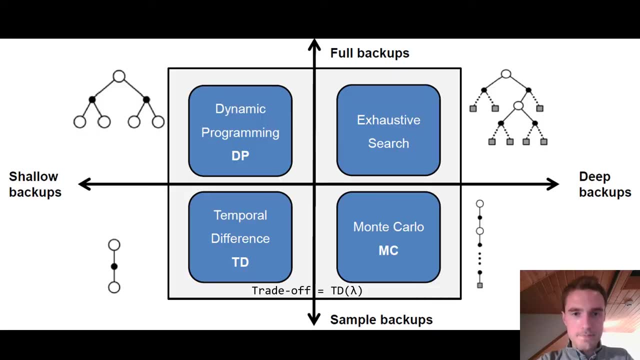 rate, to update your q estimate, and so on and so on. so for each experience s a r s s prime, you apply it and you update the corresponding cell in your table. in your table, this was the. this is the idea of salsa, so salsa is represented here. 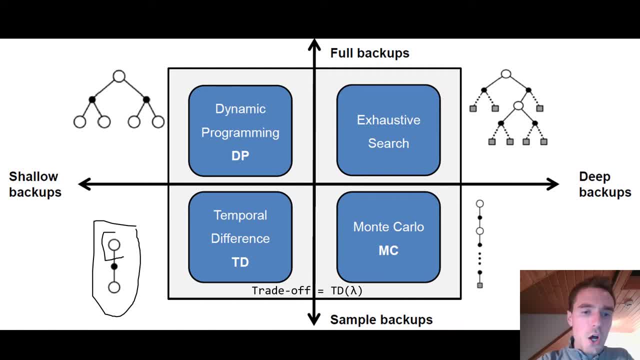 the question in this slide is: how do i update the q value associated to to this state? this represents a state. this represents also a state. the next one and the little black points represent the action that has been taken to transition from one to another and what salsa says. so salsa belongs to the family of temporal difference. 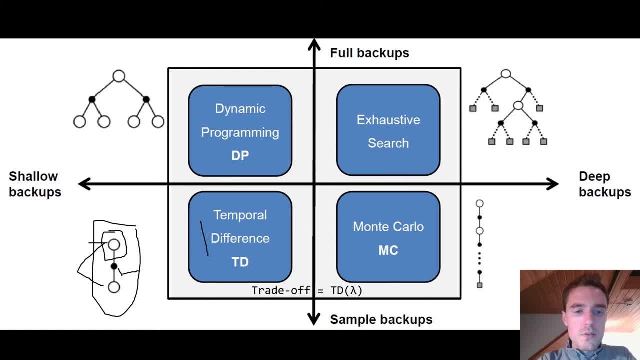 salsa is saying you, you just take this step in order to update this value. on the other hand, the monte carlo method says you want to update this value, or at least the value associated to uh, to this action state pair. what you need to do, or what you should do, is wait for the termination of the episode. 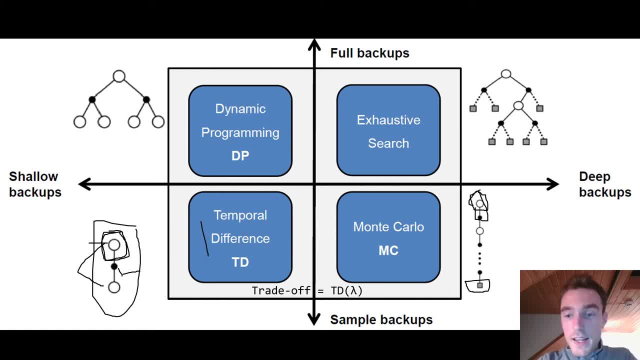 in, go, for instance, if you are, if you have lost a win, and then roll back all the information up to this point and accordingly update this. so the advantage of that is that is easy. so the advantage of that is that is easy. so the advantage of that is that is easy. 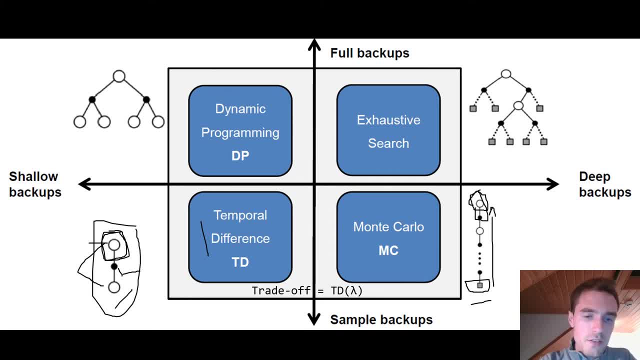 unbiased the because here it's biased. you are building your q targets based on estimation, but this is not ground truth. here you are really waiting for the end. you will get a reward at the end, you can compute the return and so on. so this is not biased, but this suffers for from. 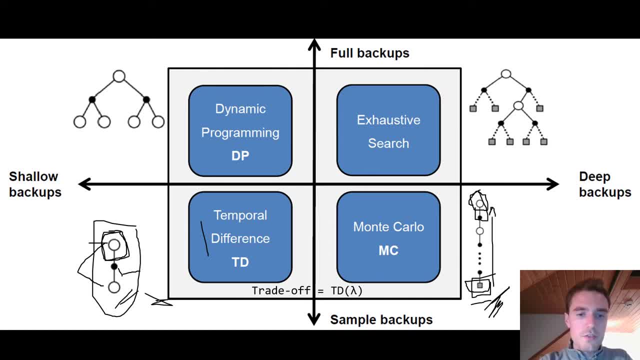 i variance, which is not the case for the, the methods, so there are some trade-offs to to have. what you could do if you have the transition model or model based, is again, in order to assess this value, you can imagine or predict, since you have a model, what happens if i go there. then i will. 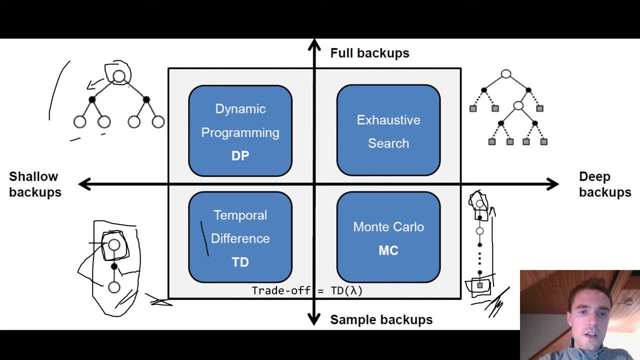 go there and so on, but again only doing one step here from here. on the other hand, this is, let's say, brute force, or if you have all the information, or if you can afford it from a computational point of view, you could do this. we could explore everything and expand each branch until the termination state. so this is the 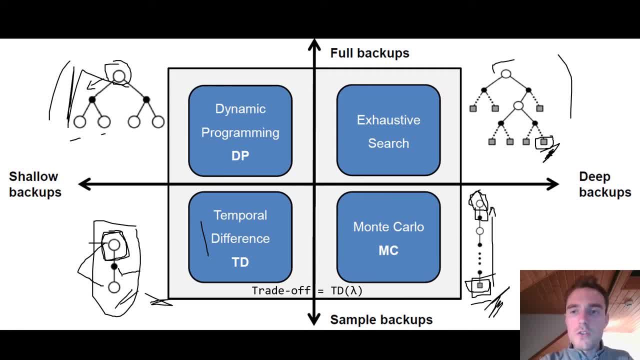 termination state and then roll back the information again. the goal of this slide was to know how do i update the value corresponding to this state. so this is a very short overview of what is possible for updating the value of one state. okay, let's see, maybe in particular how 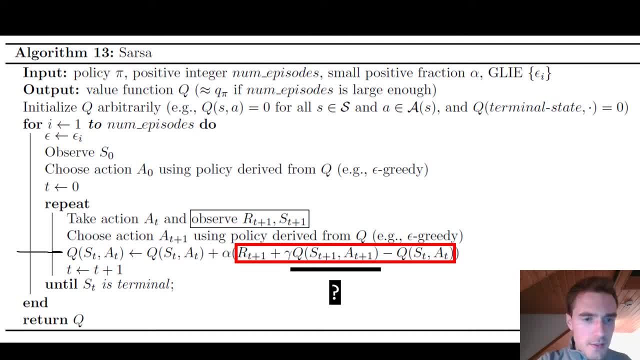 sasa works, and just consider this line, this one where we are updating our estimate of the values. so we have been experiencing one step. we saw that we went from s and a. we observed r prime- sorry, t plus one and s plus one, st plus one. now the question is: how do i update the, my estimate? 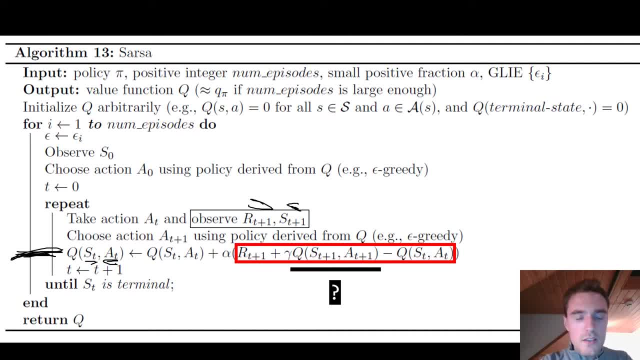 about qsa. well, what we have seen is you compute the error, this is the red, the red term, and then in the arrow you have the difference between the target and the estimate. so the estimate is here and the target is the first term, and inside the target we have the reward that we have just seen. 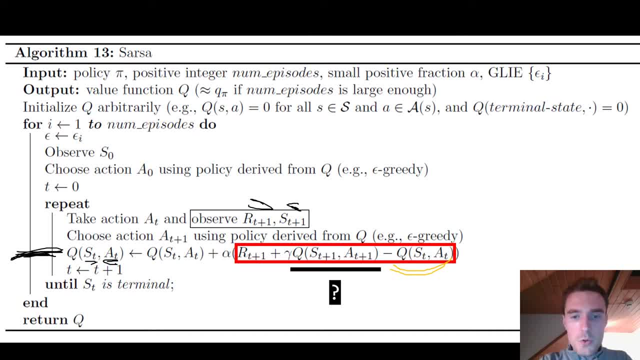 and the discounted q value associated to the next state action pair. the question that i ask you now is: what? what value can i use for this qs prime? a prime? this is the question. so let's consider our case, where we have our table or representation of the 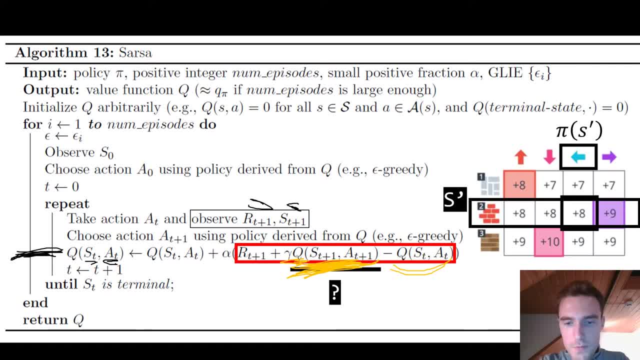 of the q value. i'm saying you, for instance: all right, the s prime is this one. so you know, this is s prime. this is your current t table. it might be the optimal one, but probably not. so you have four values because four actions. now the question is, which one do you? do you use one? 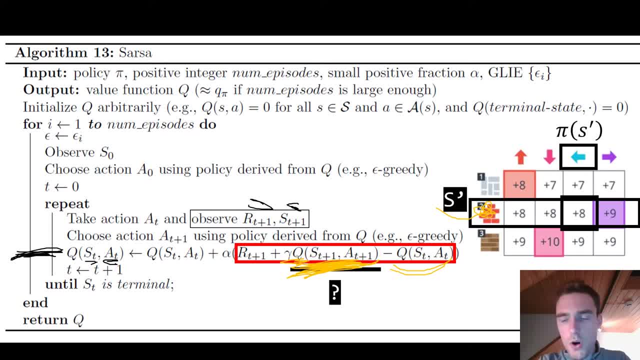 or the other. so the first possibility would be take the average of all the the four values. this will not be salsa. this will be expected salsa. this is one possibility. what you can do is take the max, in this case plus nine. this is not called salsa, this is called um sasa max, and sasa max is also. 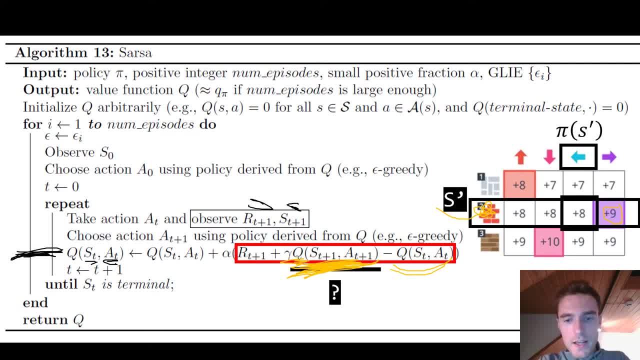 called q learning- quite popular name, q learning- and soooooo, let's first of all consider your actions and, for example, that's why i said you have a q value and S prime. i don't do all of what you can do because you only know how this 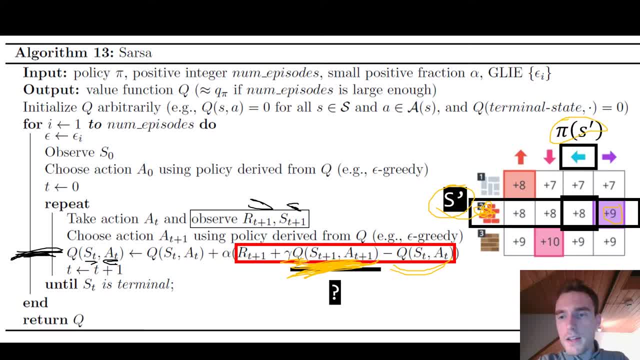 way it works, and so names and values are kept apart from the others. so you don't understand which ones are good for your policy, which ones are bad for your policy, which ones are good for your policy. and we can say all the times people are free, and so you realize the venoms and the 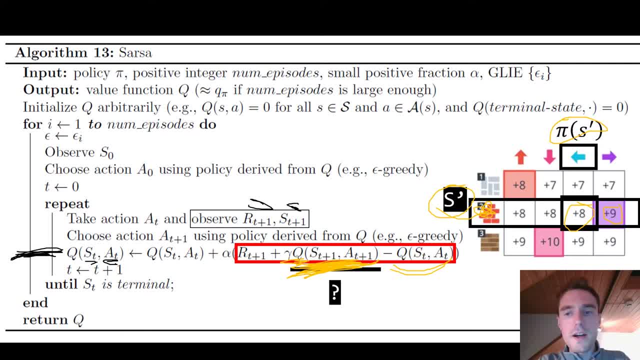 n expression variables are false in your know, all right. well, now you can get a few more for this. it to this. i read it in my table, it's plus eight and i use it to build my, my td, um, my td target, sorry, my td target. just to sum up, these methods of salsa, the different one which belong to a. 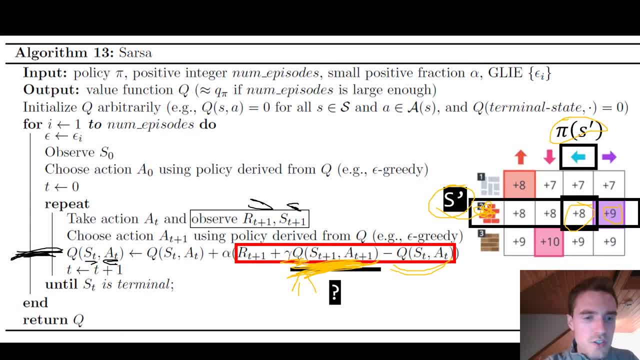 temporal difference. methods are really similar, they just differ. at this point where we want to estimate the target in order to compute the error, we saw that salsa actually reuse the policy, the current policy, the current epsilon greedy policy. this is called on policy learning, because you are reusing it to estimate your target. what you can do otherwise is: don't use the policy to make your 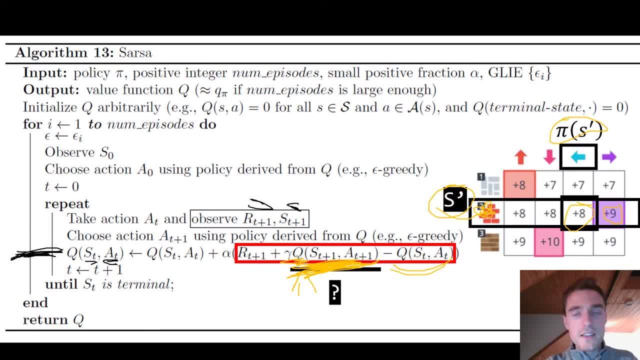 choice: either take the max or take the average. and in this case, it's not on policy, it's called off policy. you're not choosing the policy in order to, to estimate the q target. this is the difference, all right. and when you apply it, when you iterate, when for each? 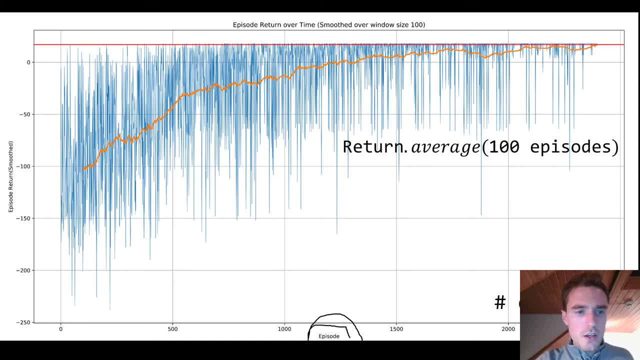 episode. so this is here the episode. you collect the rewards, it gives you the return and then you plot the return. this gives you the blue line and then you can smooth it by taking the average over 100 episodes and it shows you the yellow line and the algorithm updates the table so that it becomes: 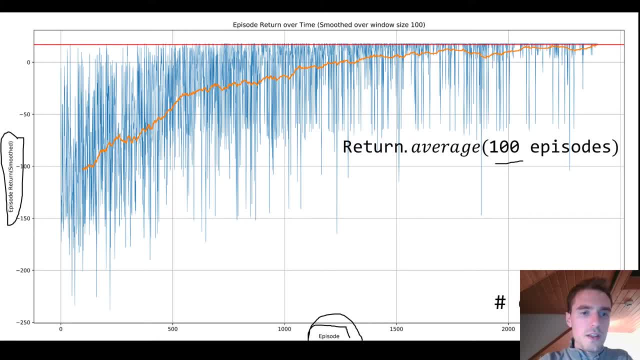 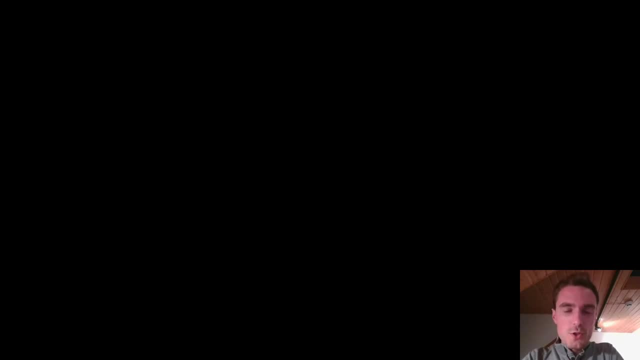 even better with respect to this goal of maximizing the expected return and at the end, we converge this to the maximum, to the optimal policy. just an example to show the learning process: so far, we have been using a table in order to store and update our q values. 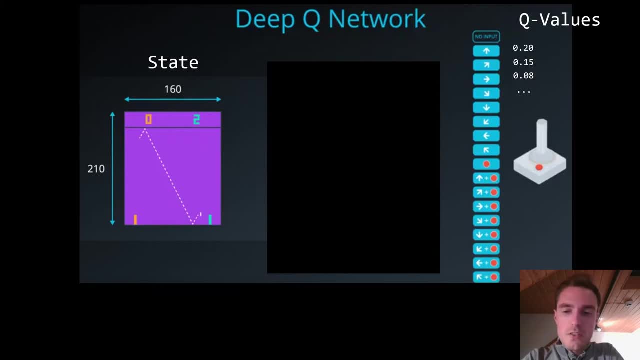 but in particular problems, it can't be the case because it's too computationally demanding. let's take an example here we have a problem where the state is composed of many, many pixels, and again we have a different actions that can be taken and applied to the 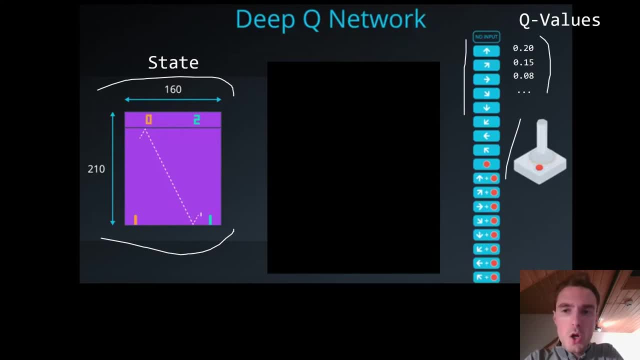 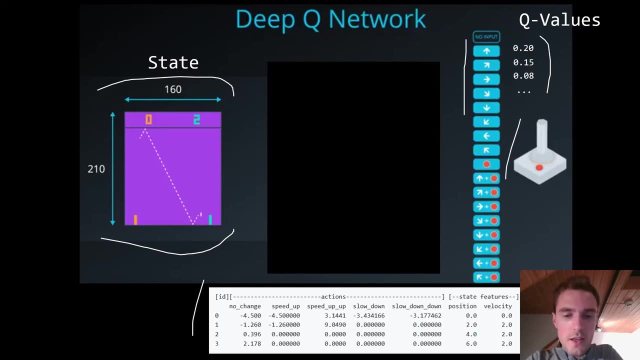 joystick and we want to estimate the values of each of these actions. so what we did so far is using a q table and for each state we have the different curve values. but this is not tractable, or this is not feasible when the state is too big, because the table will get too big. the solution for 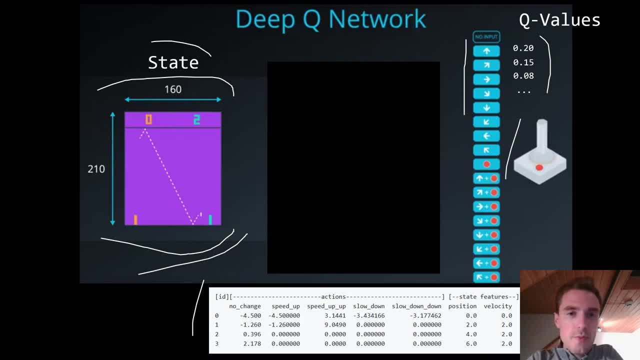 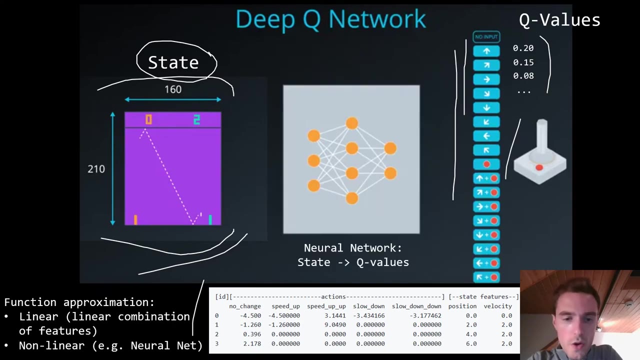 that is, to have a function approximator. so the function approximator will be given the state and will output: okay, how many action do we have? and so for each action we output one number, which is the q value. this is done, for instance, in deep q network, where you are using a net. 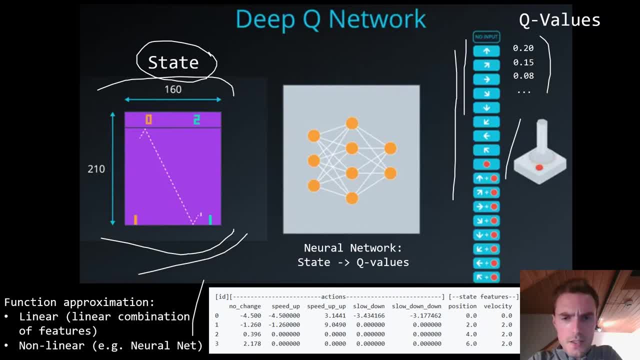 a network, a neural network as a function approximator. the idea is the following: here you put your state, so we have only three elements, but you will need one for each pixel at least plus the lgb channels. and here is the output. we have only two, but these are for the actions. 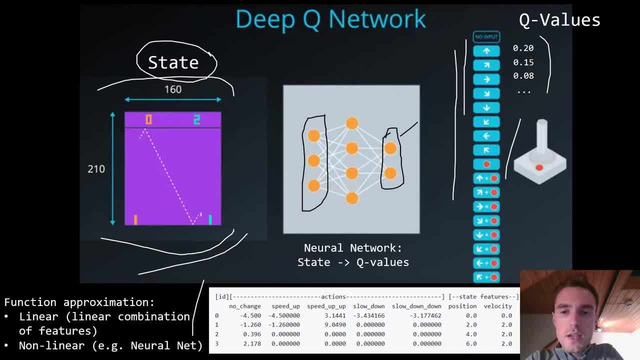 we need one per action, and then this value will be the value, the q value corresponding to the first action, and so on. and so the advantages. there are two main advantages. the first one is that now you can cope with really, really big states, which was not the case with the tabular. 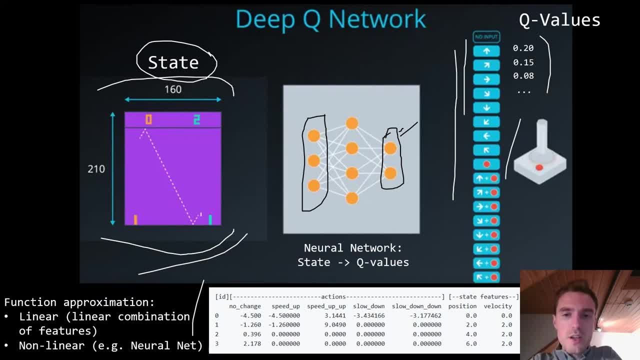 representation. and the second one is that, obviously, with the function approximator, you don't need to have seen the state in order to have a q value associated to that. this was not the case here, because we haven't met or because we haven't seen these states. we couldn't. 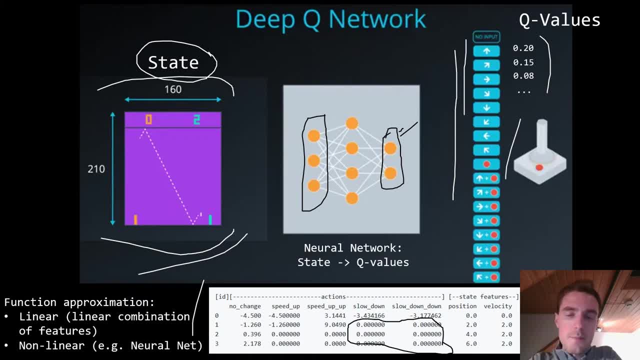 get or we couldn't estimate the value of them. this generalization property makes the, the value, the function estimator, really powerful and this is done, as mentioned, in deep q learning, with the q mentioning the, sorry, the deep q network, with the q mentioning the the q learning. so sasa max, we have just seen 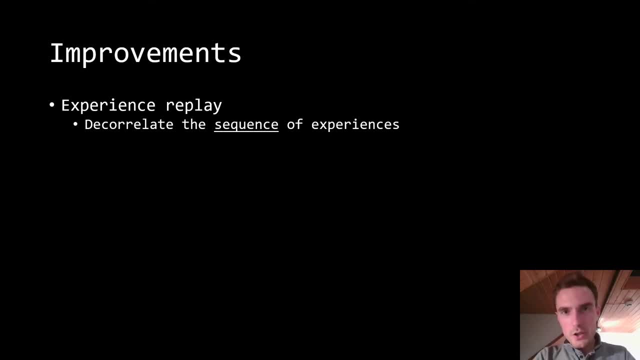 so using a function approximator instead of a q table is a good idea we have seen. nevertheless, for stability, we need to include additional improvements. so we mention five of them, and then i will cover only the first one, and the first one is about decoupling the time when 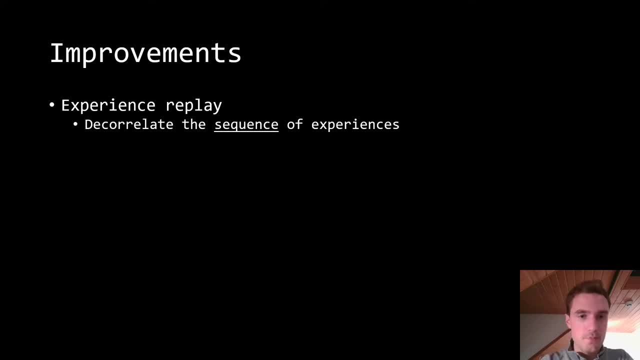 the time when you actually learn and update your model. it's because with an experience replay, we see that in a minute. the second idea is about fixed q targets. so you remember, we need two things to compute an error. the first one is the q estimate and the second one is the q target. 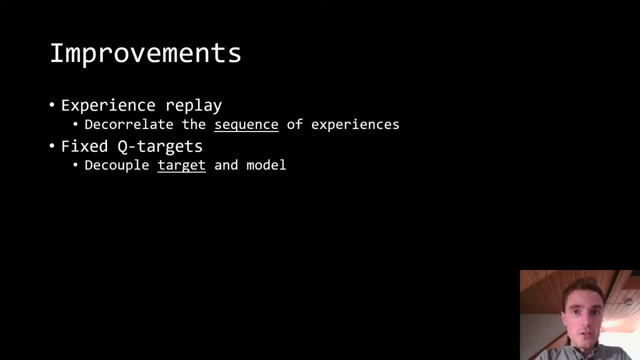 and both are read from the same model, from the same q table. and for stability, it is not good because you are updating something, you're updating your model, but at the same times, based on your model, so this has to be decoupled for stability. this is the idea of fixed q targets. 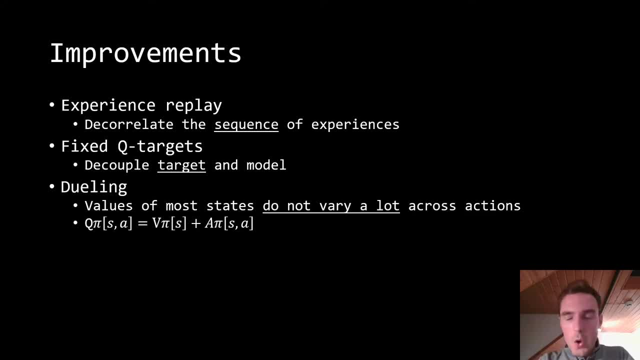 during. it says: well, you remember our table. we had some numbers in it, but do you remember the numbers? no, it's not important. what you remember is which of the four actions has the best or has the highest q value. in other words, you are not interesting in, not interested in, the absolute value. 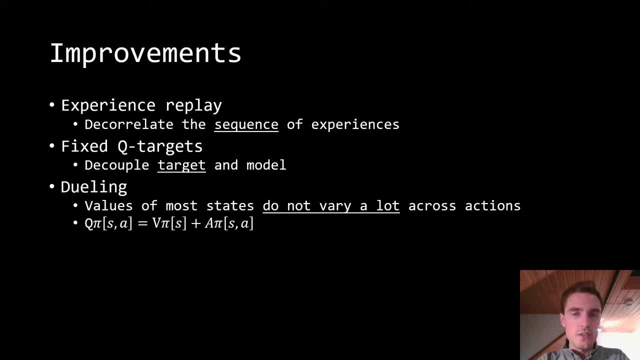 it's only about the relative. which one is the best compared to the one, no matter if it's 20 or 10, what is important is that it's bigger than the other one. so you decompose, your q value is one with, in one common term, shared by all the actions, and then the difference is made by 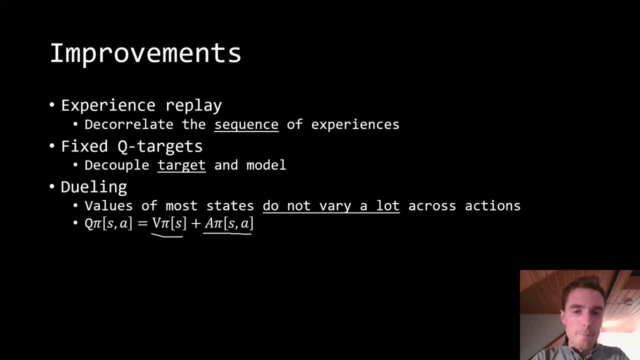 what is called the advantage term, that's the idea, splitting it to make it more stable. what is called the crazy part, the energy. so you have a critic which is value-based, you can think as a- i don't know- a supervisor or the parent, and you have an actor which is a student or the baby which is acting, and then 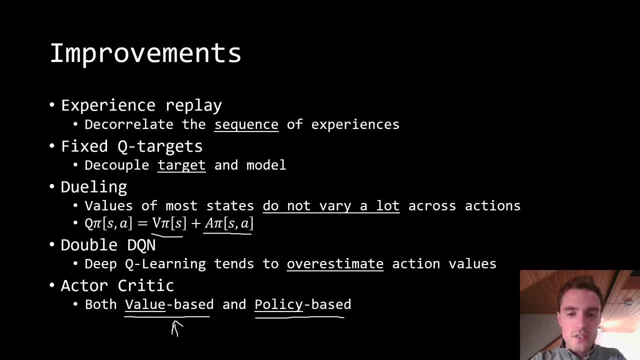 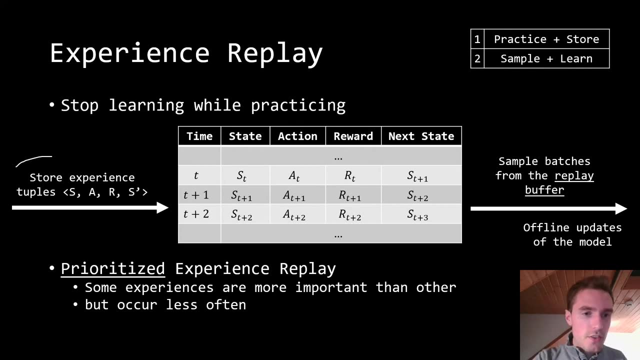 the assessment is done by the critic and the actions is done by the, by the actor. again, same idea. decouple things to make me to make things more stable. okay, experience replay: remember we are seeing these tables for each step and the question is: what do we do with that? we saw how to update our model with this, so maybe 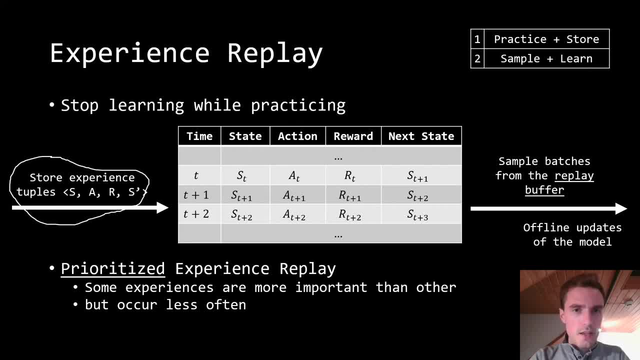 the. the other question is: how often do we update it? well, it has been seen that it's better to decouple, not to take immediately what we have seen and apply it to the model. just wait a little bit. so, for start, that's when we start to take time to try to handle it, and then we go with it. 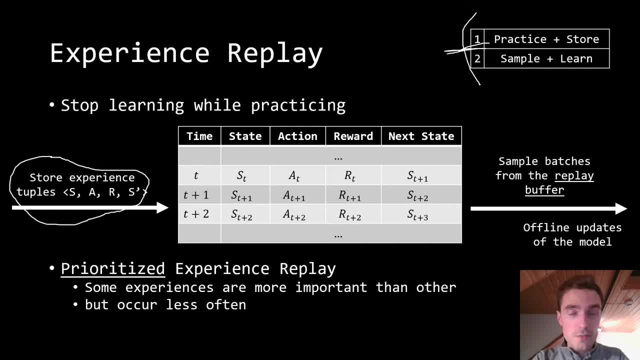 and then we start to think about it how it works. so we have this video course that i'll be River for you to learn about the ultimate five-step process. so i want you to take this as a starting point in this course. and then how it works is that you, you take practice, practice after practice. 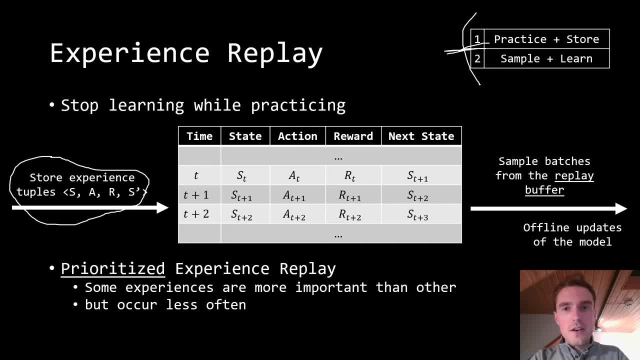 you play and you try, you experience, you collect your, your tuples of expense. and the second step went back home, or i don't know. but second step afterwards is learn what does sample mean? you have stored several tuples in a big memory place and now comes the time of sampling. so you are, yeah, randomly, for instance, getting samples. 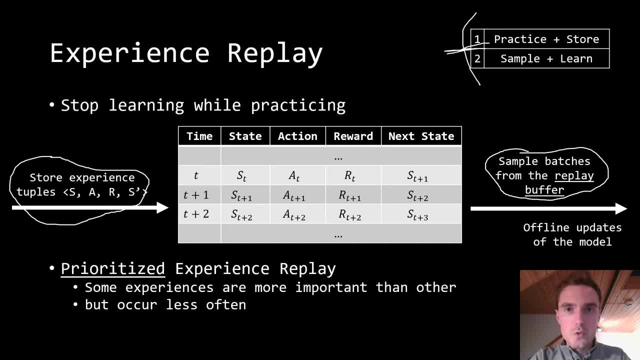 from it, which is called the replay buffer, and then you use it to update your model. this is the the idea of experience replay. if you want a more advanced version, there is this prioritized experience replay. what it says is: um yeah, some experiences are more important than others. 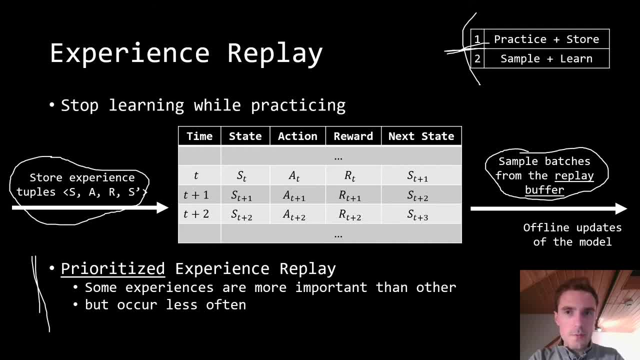 you remember when learning to, to ride a bike, a bicycle, you probably remember all of your fall or accidents where you did something wrong, and that shows that when acting, when learning something as a human, you put different importance um on some experience than the other. this is called prioritized. there is a metric you have to introduce to say this tuple was more. 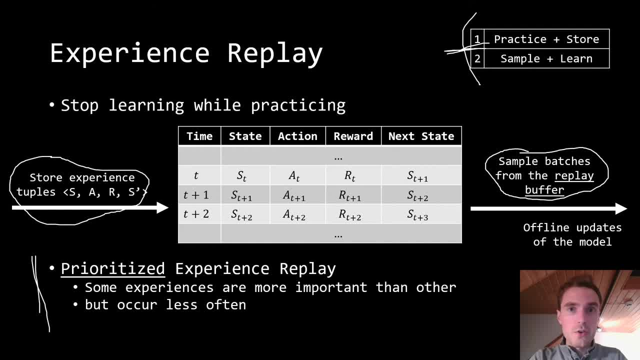 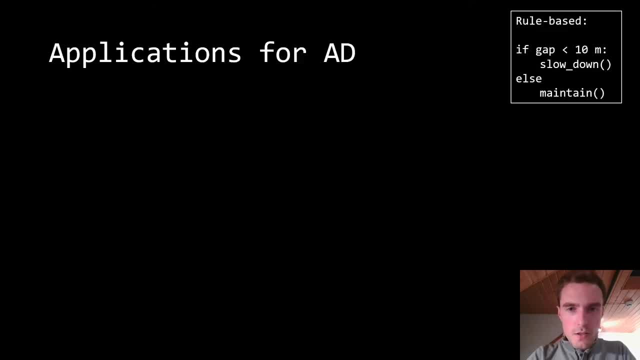 important in my, in my process, so it should be considered more often or more seriously prioritized experience replay. so we have covered the major concepts- very basic ones, but major ones- about reinforcement learning. i want now to take a couple of minutes speaking about the perspectives for rl, especially applied. 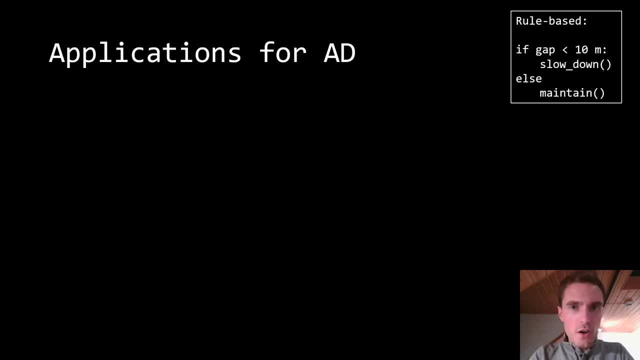 to autonomous driving. so to compare autonomous driving reinforcement learning approaches with let's introduce the rule-based methods. um a competitor to rl which says, for instance: this is a if else statement: if the gap with another vehicle is smaller than 10 meters, then slow down, otherwise maintain really basic, really simplification. but now we have something. 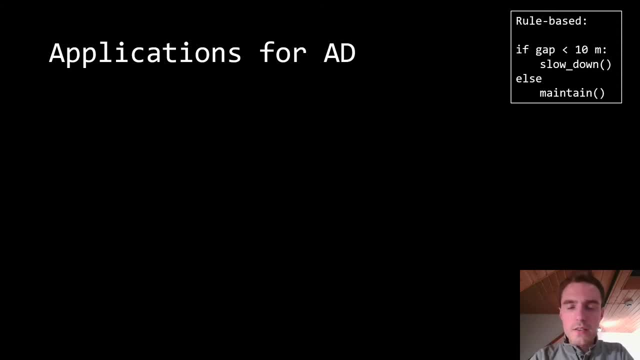 to compare with and using this comparison, we will set a couple of advantages. first, one is about the ability to use the linear approach to can do generalization really well. remember the what i said with the function approximator: when you can estimate a state without having explored it. 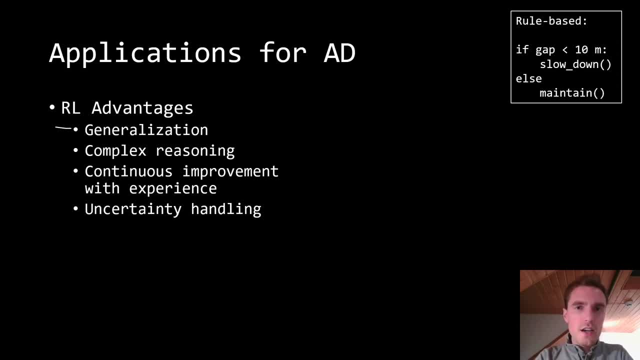 this is the same thing here: although you haven't seen a scenario, or although you haven't experienced or be confronted to a particular situation, you still can make a decision. so that's the one strength of reinforcement learning. um, in the same vein, you can address complex reasoning without having to design manually with an expert knowledge. 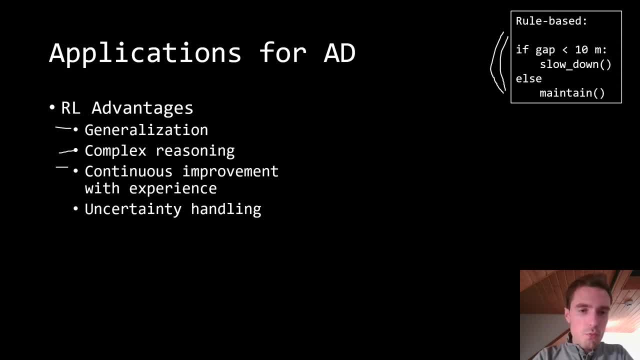 definition of all the rules. you can cope with continuous sorry. you can have the benefit of learning over time, and so you're improving your model over time. the better sorry the more data you have, the more data you are exposed to, the more experience you leave, the better your model get. 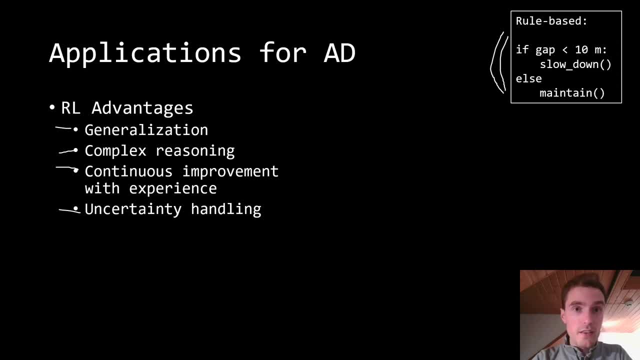 it. and, last but not least, you can. if you modify a little bit the formulation, for instance, having this partially observable mark of decision process, you can really well cope with uncertainty, which is a very important benefits when addressing autonomous driving situations. on the other hand, there are limitations, and especially when confronted to real-based methods. 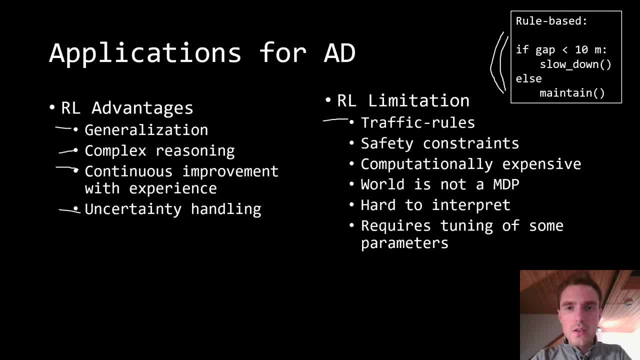 this is difficult to make sure that traffic rules are respected. but 100, sure, not one. 99.99, it's about 100 percent sure. this is not obvious. the same applies for 70 constraint. this is the strength, of course, of rule based. this is categorical. and another thing, not necessarily, but it can be more. 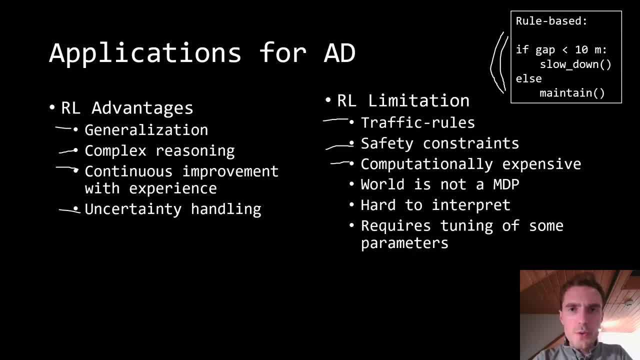 expensive from a computational point of view to use reinforcement learning approaches. you have to be very careful of the design. you have to use the design choice. you might have already guessed it, but the word of driving is not mdp. there are some tricks- stacking frames, for instance, or having a recurrent network- to cope with the idea that the future is not only dependent on the present, it's only, it's also depending on the past. so you have to adapt the formulation and 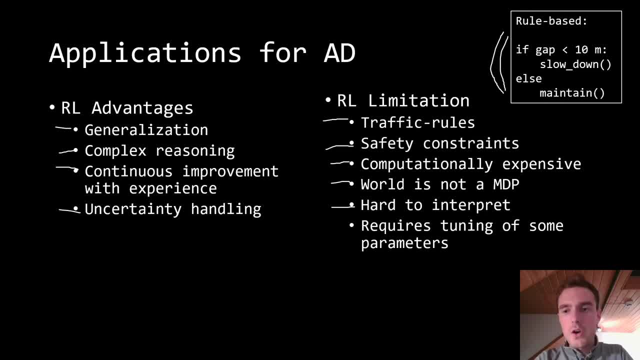 some, yeah, draw back. or at least one strength of the rule-based method is that is pure, is really interpretable. you just have to go to the different statement and see in which case you are. makes it easy to debug. and yeah, rl as a machine learning tool requires some hyper parameter tuning model. 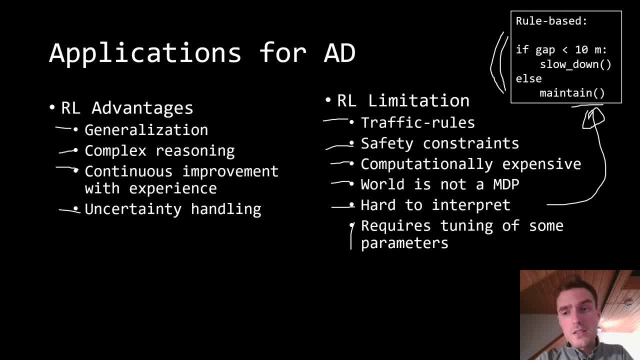 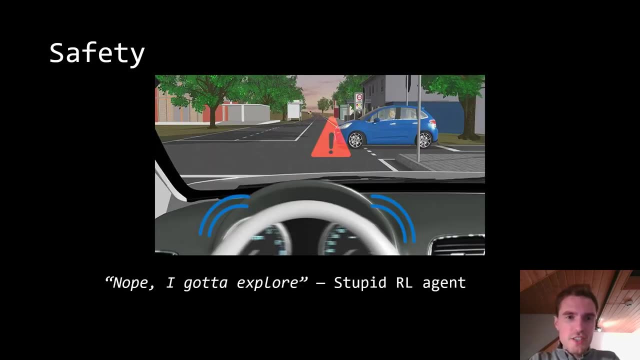 tuning, which is not required for that. so strengths, limitations. what i want to say with that is that both make sense and the best idea would be not to have it alone but to make a fusion of them and merging. the two approaches make sense, especially for for safety. 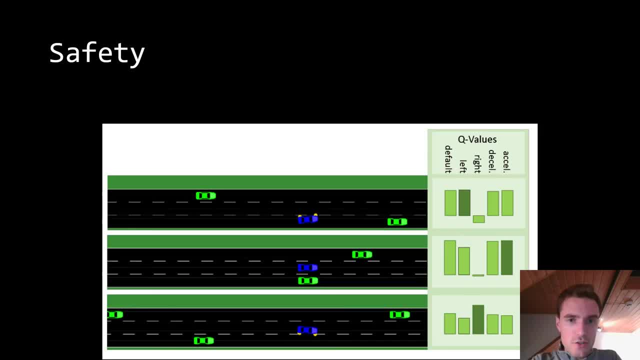 so for safety, what you can do is called action masking. remember this scenario where we are driving on the highway and for us it's obvious in this particular scenario, there is no point taking the action. go to the right, it will just take a few seconds for the road and there is the chance of you taking a few seconds off the road. 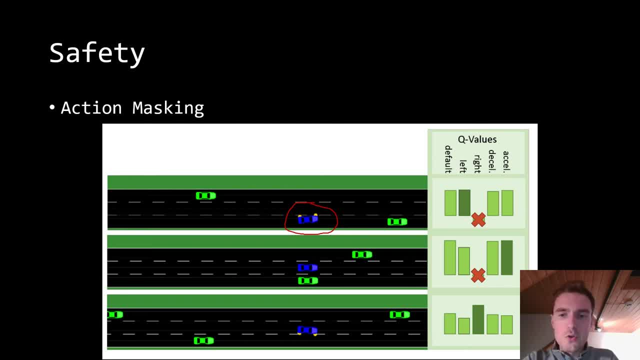 so why not saying, in this particular case, i forbid you no need to explore, no need to contemplate. you only have four actions. and this could be done for um safety purpose, where we know here is the same case, there is no point going to the right um. it shouldn't be too much effort to code that. 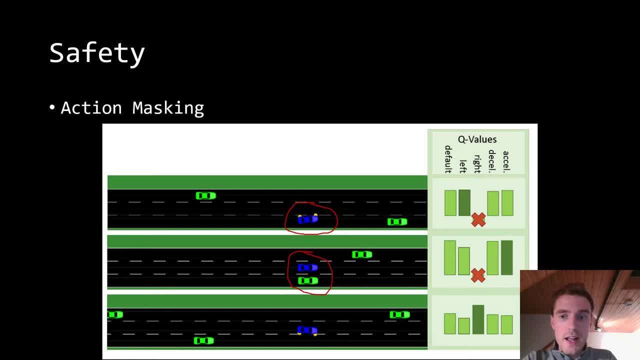 uh, he shouldn't cover all the possible situations, but just strict rules, and there shouldn't be any where you can then make sure reinforcement learning won't even consider this option. There are different benefits of that. The first one is that it reduces exploration. You don't spend time having a look. okay, what does happen when I'm doing that? 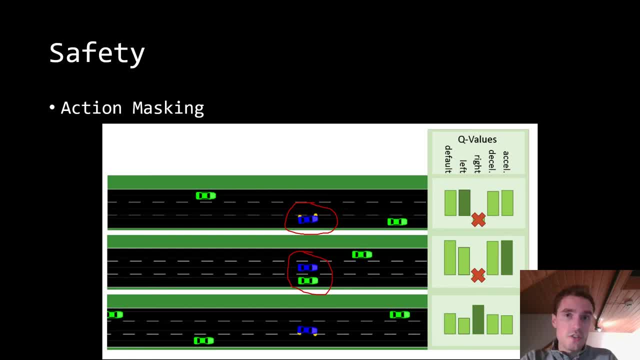 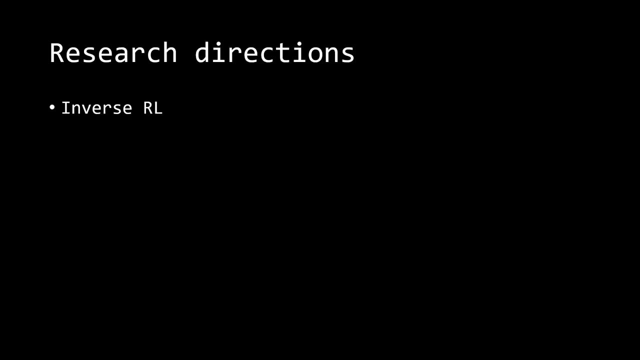 Maybe most important. more importantly, it's about safety. It just increases safety, robustness and interpretability. Action masking an example of merging, rule-based and reinforcement learning for autonomous driving. Let's mention a couple of research directions that are currently taken for autonomous driving. 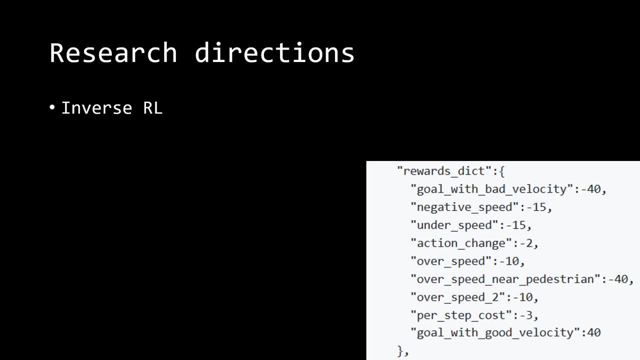 You remember my configuration here of the reward structure In particular. yeah, the cost for each step was set to minus three. You could ask why not minus two, why not minus four? You will be right. The idea of inverse RL is okay. this step of designing it is quite a hard task. 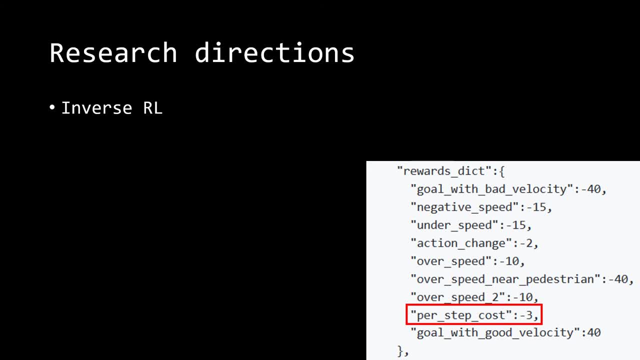 What if, instead, we try to learn this? Learn means, in this case, we observe a good driver and we assume that his behavior is actually related to a reward function that is hidden. This is the hidden state, And we want to get access, to have an estimate of this latent. 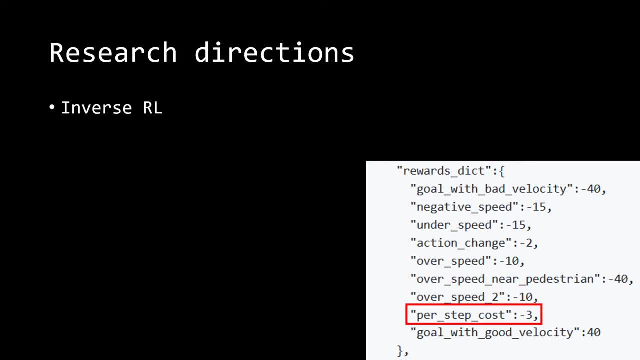 variable. This is the idea of inverse reinforcement learning. Learn the reward function. There is what is called hierarchical reinforcement learning. The idea is again to decouple, to make it simpler. by decoupling You decouple the low level decision, For instance, all what is related to speed control. got it a bit faster, got it a bit. 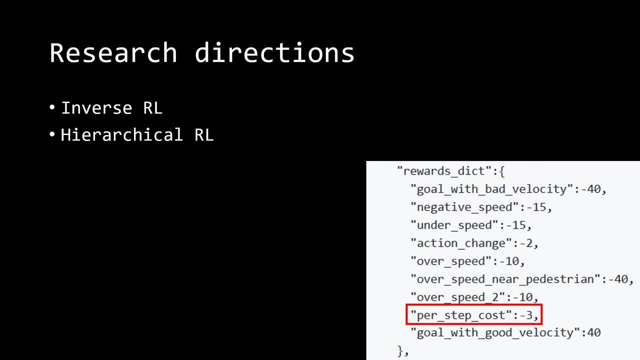 slower and so on, From the high level abstraction of decision. ie yeah, overtaking someone. this is a higher semantic decision multi-agent. we have already mentioned it, but if you have the opportunity to communicate with other cars, with other participants, with the infrastructure, then you could together. 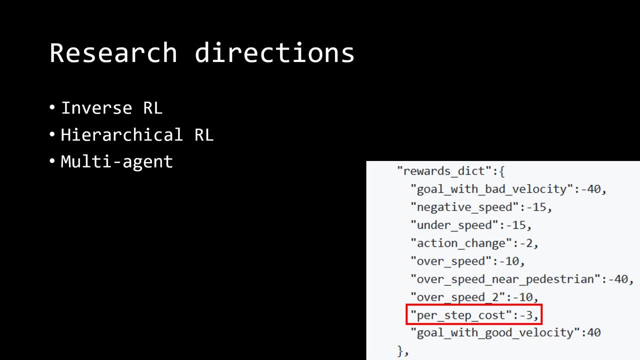 plan a better strategy. for instance, if you know if you are crossing and then you know that it will be going straight, then you will stop. but if he is saying, okay, i'm turning, then they will be free. this is just an example. it requires vehicle to vehicle communication. 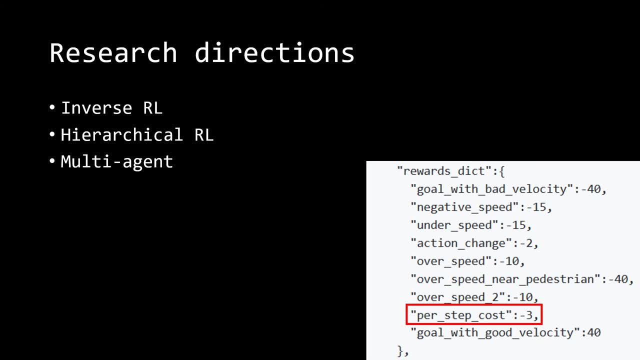 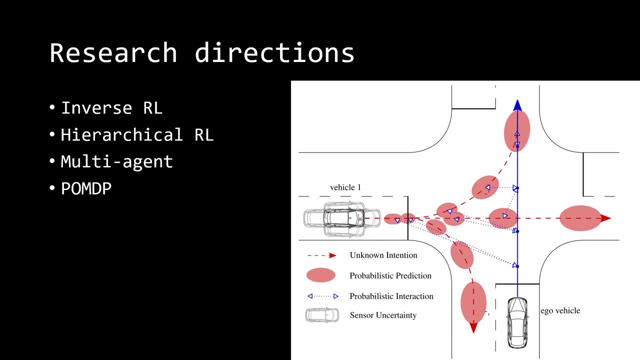 but, assuming you have it, this is a good opportunity to apply reinforcement learning. the pomdp means partially observable markov decision process. this is the case. this is actually the case for every driving situation. the sensors gives you only approximated values about the, the state of the other participants, for instance the position you 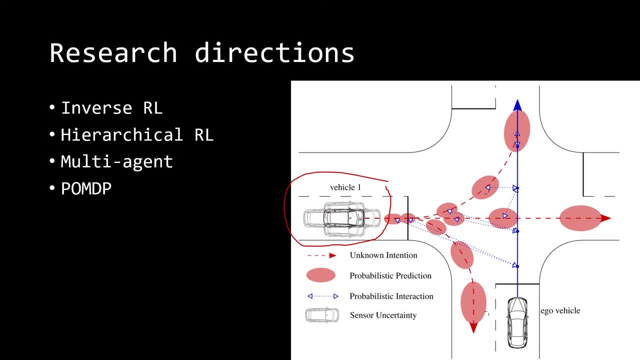 are not sure if it's exactly here or here. as a result, it's difficult to make decision if you are not sure, and this is just about the uncertainty in measurement. this is not mentioning the fact that there are some occlusion with occlusion. you have no idea if someone is coming and with all this uncertainty. 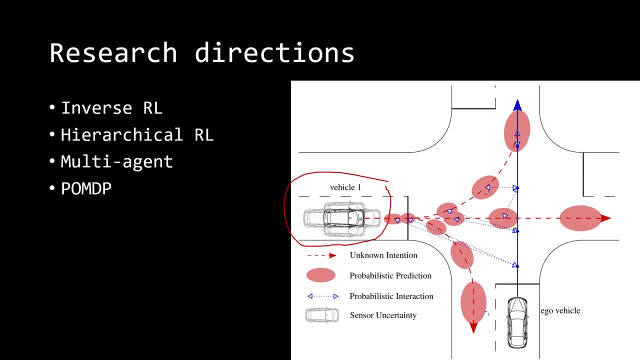 it's really difficult to make prediction, it's really difficult to make decisions. so what you do is you formulate it as a partial observable mdp, where you try to track, to update beliefs about the state. you can't access to them, but you try to to track them and make decision based on that. 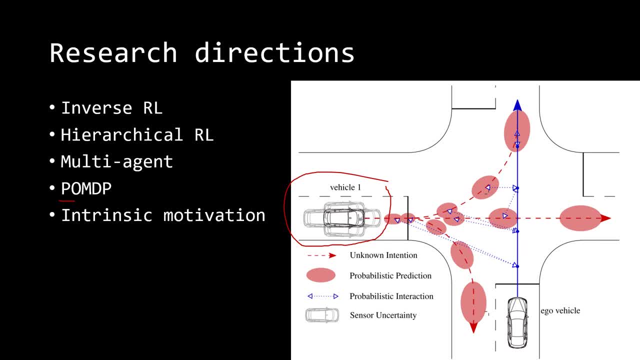 yeah, so that's the one for the very first of my presentation. for that right, kindly. so i have one more question for jim, and it's a real deal, as the guy just said. so this question is usually asked by the имеет. the problem is it's a knowledge. 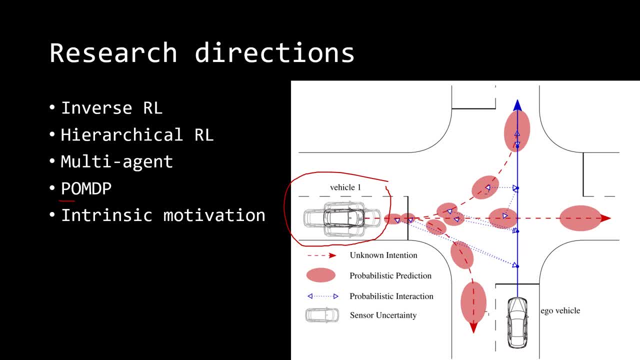 field with a lot of different observations. typically for my area, research, i was saying that in academic as well as in the engineering, we are able to know the answer and what is the answer to this question. so this is just a real topic. so obviously this is not. 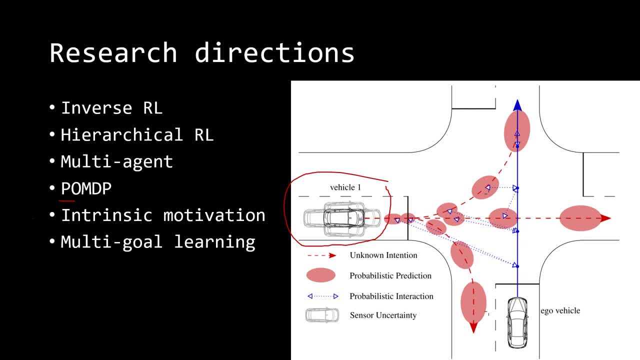 And last one was about multi-goal learning. You still keep your five actions, for instance. You still keep one set of action. You have still one state, But what you do is you are defining several goals and you will get, as a result, several Q tables. 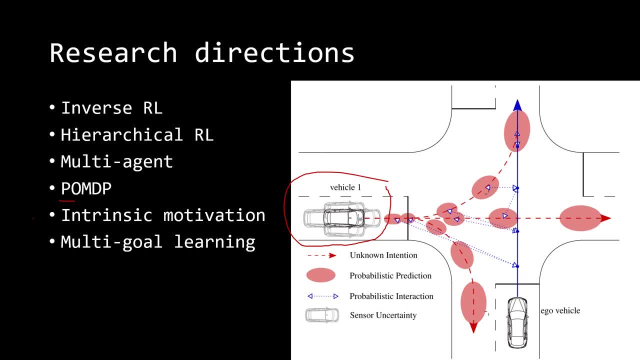 For instance, one goal would be: OK, I have to drive and learn to cross an intersection properly. The other one would be the policy that says you are to avoid going too fast close to pedestrians. Now you have two policies. They both take the same state. 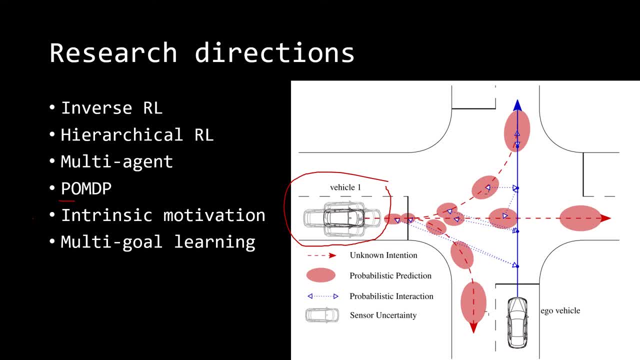 They both propose you an action And of course it's a question: How do you select if they are not agree on what doing? This is, of course, the question of multi-goal learning, But the idea is again: decompose, decompose. make sub-problems from this problem. 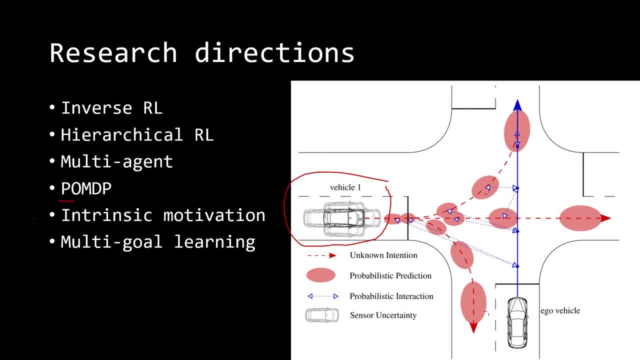 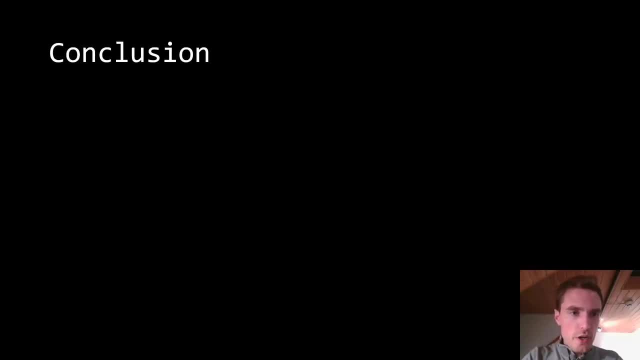 Decompose, To make it simpler. So that's the research direction to keep in mind. This brings us to the conclusion. So what we are seeing today is the different concepts of reinforcement learning, In particular the intuition. that is closed. We can draw a parallel with the human behaviour. 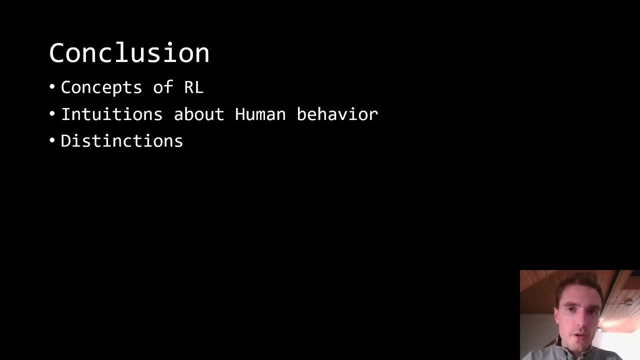 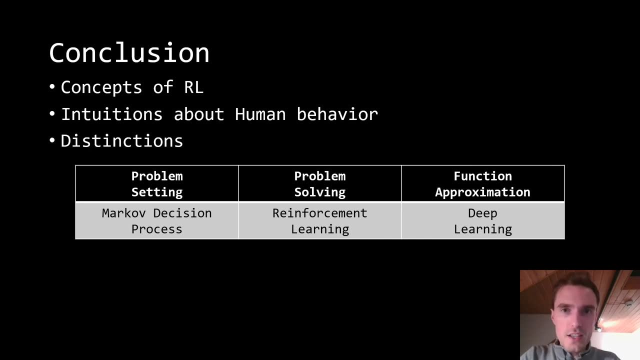 Not to forget the distinction, the several distinction we saw. In particular, remember that the MDP is used to formulate the problem, That reinforcement learning is about solving it, trying to find the optimal policy. And if you heard about deep learning in the context of RL, it's really about having a function approximator instead of a tabular representation. 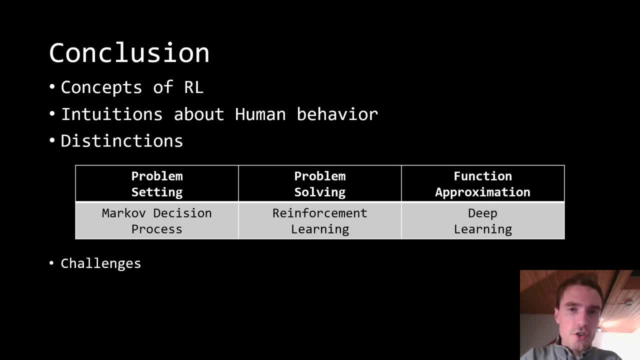 Maybe the challenge is to mention the state representation. We have seen that if the state is big, this is not so easy to address. Also, the delay rewards. We have mentioned it for Go where it's quite far away the point where you get a single reward. 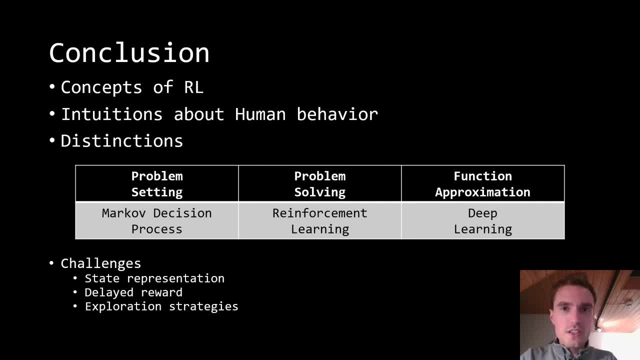 So that's a problem. Exploration strategies: It's not so obvious how to organise it so that you see everything, but at the time not spend too much time on it. Fine tuning: It's a machine learning approach. So parameters In particular- I mentioned the epsilon decay has to be tuned.